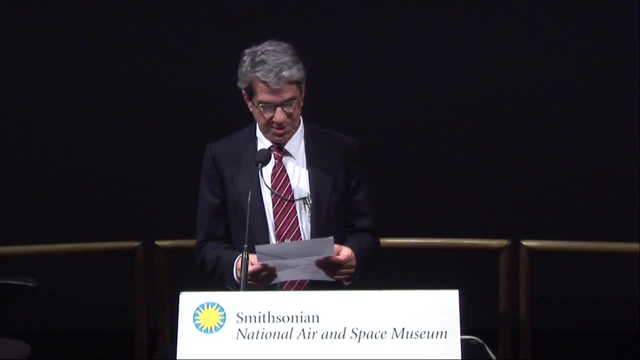 Alumni, Centennial Professor of Physics and Astronomy at Johns Hopkins University and the Principal Investigator of NASA's WMAP. He received his Bachelor's Degree in Physics and Astronomy from the University of Maryland and a PhD in Physics from the Massachusetts Institute of Technology. He then worked at the Goddard Space Flight Center, rising in. 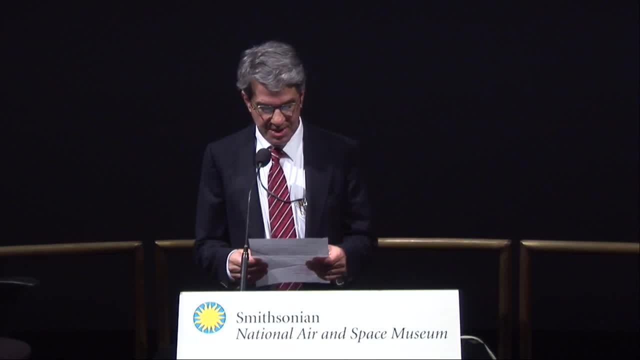 2005 to become a Senior Scientist for Experimental Cosmology, a Goddard Senior Fellow and a Branch Head for the Infrared Astrophysics Branch. He's won numerous prizes and awards, including the coveted Henry Draper Medal of the National Academy of Sciences and sharing 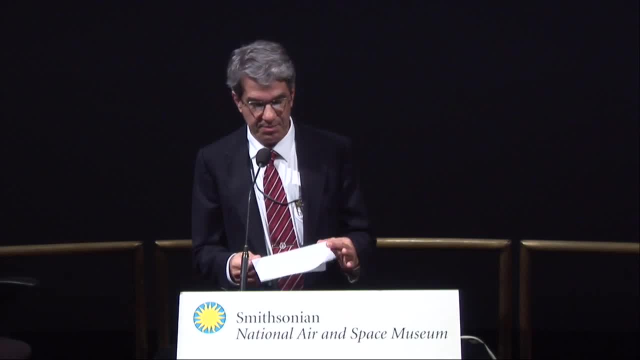 the 2010 Shaw Prize in Astronomy. Now, for those of you who came early and viewed the documentary this evening about James Van Allen and his Iowa team, you will appreciate how far the Explorer series has come in the past 50 years, and we are especially pleased tonight to have someone in the audience who 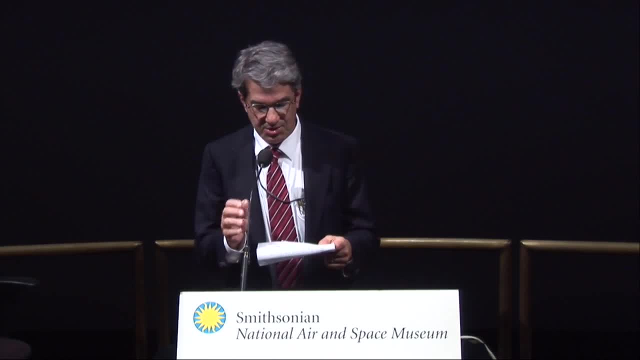 lived with the Explorers longer than almost anyone. George Lilley, who is the Director of the Explorers, was one of James Van Allen's graduate students in 1957-1958 when he helped build the payloads of the very first Explorers. 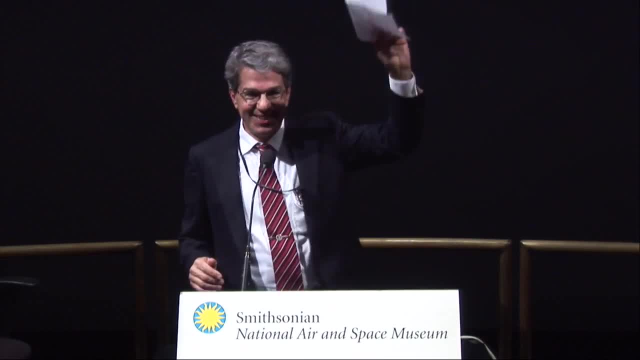 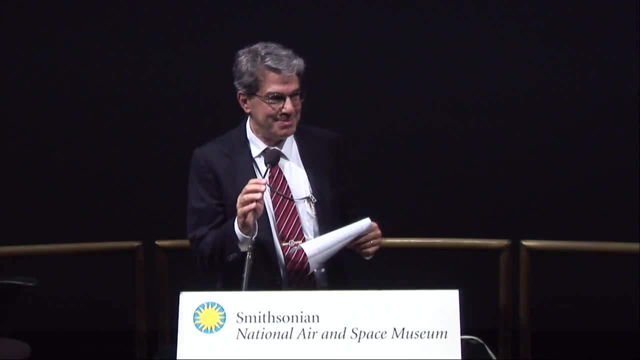 There you go. Hey, Great to have you, What an honor to have you here. It's just kind of for me as a curator here at the museum, it's kind of like if you were an art historian and you say: oh, there's Leonardo da Vinci in the audience, How you doing? Whoa, Anyway. 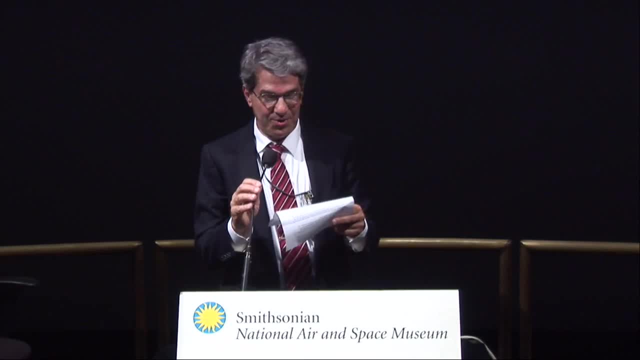 so well Also. finally, I want to thank our wonderful sponsors, As they have for the past nine years. the Science Mission Directorate of NASA continues to be a great friend supporting this 2012 season. Tonight, NASA is represented by David Schuman, Executive Officer for the Science. 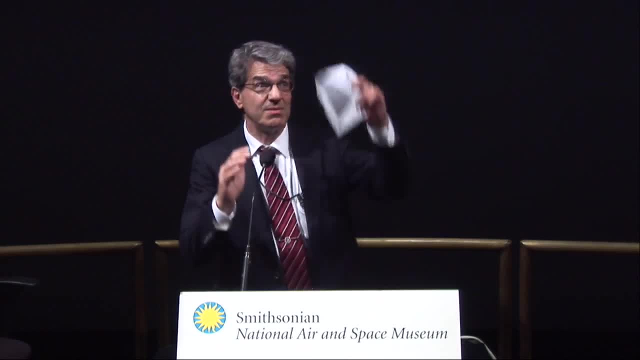 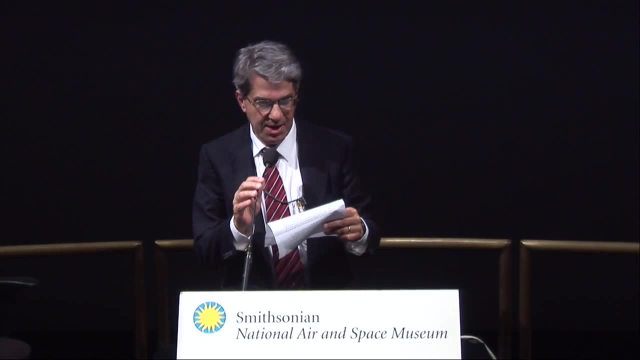 Missions Directorate's Associate Administrator, Dr Schuman. stand up There. you go Right there, Okay, Thank you very much, And we also welcome Michael O'Hara of the Aerojet Corporation, which is co-sponsoring the 2012 NASA Explorers. 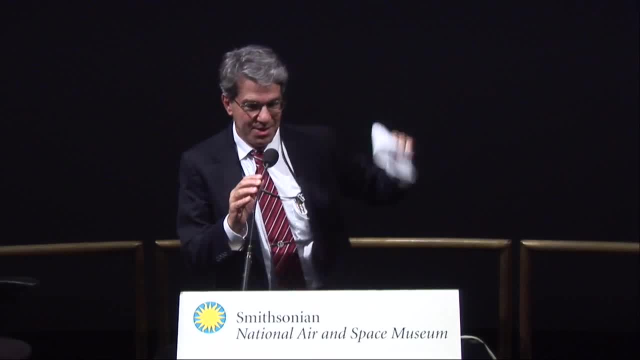 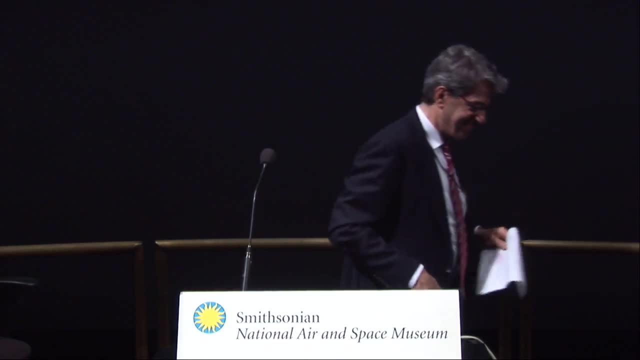 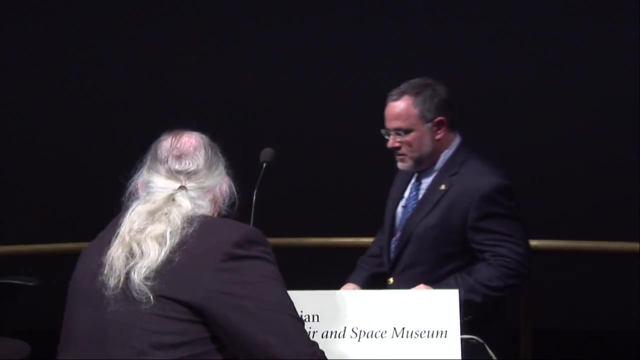 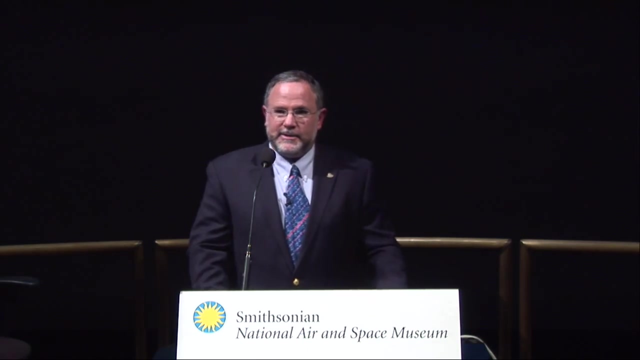 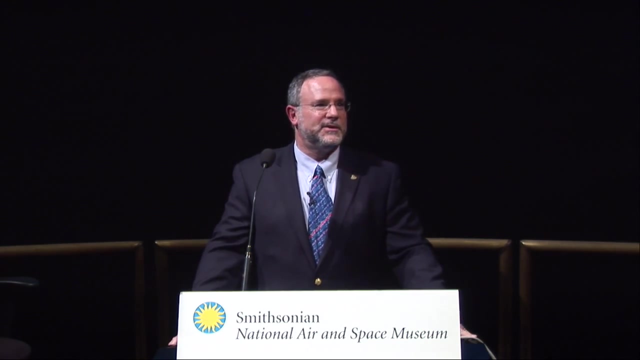 Thank you very, very much, So I will now turn over the podium to Dr Bennett. Well, it's always great to be at the National Air and Space Museum, one of the truly great museums of the world, So I love this place and I'm very pleased to be here to talk. 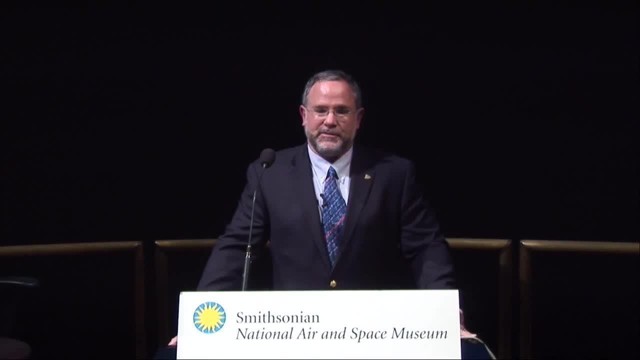 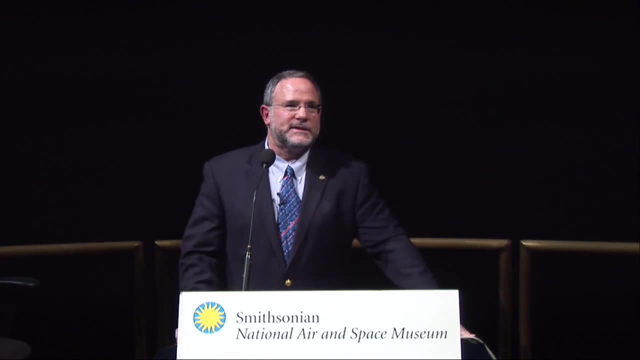 about the cosmology from WMAP, which I entitled Big Bang for the Buck, And I'd like to focus the discussion this evening on a question that's very important to me and very fundamental, which can simply be asked is: how did our universe come about? 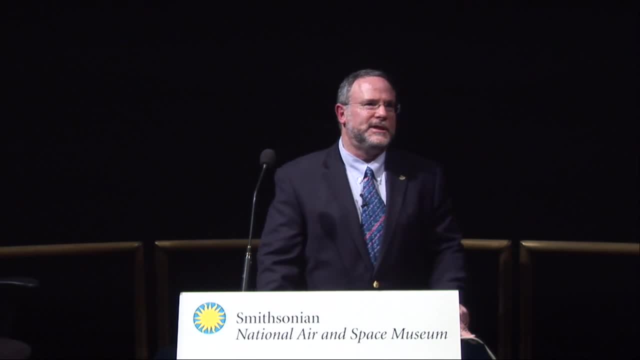 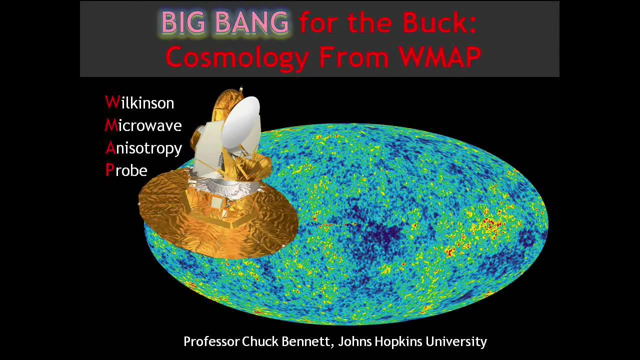 Okay, Okay, It would be completely reasonable to say that there would be no way for us to know. After all, we are human beings trapped on or near this tiny speck of dust in the universe called the Earth, And the universe is vast and enormous, so it's far from obvious that this is a question that we can answer. 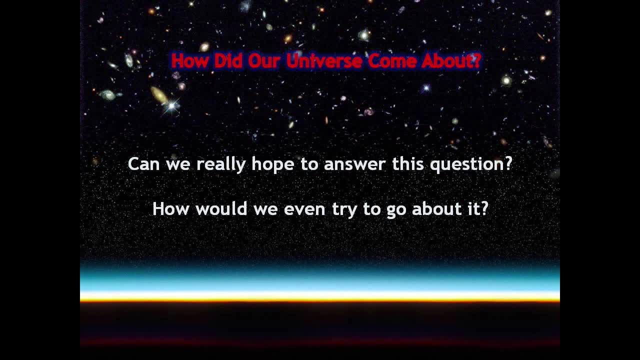 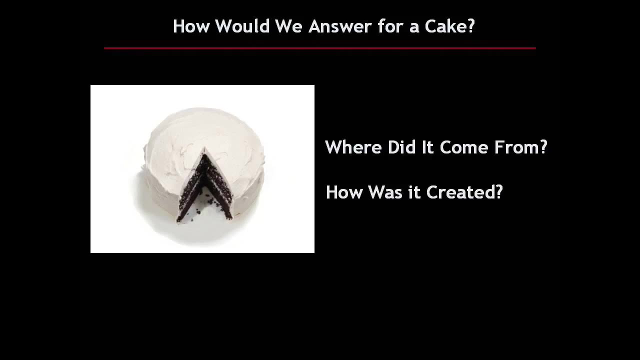 But so there's also the question: can we hope to answer the question And if so, how do we go about it? So I'd like to begin with an analogy and ask maybe a simpler question. Suppose we had a cake and we said: how did this come about? 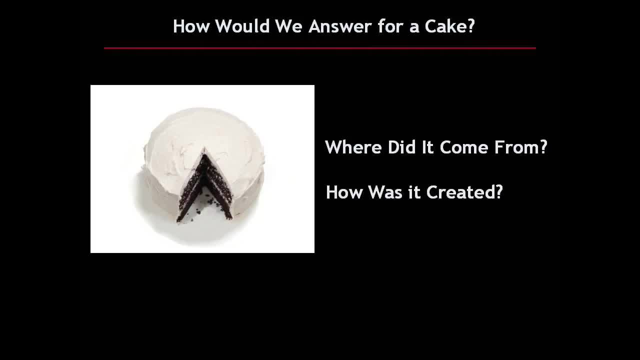 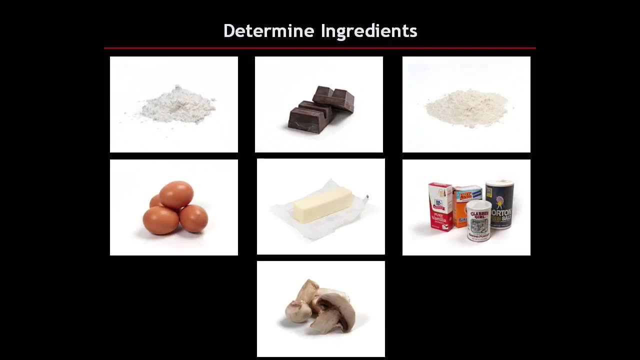 How did this cake get here? How was it created? How would we go about doing that? So what you might want to do is do a chemical analysis or some other way to get the ingredients. There might be flour and eggs and chocolate, butter, sugar, other ingredients. 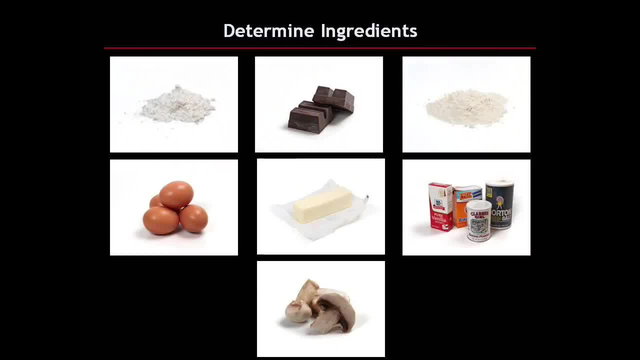 That you might expect to have in a cake. And if you did an analysis you might also find ingredients you didn't expect to find in a cake. So you should always be ready for surprises. You even better than the ingredients would be to find a picture of the cake being made. 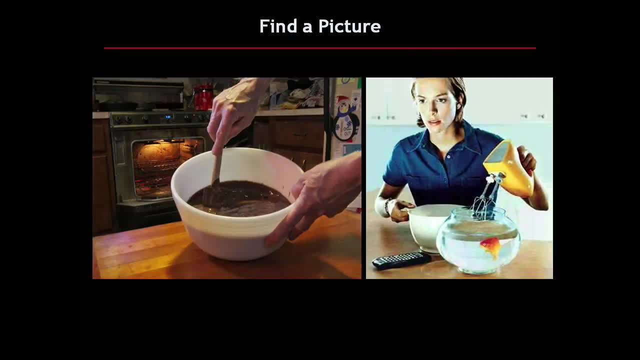 Then you would sort of see the ingredients and the process of the cake being made. You might see the chocolate being stirred And, once again, you might want to be ready for surprises. That's a good idea, That maybe things didn't happen exactly the way you thought they did. 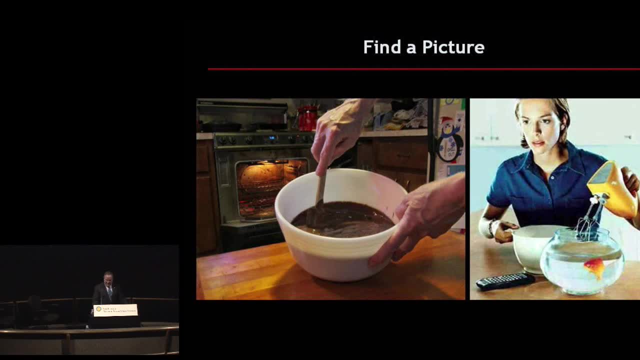 So to understand the creation of the universe, we need a picture, And to get a picture we need a time machine. We need to go back in time to see how the universe was put together And, according to this movie, having a time machine will help us do this. 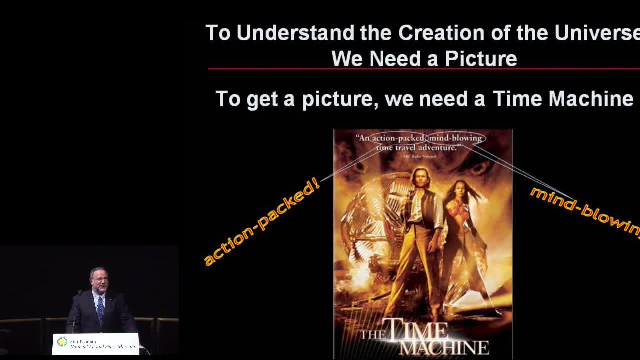 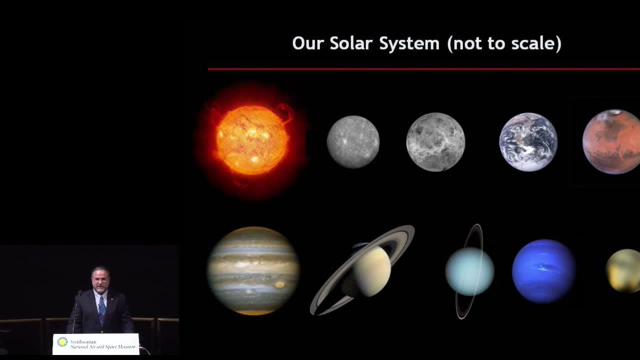 in a way that's action-packed and mind-blowing, And so that's what I promised for this evening. So, if we look out in nearby space, what do we see? We see our sun and we see the planets, And I guess I have to be careful, because Pluto, which I have here, is not a planet. 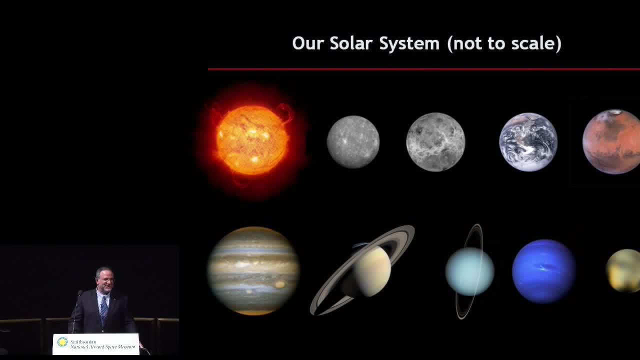 So that's got to go away. It was a planet when I went to school, but it's not anymore And the distance is a little bit too far. It's a little bit too far, So the distance to these planets is quite large. 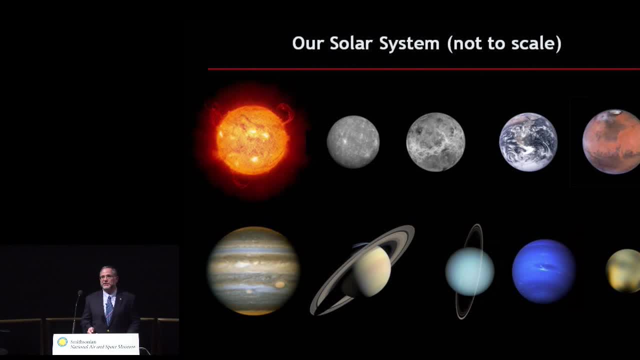 As you know, if we send spaceships through the solar system, which we do, it takes a long time for them to get where they're going. So the solar system is quite large. However, our Milky Way galaxy is quite a bit larger than our solar system. 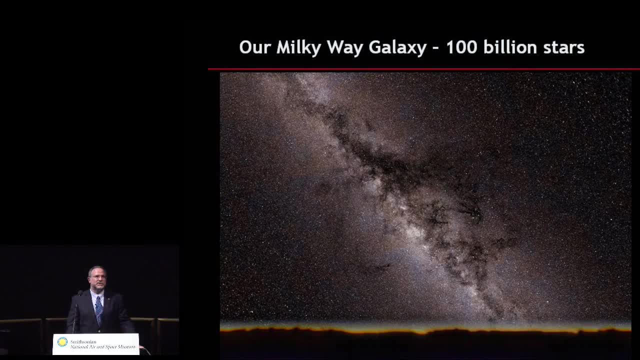 Our Milky Way galaxy contains 100 billion stars and is shaped like a pancake. Okay, So we live in this pancake-shaped thing And if you go out to where the sky is dark, you'll see why they call it the Milky Way. 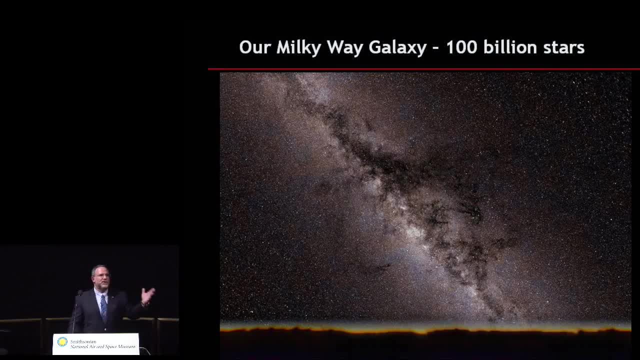 because you see this band of light across the sky. That's the cumulative emission from all of these stars. The dark areas that you see here are a result of particles- dust, blocking our view of the stars, And if you want to actually see better through the dust, then it helps to observe in the infrared. 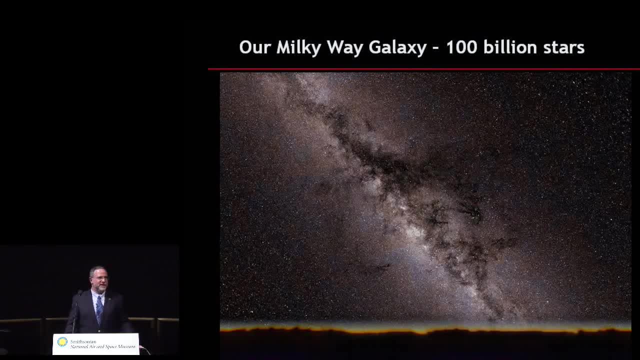 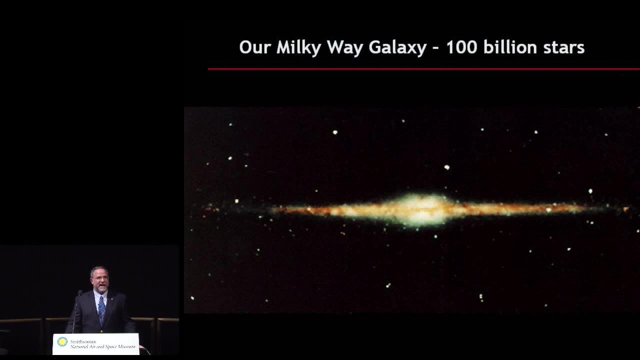 So here's a picture from an experiment, Here's a picture from an explorer mission, the COBE, which looked towards the center of our galaxy in the infrared, And you can see again here the kind of pancake nature of our galaxy that we live in. 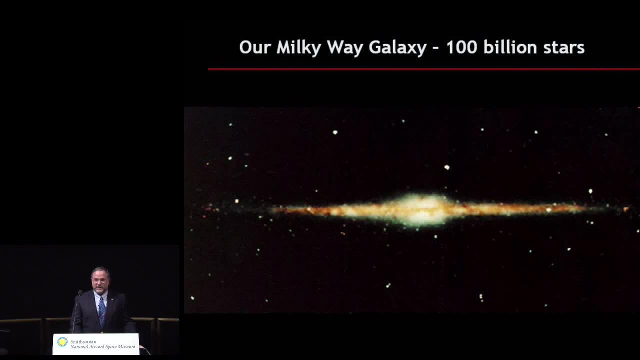 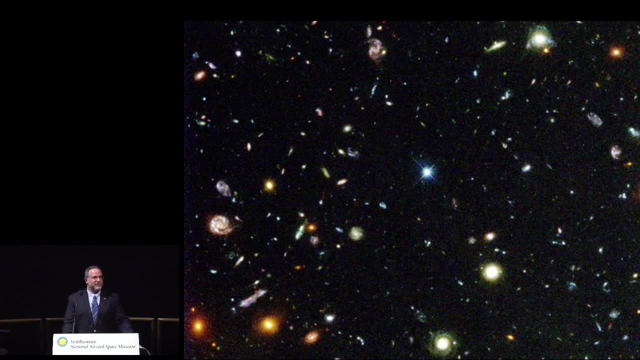 Well, I said that there were 100 billion stars in our galaxy, but there are also something like 100 billion galaxies in our visible universe, And this picture is from the Hubble Space Telescope And virtually, I think, everything that you see there is a galaxy. 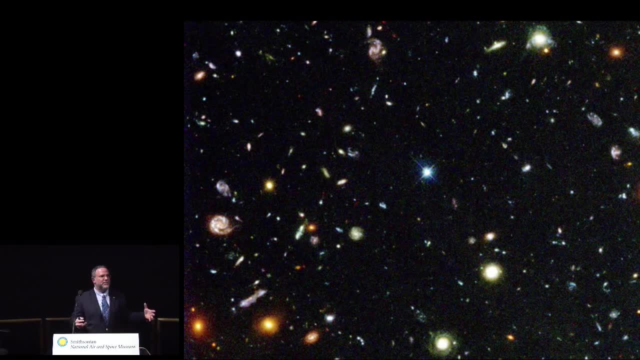 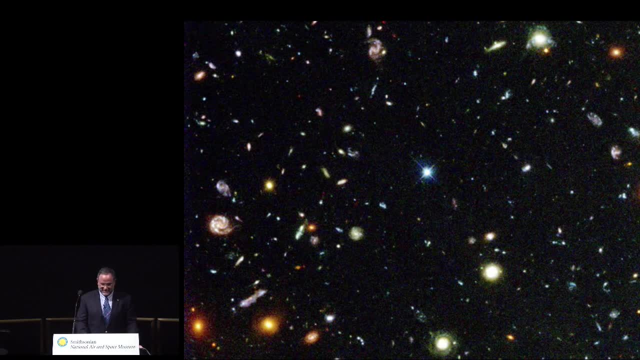 Well, I'm running out of words, but it's an unbelievably vast amount of space, And the thing about all the light that we see is that it has to obey the speed limit, which is 671 million miles per hour. That's quite fast: 186 miles per second, or one foot. 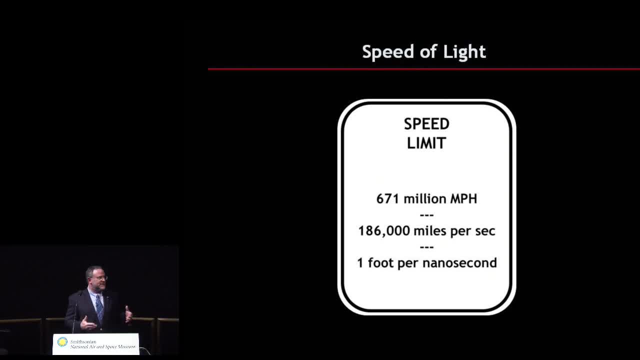 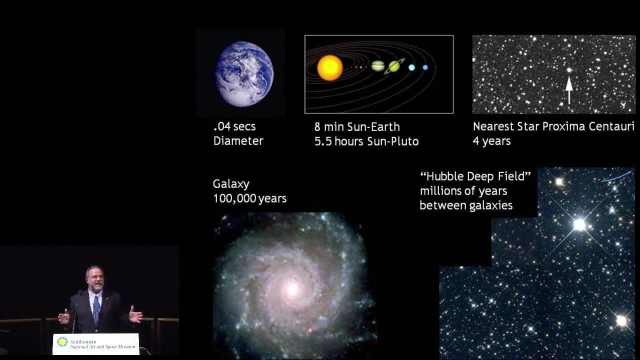 You know, the number of feet we're on is about 1 in 4.. It's about 1 in 6 foot in a nanosecond. So this is really fast. This is why, when you turn on a light switch in your bedroom, it seems like the light comes on immediately. 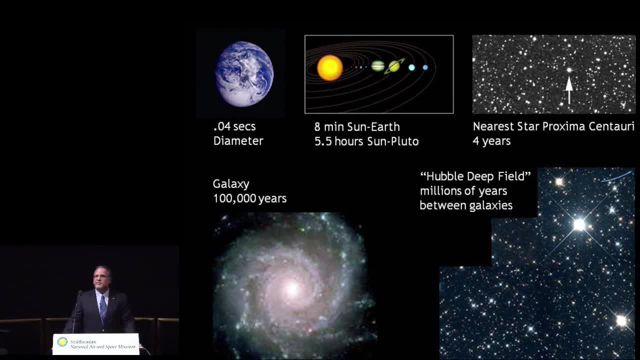 You don't notice the time delay because the light gets to you extremely quickly, But when you're looking in space it's not. this fast speed is made up for by the large distances, So it takes light actually .04 seconds to go the distance of the diameter of the Earth. 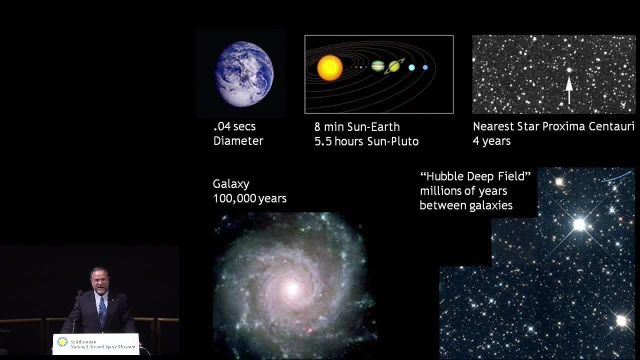 It takes eight minutes for the light from the sun to reach the Earth- Sun to get to us here on Earth- and 5.5 hours for it to get to Pluto. So you get the sense that here you've got this enormously fast speed of light, but you also have enormous distances. What this? 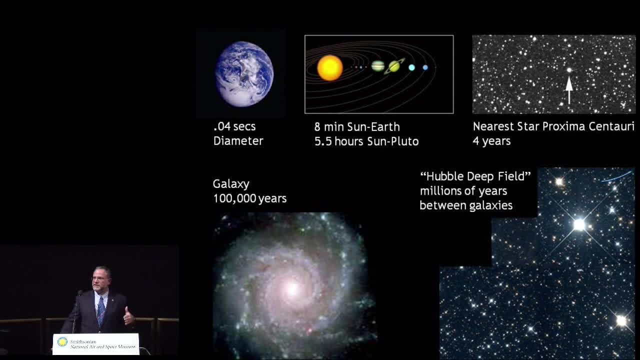 means is that when we look at the Sun, we are not seeing the Sun as it is the moment we look at it. We are seeing the Sun as it was eight minutes ago. The light that gets to us takes time. Now you get a sense of the time machine that we're going to be working on here. We are seeing the past when we 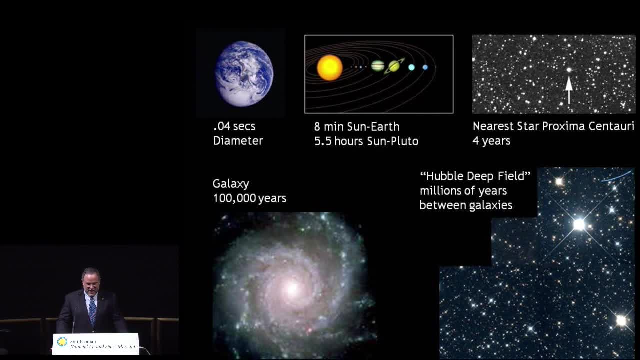 look at the Sun, We're seeing the past of eight minutes ago. The closest star to us besides our Sun is Proxima Centauri and it takes four years for the light from that star to get to us. So we see that star as it looked four years ago. If the star were to blow up or disappear or fizzle out. 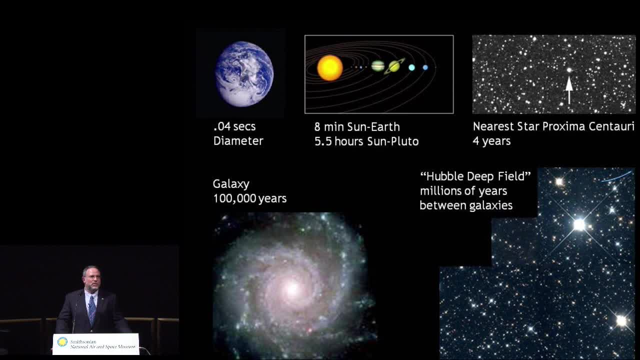 we wouldn't know it for four years. We are looking at it as it was Our galaxy. The galaxy takes light. 100,000 years to go across the galaxy, even at that enormous speed. That's how huge the Milky Way galaxy is. And yet the Milky Way galaxy itself is tiny in the scale of 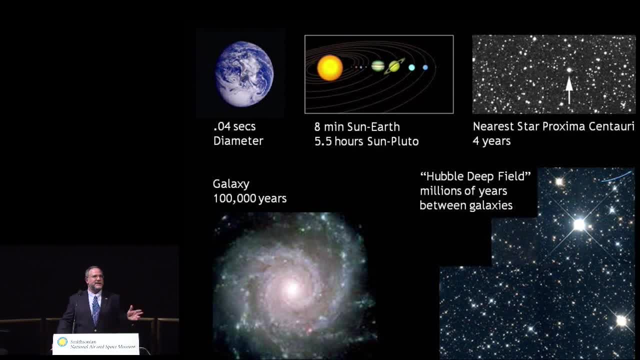 the universe. It takes millions of years for light to get between galaxies, typically, So the universe is enormous and it takes light time to travel, And this provides us with our time machine. And the nice thing about this time machine is we don't have to read the instruction manual. 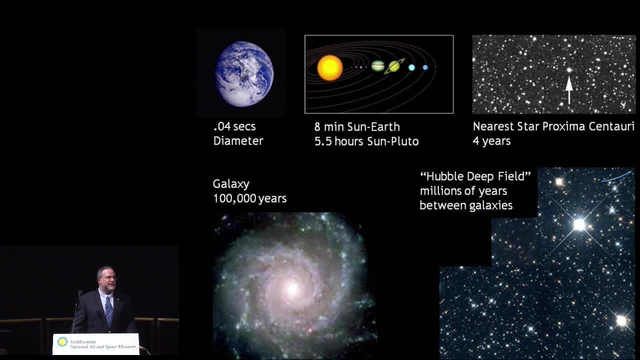 The data on it is small and we can look up instinctively. So when we have good data we layer our knowledge and take actions to study than do random science, sitting on it on a bench and trying more science And increasingly it comes from the universe. We actually can't. avoid it because we can get sort of the past or figure out how it's operate. Because we can't avoid it. The light that comes to us takes time to get to us. There is nothing we can do about it. We can't avoid it, But we can take advantage of it by allowing that to give us a way. 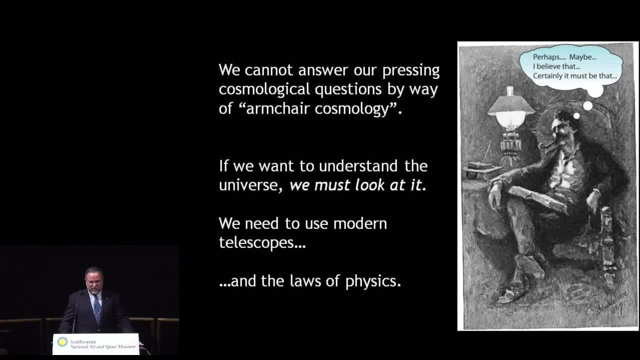 to look into the past, So to answer our pressing questions about cosmology, about the science of the universe as a whole. we cannot do it by sitting in an armchair and thinking great thoughts or reasoning about what it must be like – because it's impossible to think otherwise. It's impossible to 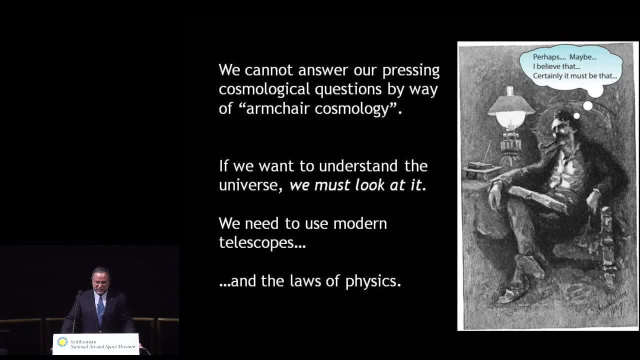 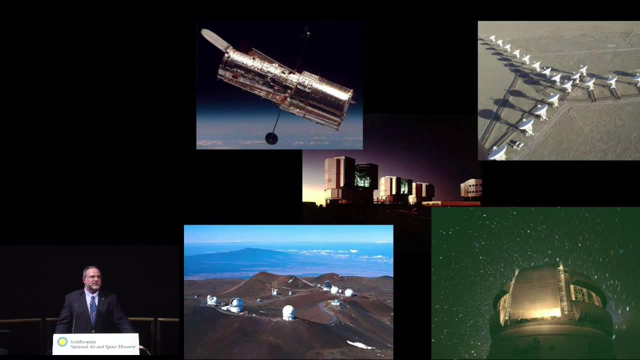 because it's impossible to actually know. in truth, what we have to do to understand the universe is to look at it and to make measurements of it, and to do this we need modern telescopes and we need to understand what we see in terms of the laws of physics. so we have an armada of telescopes in space and on the 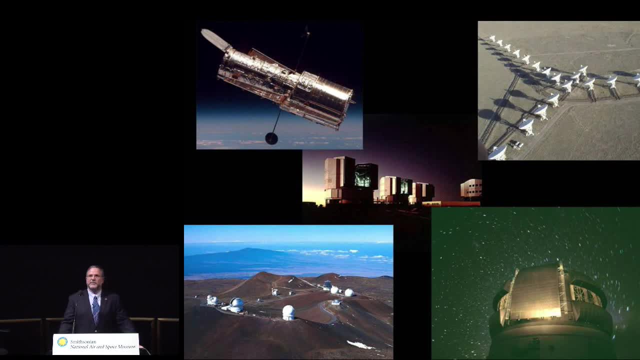 ground and at all kinds of different wavelengths, from gamma rays and x-rays, visible light, microwaves, radio waves, all designed to do different things, you know, specifically designed for the purpose that of the kind of science that they should do. but we have all kinds of eyes on the sky and then when we have 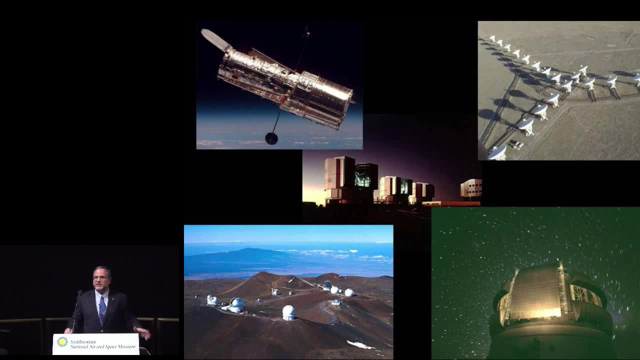 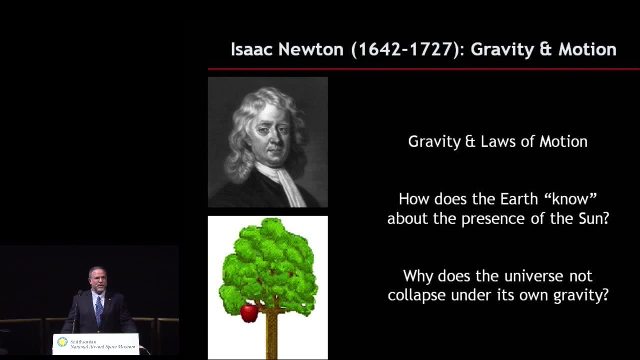 the results. we have to understand them and for cosmology, for the universe of whole, it turns out, the important thing to understand is mostly is gravity. gravity is the weakest of the forces in physics, but on the scale of the universe it is the most important. Isaac Newton, who was a truly brilliant 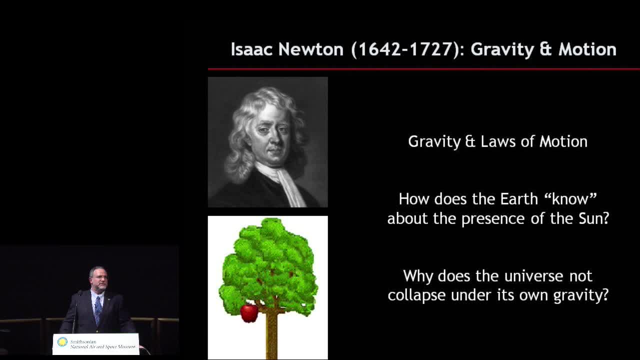 guy came up with laws of gravity, so called Newton's laws, and, for example, you can use Newton's laws to calculate how the earth goes around the Sun. however, Newton was so brilliant that he not only wrote down what he understood, but he also wrote down what he didn't understand, and he he said that he can. 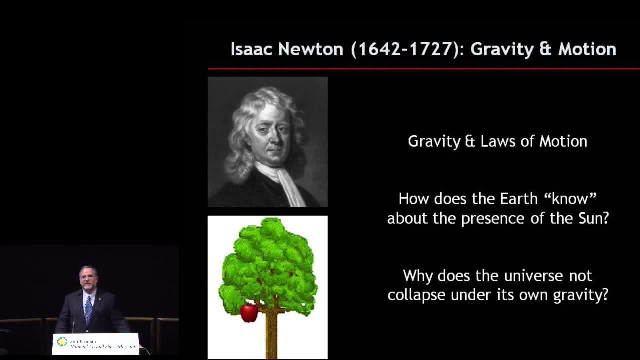 calculate the orbit of the earth around the Sun. but he doesn't understand how the earth knows the Sun is there. I mean, the earth would normally just go straight if it was going in a line. that's one of Newton's laws. a body in motion keeps going, so why did why it turns? because the Sun is there. he has 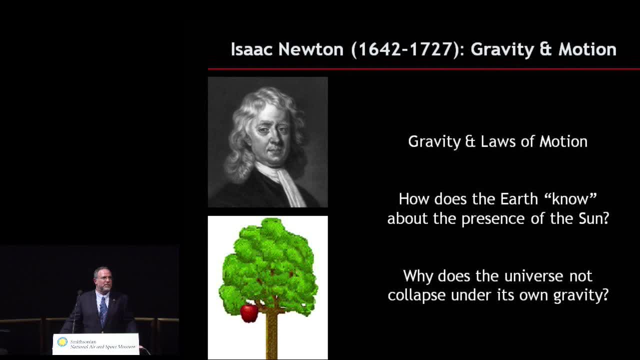 that in his equation, but how does it know? there's no rope, no smoke signals, no semaphores. how does it know to turn? another thing he didn't understand was you look up in the sky and you see all these luminous bodies across the heaven and 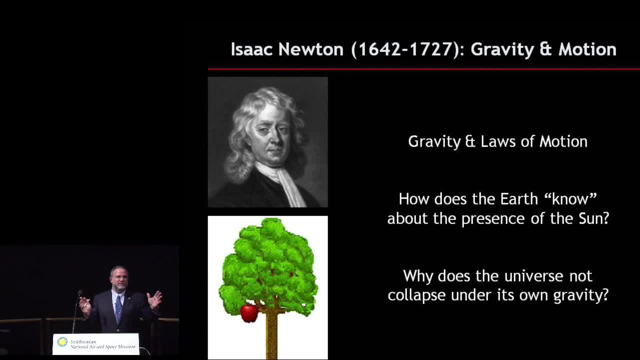 he didn't understand why gravity didn't make it all combine and collapse together. why is it all still spread out? and so, for these questions, he wrote down that he frames no hypotheses. he, in other words, I don't have a clue, but it was the brilliance of him to actually write down what it is that he, that he didn't. 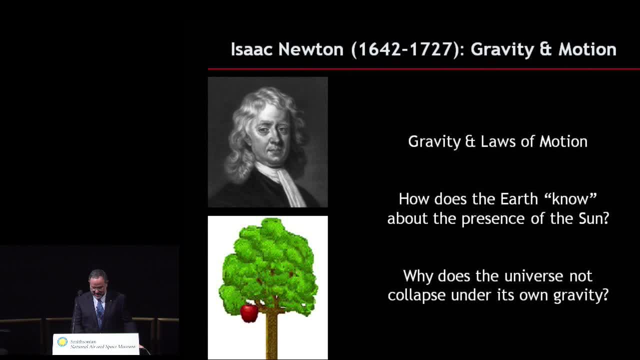 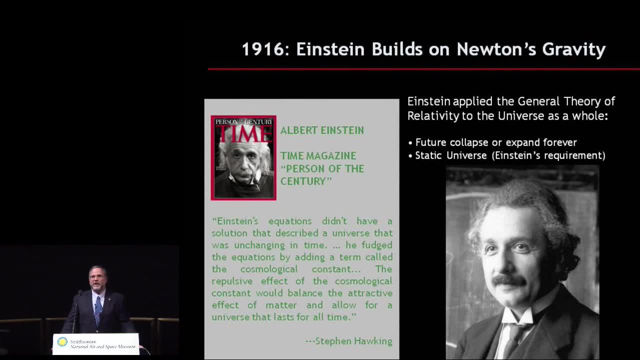 understand, and there was. there was a lot he did understand. so this is where Albert Einstein came in. Albert Einstein built upon Newton's laws of gravity with a new theory of gravity called the general theory of relativity- it's a fancy name for a theory of gravity- and he applied this gravity that he came up. 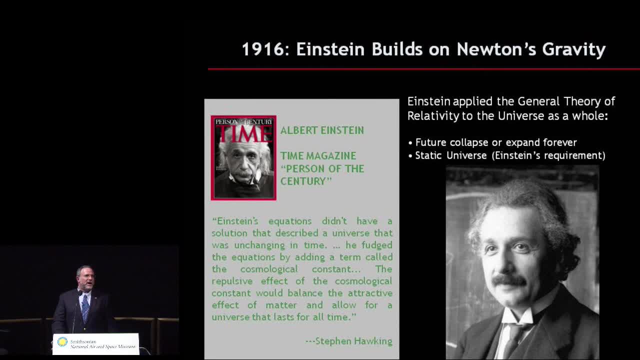 with to the universe as a whole, and he was surprised that the answer that he got was that the universe should be expanding or it should be contracting. those are the solutions to his equations. and yet at the time there was no evidence that the universe was anything but static. it was there today it was. 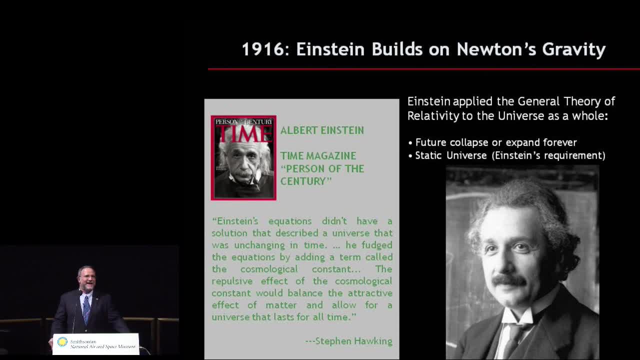 there yesterday there was no evidence, and so he decided he made a mistake in his equation and that he had to fix it. and so he built into his equations a fix, which was an extra term in the equations, that acted like an anti-gravity. so if you think back to Newton's question of why the stuff in 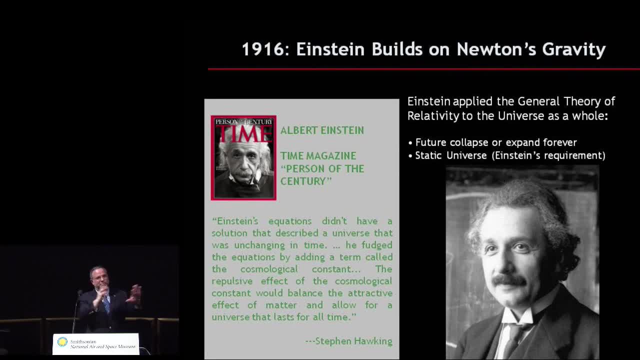 the sky just doesn't fall together, Einstein puts in an anti-gravity that pushes it back apart again. so I think exactly balances the gravity with the anti-gravity, and that was his theory. back in the year 2000, Albert Einstein was named by Time magazine as the person of. 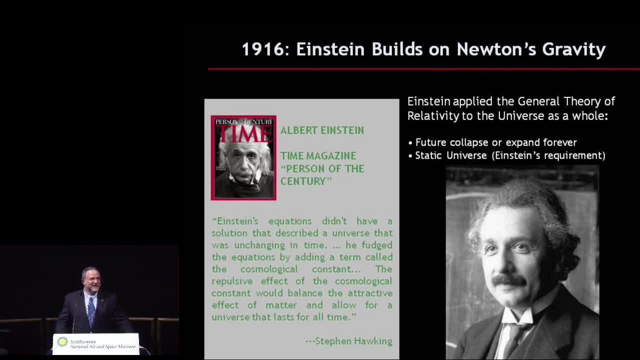 the century. this was a personal victory for us physicists around the world. you know, eat your heart out rock stars. you know it's a physicist, politicians sorry. and there was an article in this issue of Time magazine by Stephen Hawking that said Einstein's equations didn't have a solution that described the universe. 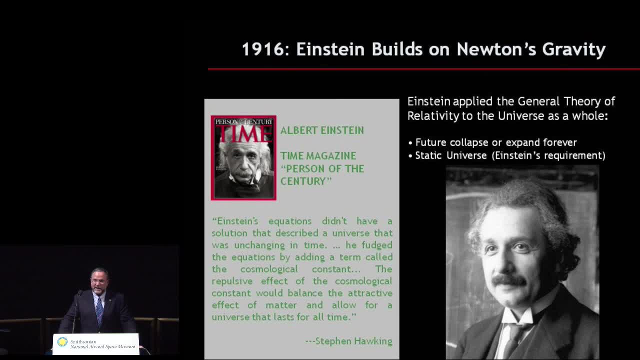 that was unchanging in time. he fudged the equations by adding a term called the cosmological constant. the repulsive effect of the cosmological constant would balance the attractive effect of matter and allow for a universe that lasts for all time. well, if we fast forward to 1929, the great American 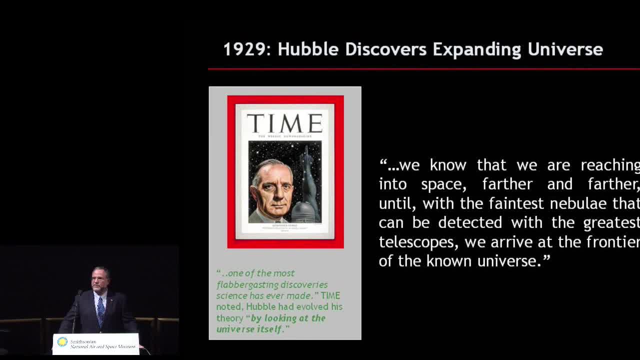 astronomer, Edwin Hubble, discovered that the universe in fact is expanding. here is Edwin Hubble on the cover of Time magazine and, and the article about the universe has been published on the screen and it's been published in various journals. this is the first ever and the first article that the time writer had. 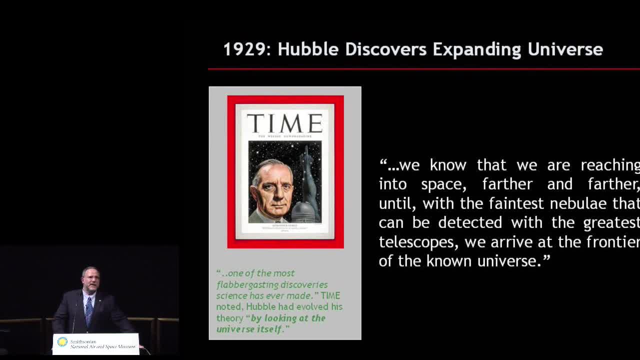 here said that this was one of the most flabbergasting discovery sciences ever made, and Time magazine noted that Hubble had evolved this theory- quote- by looking at the universe itself. so there's two things about this that caught my eye when I read this. one is the word flabbergasting. I think that's a terrific. 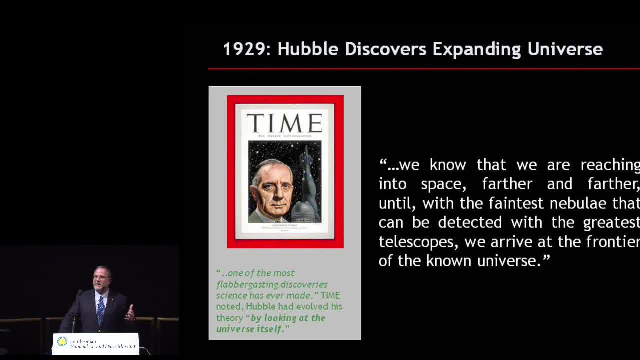 word not used enough and you should all use it as much as possible. it is take. when I read that he evolved his theory by looking at the universe itself, I read that and I go: well, how else would you do it? And then I realized, I thought back and 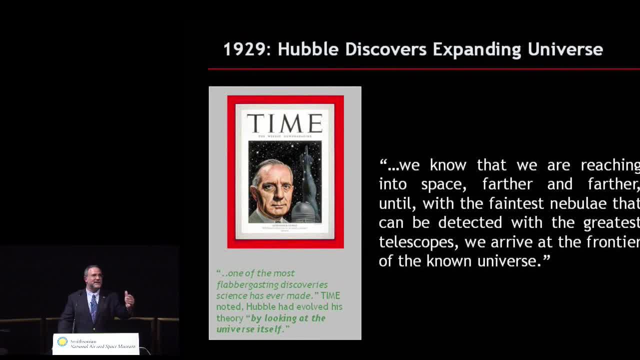 said: well, that's not so obvious. As I said at the outset, it's not obvious that we should be able to learn about the universe from here on Earth And in fact I think a lot of people thought of that picture of the armchair as the way you could ever possibly know the universe. 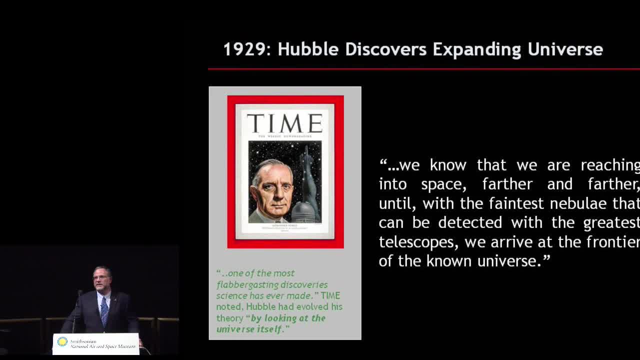 And I think this writer for Time Magazine had that sense that this is, and I think he's right. this is an amazing thing that you can learn about the universe by actually looking at it and making measurements. It is an amazing thing. Hubble said that we know that we are. 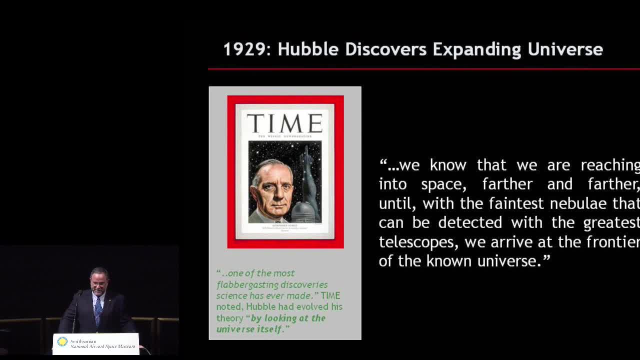 reaching into space farther and farther until, with the faintest nebulae that can be detected with the greatest telescopes, we arrive at the frontier of the known universe. One of the first things that Hubble said was that we are reaching into space farther and farther. 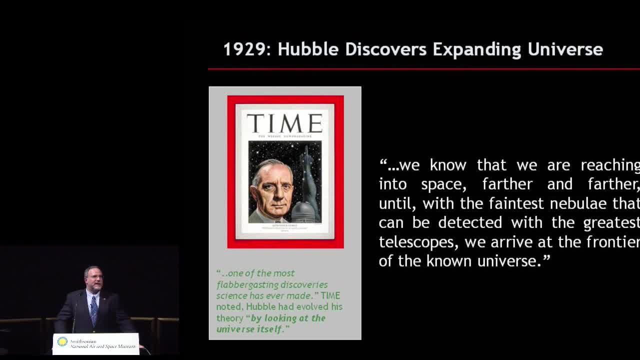 One of the things that I hope to describe to you this evening is that what was the frontier of the known universe to Edwin Hubble is now our backyard. We have driven the frontier of the known universe far, far beyond what Edwin Hubble probably could ever have imagined. 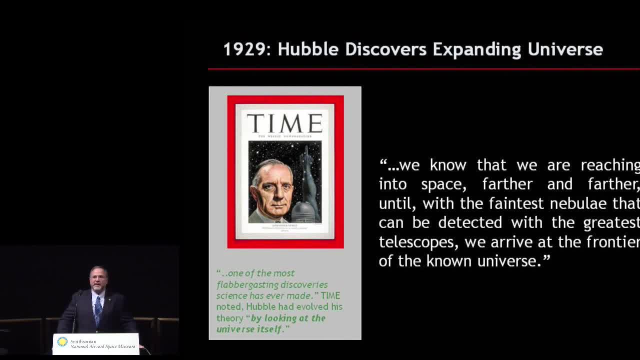 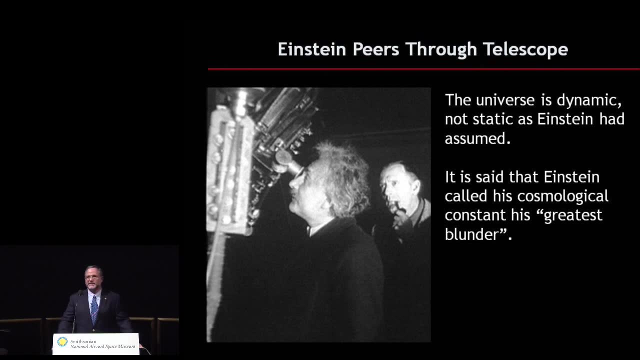 And this is the progress that we see over the years, just from generation, building upon the work of earlier generations. Well, remember, Albert Einstein introduced this extra term in his equations to make the universe static. and now Edwin Hubble says it's not static after all. And so there's Einstein looking through the telescope and it's reported. 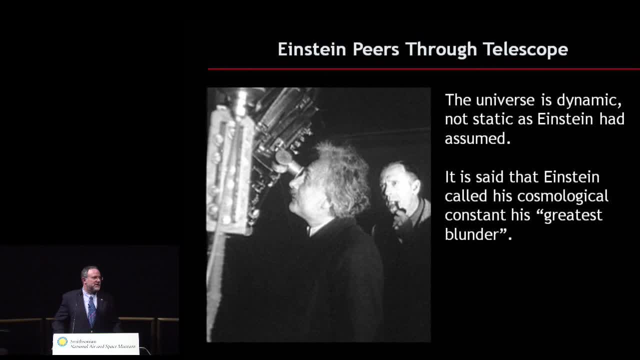 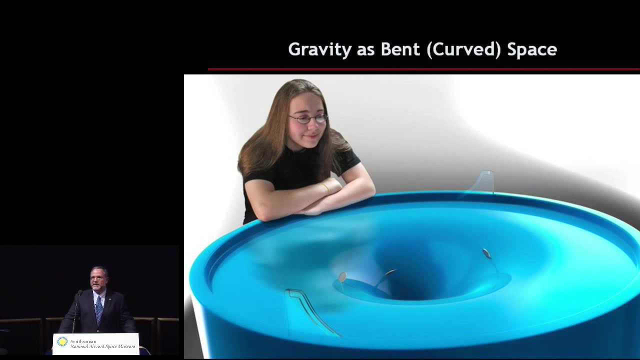 that Einstein. he clearly realized that his cosmological constant was not needed, and it was reported that he said that this introduction of this cosmological constant was his greatest blunder. So how did Einstein think about gravity? He thought about gravity. What was the idea? I don't know if you all have seen these, or 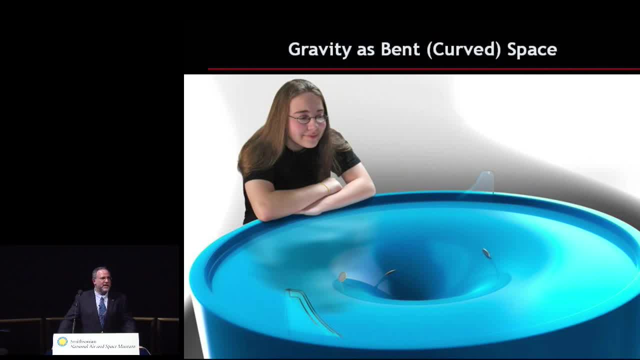 played with these kind of toys. They used to be around in shopping malls and maybe airports and things. But basically the idea is that you launch a coin on the launcher and it starts rolling and it goes around and around and around and around on this kind of vortex. 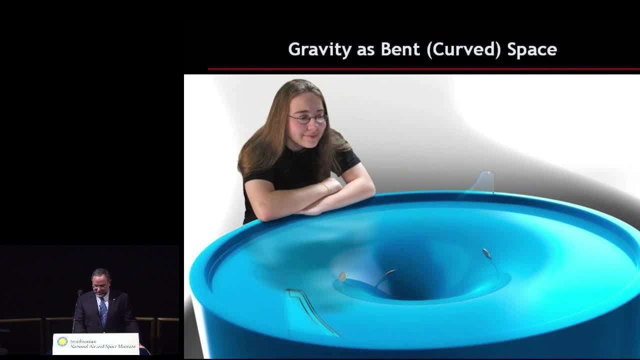 shaped surface, And I think you can imagine, even if you haven't played with one of those. I think you can imagine it. But- and this is how Einstein thought about gravity- Einstein thought about gravity as curved space, that having material curves the space around it and then objects move. 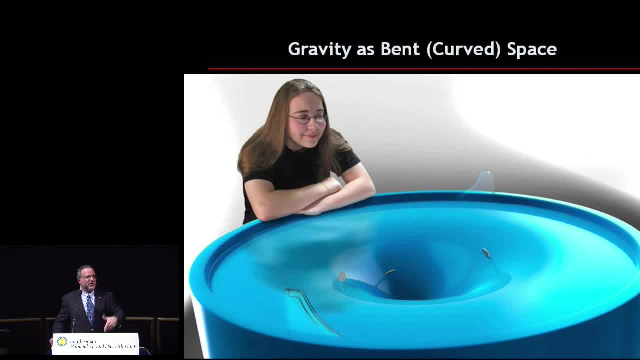 in the straightest line they can. on a curved surface, Normally you roll a coin and ideally it goes straight, But if it's on a curved surface it can't do that. So here's our sun, bending the space around it, because Einstein says that mass bends. 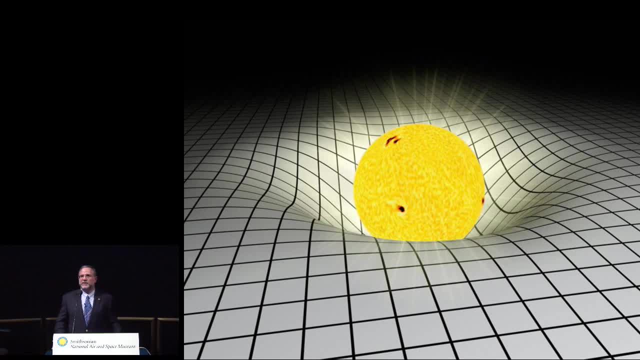 space And then the Earth, like the coin, goes around and, around and around. And this is the Einstein picture of how gravity works. and this is Einstein's answer to Newton who said he didn't understand how the Earth knew the sun was there. Einstein says it knows because the 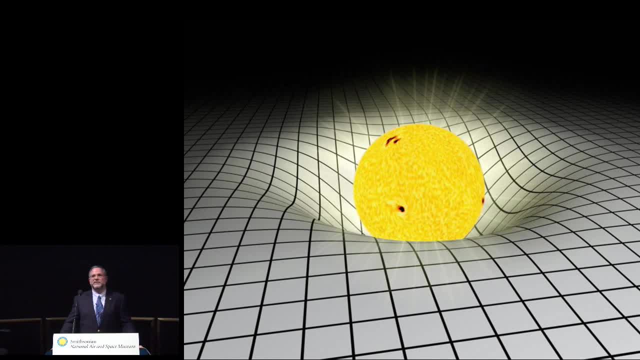 sun is bending the space around it and the Earth has to follow the straightest path it can in bent space. Sir Arthur Eddington was a big fan of Isaac Newton and relativity And he said: you know, if you're going to be able to bend space, you're going to have to follow the straightest path. 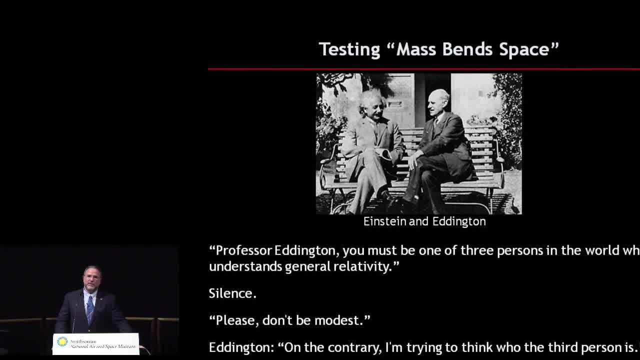 it can in bent space. Sir Arthur Eddington was a big fan of Isaac Newton and relativity and he said: you know, if you're going to be able to bend space, you're going to have to follow the straightest path it can in bent space. and the Earth has to do that and the Sun is bending at an 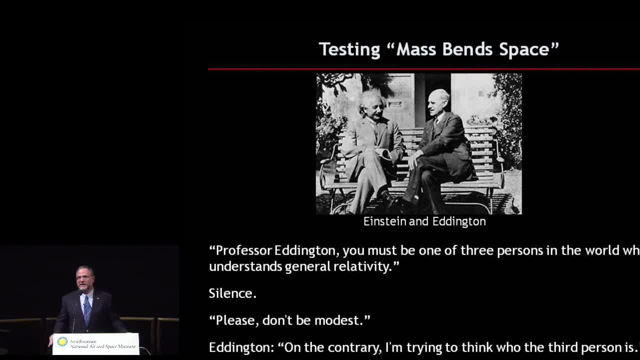 angle when it has to follow the straightest path it can, and it's a". It's one thing to come up with an idea, It's another thing to know, if it's true- and there's a story told about Eddington- that somebody asked him. Professor Eddington, you must. 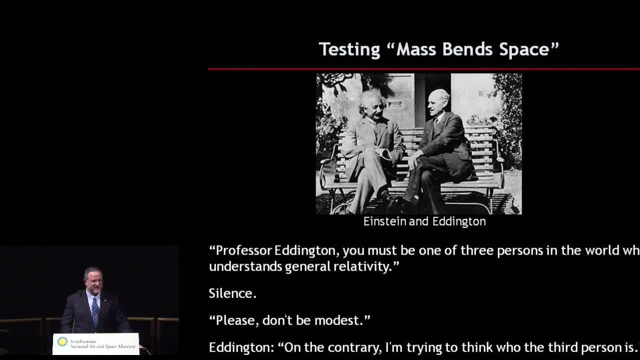 be one of the three persons in the world who understands general relativity. Silence, Please don't be modest. On the contrary, I'm trying to think who the third person is. So Eddington had an idea for how to test the theory. 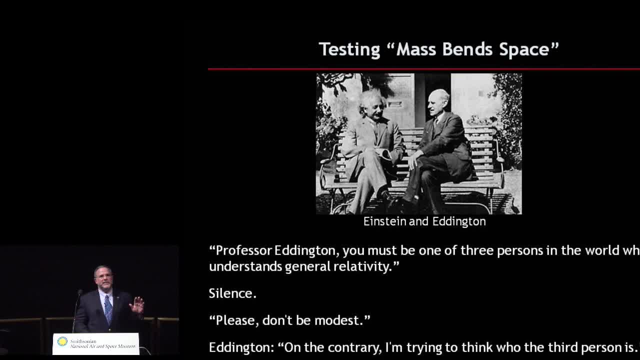 He thought about: wouldn't it be good if we could observe a star whose light is going kind of by the sun, to see if the light gets bent by this supposed curved space from the sun, If we see the position of the star move over because of that? 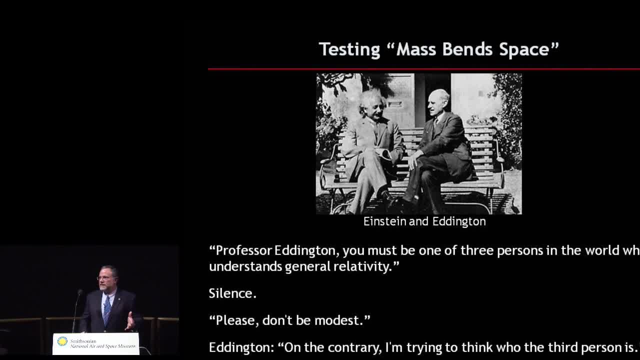 then we know that Einstein was right. The only problem with this idea was that you can't see stars behind the sun or near the sun, because the sun is so bright. But Eddington knew that there was an eclipse coming up and he realized that for a moment you would be able to see the stars. 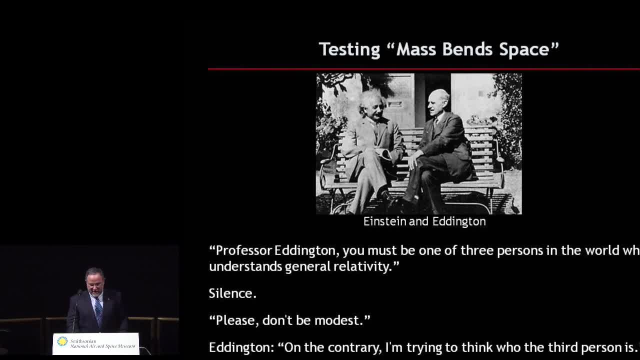 as their starlight grazes by the sun, And so he mounted an expedition to Brazil to try to do this experiment. So here's the idea, Here's our picture of the sun. Normally, the starlight would go straight and you would see it there. 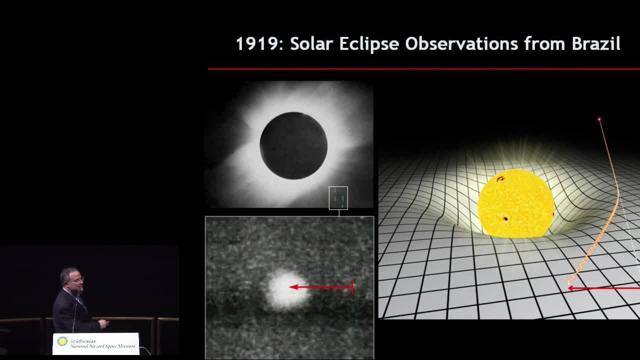 but if it has to go by the sun it's going to curve a little bit. Now, Newton's laws of gravity work on objects that have mass. If an object with mass went by, it would do this, but light doesn't have mass, so it shouldn't do that. 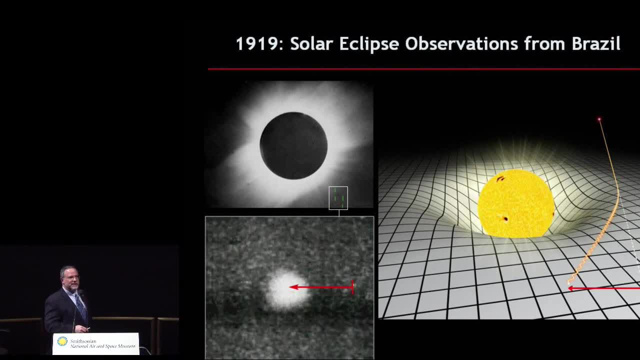 And so this is a pretty good test of Einstein's theory of whether there's curvature there. And then here's the eclipse: There's a star, and its position is moved over from here to here Because of the bending the curvature of the space near the sun. 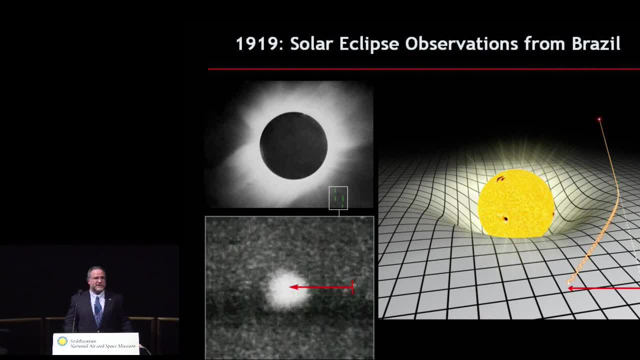 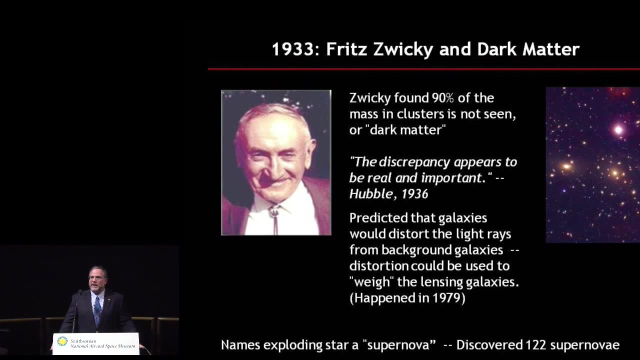 So this tested the idea- Einstein's idea- that massive objects bend the space around them and that affects how things move. I'd like to fast forward now to 1933 and a tremendously underestimated scientist named Fritz Wicke, And Fritz Wicke basically invented the idea of dark matter. 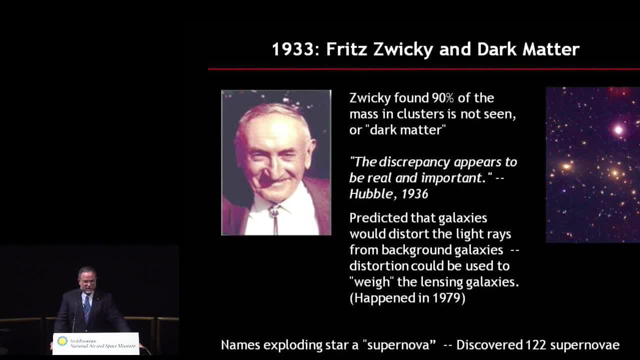 He was, and a lot else too. He was studying a cluster of galaxies. These are a bunch of galaxies that are close to each other because of their gravity pulling them together, And he measured the speed of these galaxies and he was astounded by how fast they were moving. 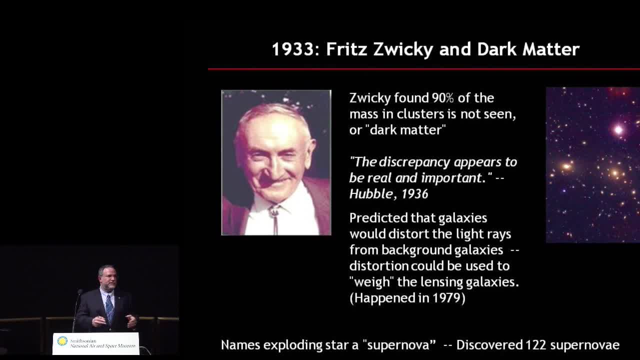 In fact, they were moving so fast that they should have long ago just flown off into space. Why are they still together? And Wicke realized that the only way to explain this is that there must be a lot more mass, a lot more matter in this cluster. 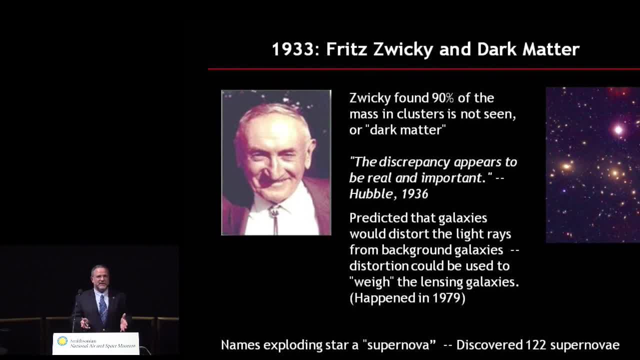 than he can see light from. So he decided the only way this makes sense is if 90% of the mass in clusters is something that he called dark matter, something that's not emitting light but has gravity, And so this was one of the earliest. 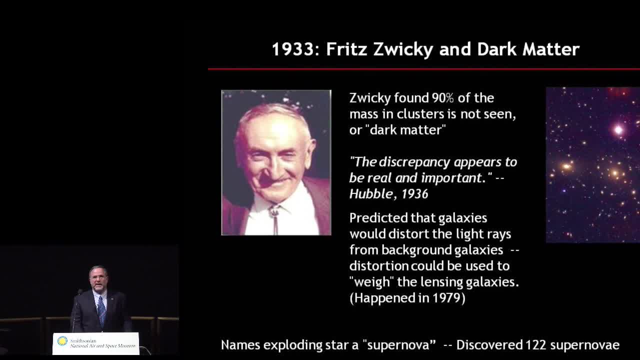 substantial introductions of the idea, and again the words dark matter came from him. The discrepancy appears to be real and important. Hubble said in 1936.. Now, as Wicke didn't just stop there, he also had an idea. 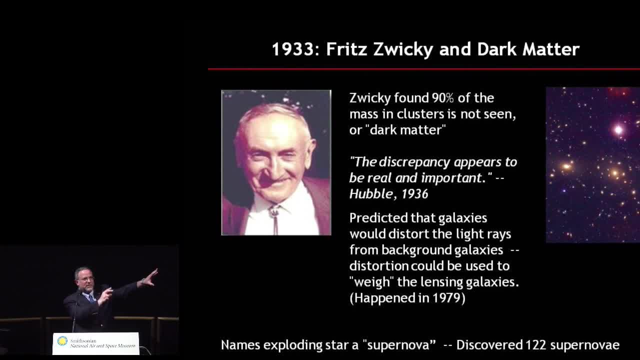 He said: well, if we had two galaxies, one farther away and one closer, and the light from the farther one came by the one that's closer, it would bend the light of the distant galaxy and we could tell by the amount the light has bent. 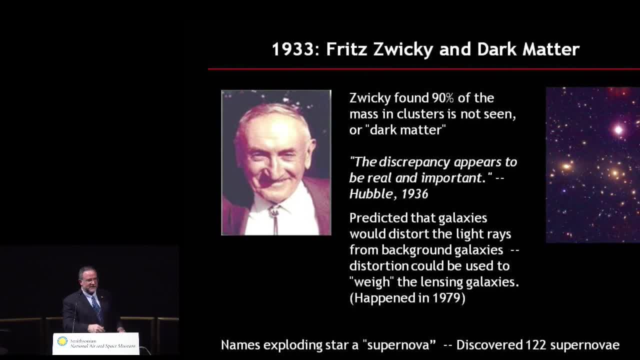 how much the galaxy weighed. So we can weigh entire galaxies this way. And he was absolutely right, but way ahead of his time. It didn't happen until 1979.. And just to finish off with Zwicky, he's also the guy that came up with the name. 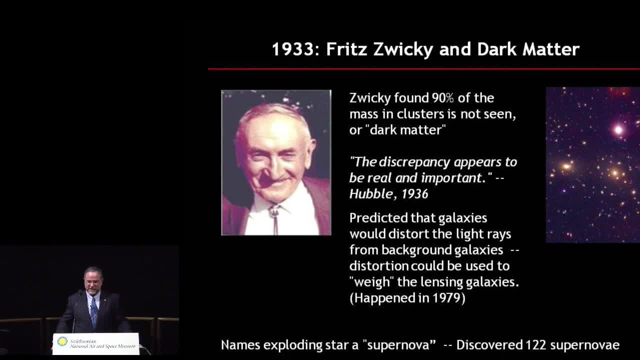 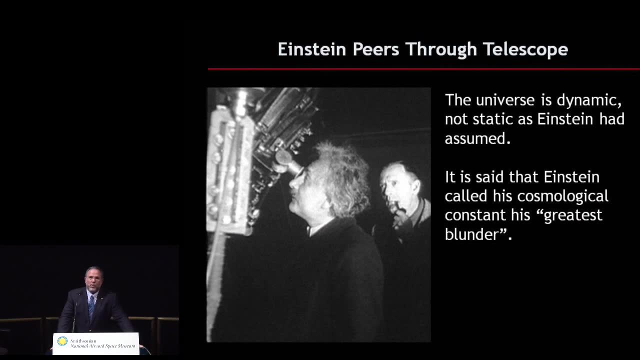 supernova for exploding stars, and he discovered 122 of them himself, And much more about him too. You don't hear his name too much, but he was really extraordinary. So let's get to the heart of the Big Bang Theory. We know from Hubble that the universe is expanding. 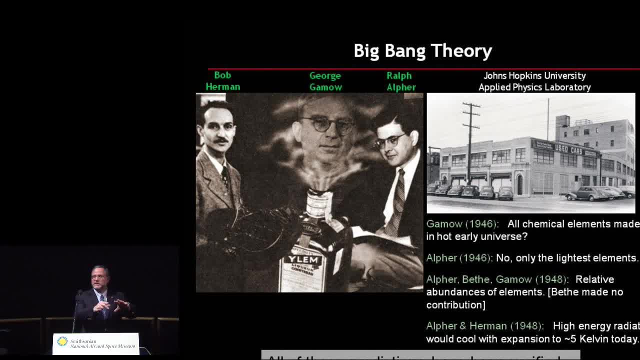 and if you think about material being in the universe and the universe expands, then the density of material drops. You have the same material spread over more space. Not only that, but if you have heat in the universe and the universe expands, the amount of heat drops. 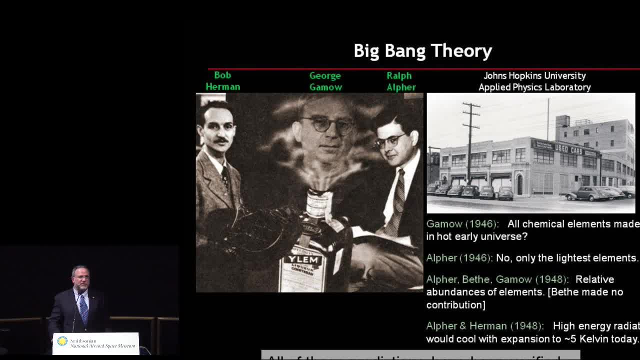 the heat density drops and so the temperature of the universe drops. So the guy George Gamow, coming out of the bottle here like a genie, had an idea in 1946. He was a professor at George Washington University near here. His idea was that maybe in the early universe 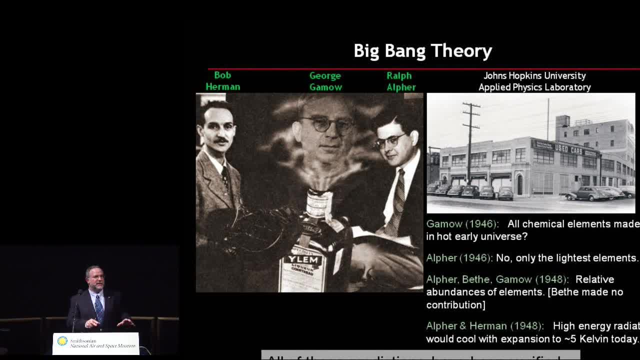 since it had to be hotter and more dense, because, looking back from this expansion, maybe all of the elements in the periodic table of elements was formed in this dense, hot early universe because it would be so hot and dense that it would act like a nuclear fusion reactor. 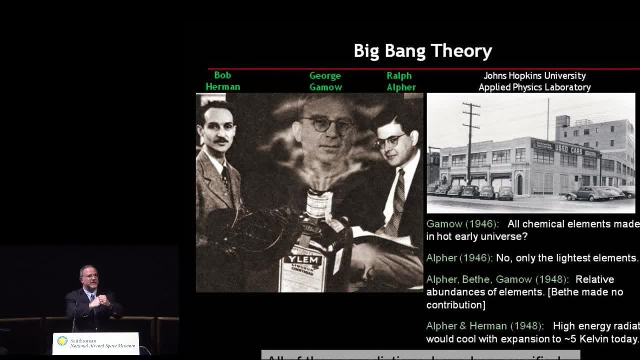 You would take hydrogen and another hydrogen and you'd make helium. You take the helium, you add another hydrogen, you have lithium, and on and on and on and you make all the elements. He had a graduate school student, Ralph Alpher, shown here. 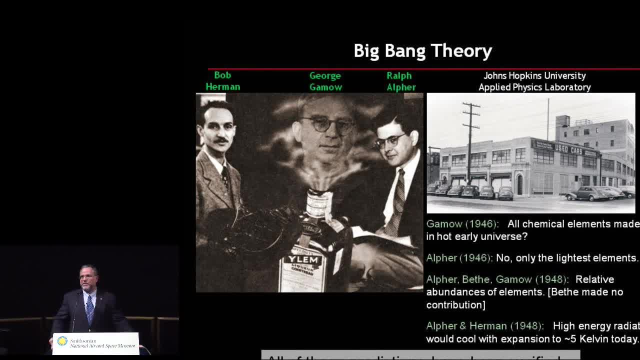 and he assigned Ralph Alpher the job of calculating this idea, And Ralph Alpher worked at the time at the Johns Hopkins University Applied Physics Lab shown here. This is near what is now the Silver Spring Metro Station, near Georgia Avenue and Carlsville Road. 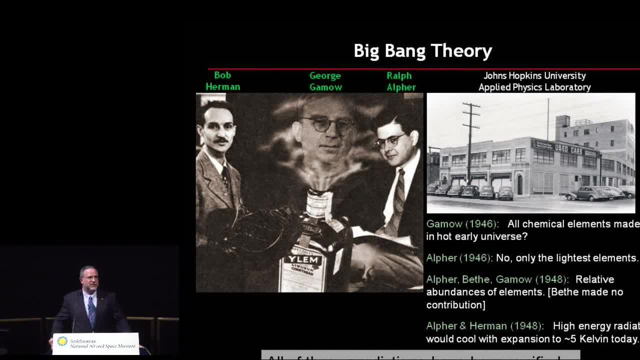 And it says used cars on it because it used to be a used car lot before it was taken over for World War II weapons research. They did not change the sign to say secret World War II weapons research. So Alpher did the calculation and reported back to his thesis advisor. 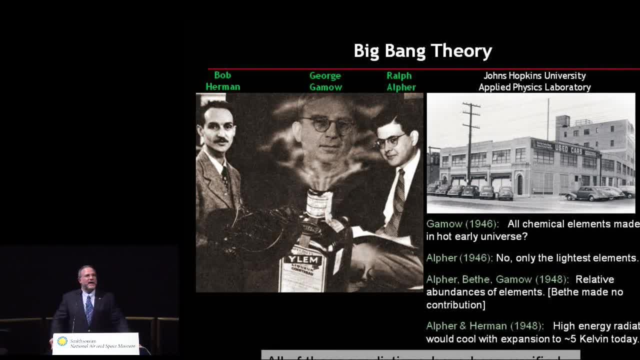 no, you were wrong. You can't make all the elements that way, because you've got a battle against time to put these elements together, one after the other, fusing one to the next, and you don't have enough time to do it. 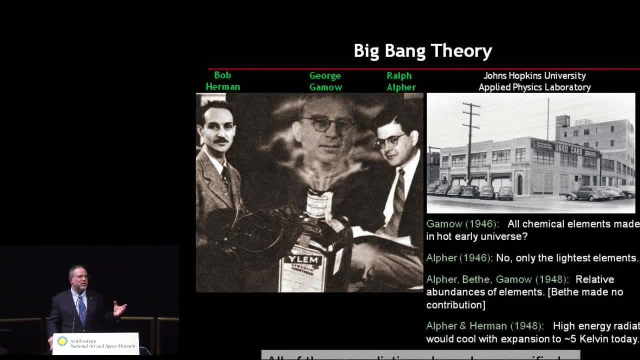 The universe is expanding, the temperature is dropping, the density is dropping and, most importantly, to do this you need free neutrons, and free neutrons live for only 14 minutes. You've got 14 minutes to make all the elements. 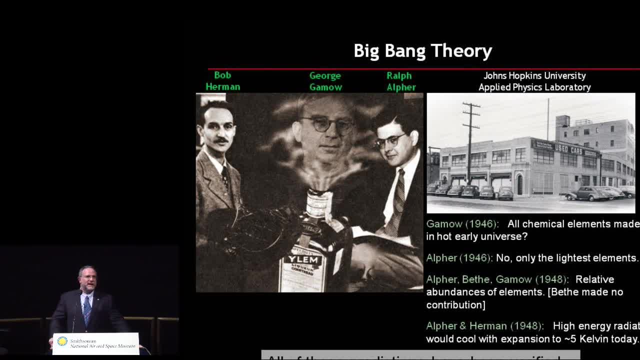 can't be done. So what we know today is that the lightest chemical elements- helium, lithium, for example- were made in the early universe. but all of the heavier elements, like all of the carbon you're made out of, I'm made out of the room. 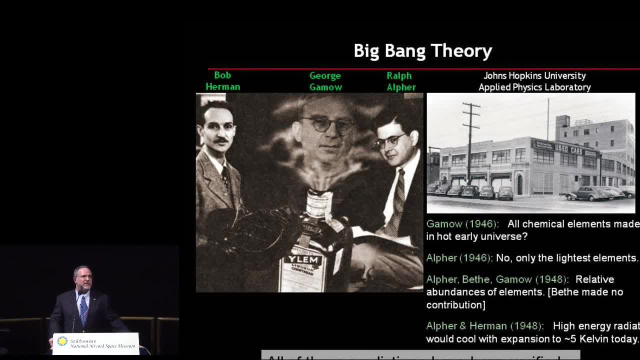 all of the carbon in your bodies comes later on from stars. Every carbon atom in your body was made in a star somewhere. The universe only made the lightest elements. The next paper was written to show, to actually give the numbers for the relative abundances of these elements. 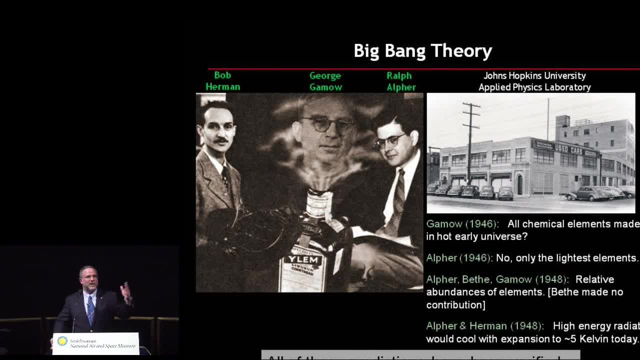 How much hydrogen, how much helium to hydrogen, how much lithium to hydrogen, if you went out and measured what the ratios should be. Now this paper. the authors were Alfer and Hans Bethe and George Gamow. Now, Hans Bethe knew nothing about this paper. 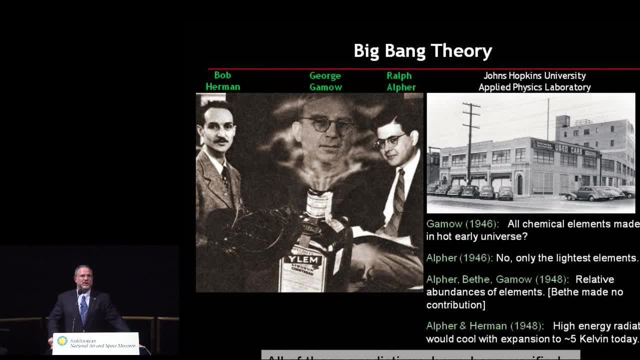 and was not didn't do the work at all. His name was put on completely as a joke by George Gamow because he wanted the authorship to be Alfer Bethe Gamow. Today that would be considered unethical, But George Gamow was a jokester. 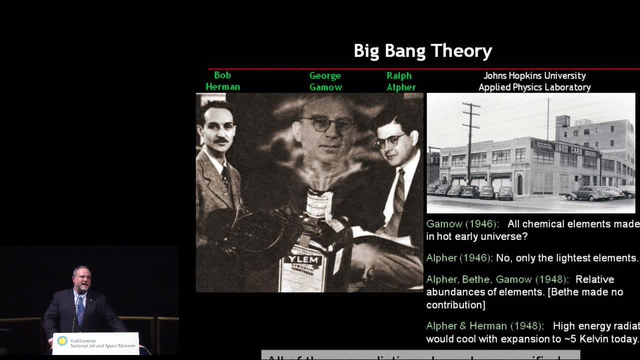 In 1948,, Alfer and Herman went on to point out that if the early conditions of the universe were like a nuclear fusion reactor- very hot and very dense- then you would constantly have radiation coming off of the matter, and that that radiation didn't just 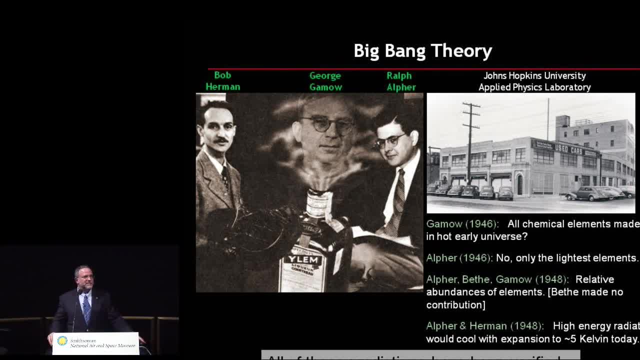 disappear, but stayed in the universe And as the universe expanded over time, that high energy radiation kind of calms down And they predicted that the sky today should be filled with this radiation all over the sky and that it should have cooled to an equivalent temperature of five degrees. 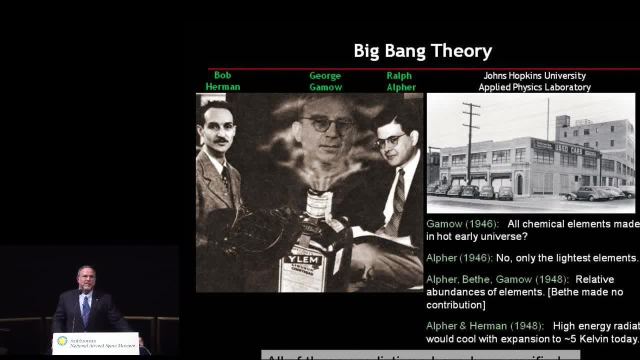 above absolute zero, which happens to fall in the microwave part of the spectrum. So they predicted that there's a microwave glow across the sky left over, And they even looked into the possibility of observing it and were told that it was too faint to observe. 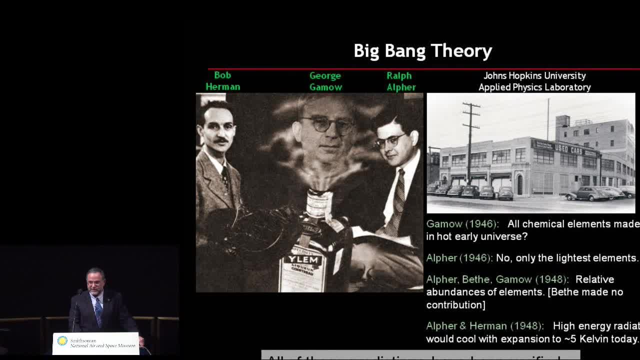 Well, since then, it has been observed, as I'll be telling you. In fact, every one of these predictions has been come true, has been shown to be true. And then the collection of all of this is what, effectively, is known as the Big Bang Theory. 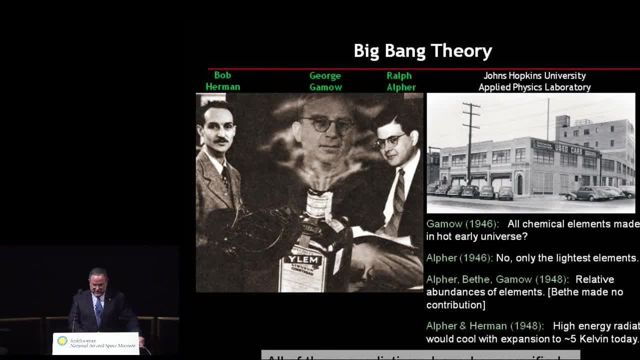 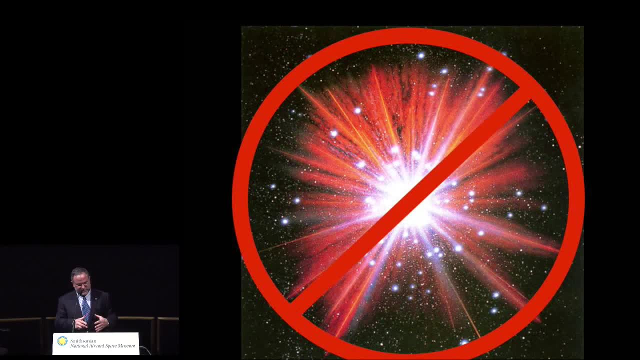 And so when you see pictures like this- and maybe you know the universe forming in a universe that's already there- I have no idea what this picture is showing. One thing is for sure: it's garbage. So this is not what the Big Bang Theory is. 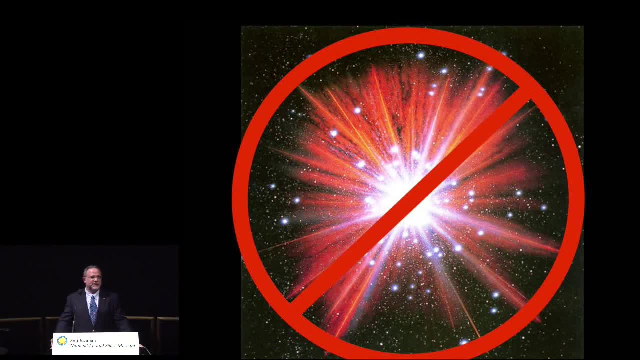 And I've dealt with the media a lot over the years And when they come to do things you know, I can tell you there's nothing they'd rather show than an explosion. Watch TV you'll see explosions and car chases and all kinds of things. 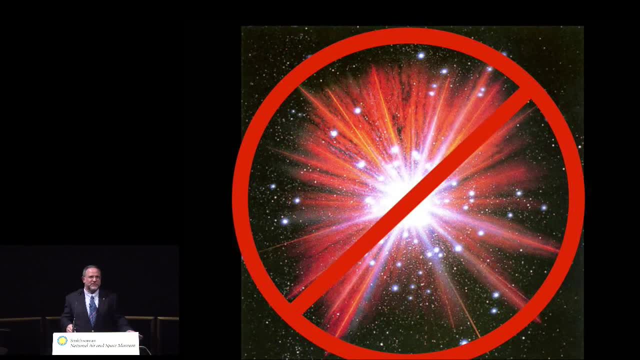 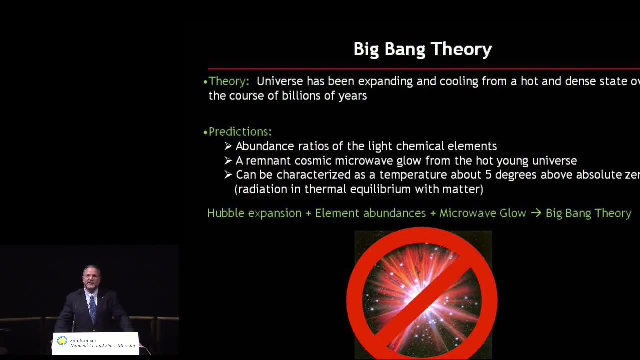 And when I tell them: but there was no explosion, they go: well, we're going to show one anyway. So it's very interesting, Very confusing. So what is the Big Bang Theory? So the way I would state it and different people would say it differently- 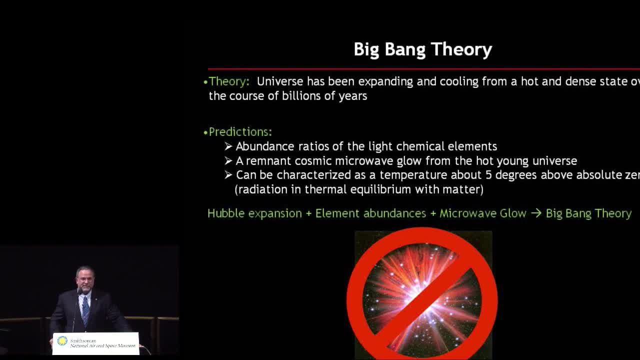 but I would say the statement of the theory is that the universe has been expanding and cooling from a hot and dense state over the course of billions of years. It's a statement of the expansion and cooling which is the framework for all of the results. 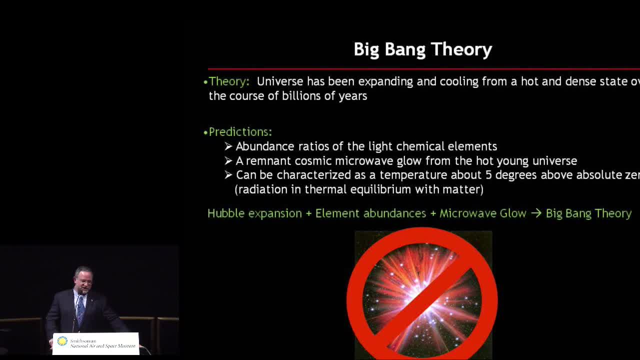 that I was just telling you about and that this framework makes predictions. It makes the predictions of specific abundance ratios of the light chemical elements. It predicted that there should be a remnant afterglow of microwaves from the early universe and it predicted that these microwaves 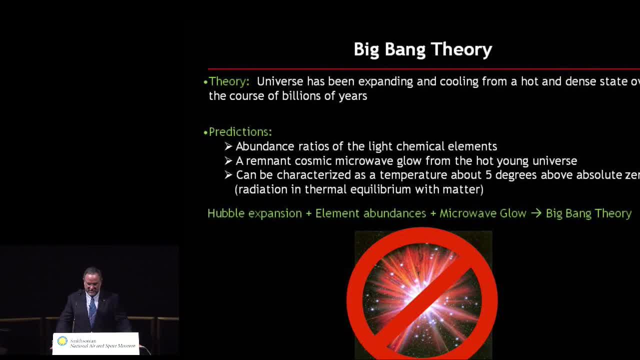 should be characterized by a temperature somewhere around five degrees above absolute zero. This is the result of radiation that's in equilibrium with matter, as it was early in the universe, And we love theories that make successful predictions. The others we don't talk about anymore. 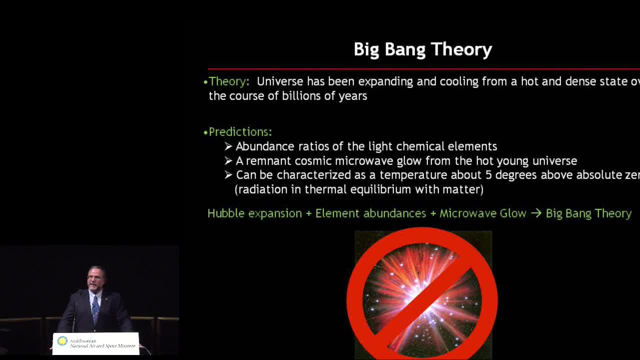 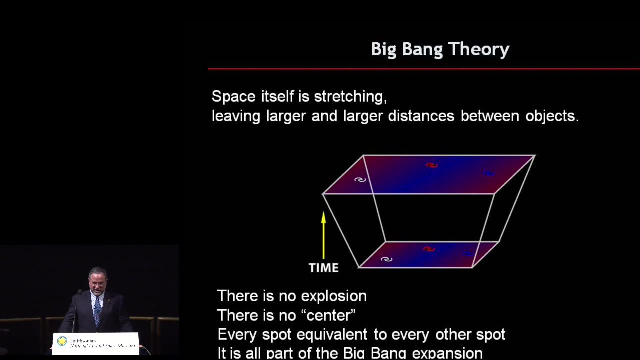 So the combination of the Hubble expansion, the light element abundances, which have been verified, and the microwave glow, which has been discovered, all support the idea of the Big Bang Theory. So in the Big Bang Theory, it is space itself that is stretching. 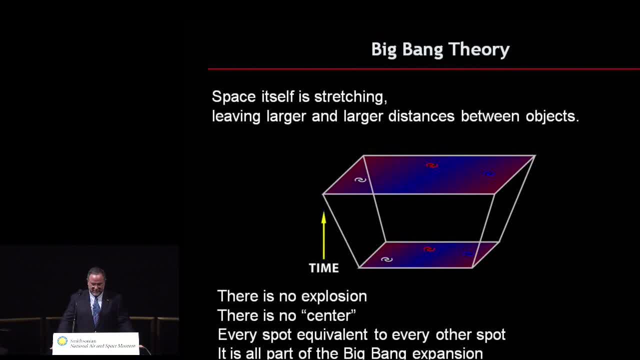 leaving larger and larger distances between objects, And this is true everywhere. In this picture. there is no explosion, There's no center to the universe. unlike that picture, This happens everywhere, And every spot that you pick in the universe is just like every other spot. 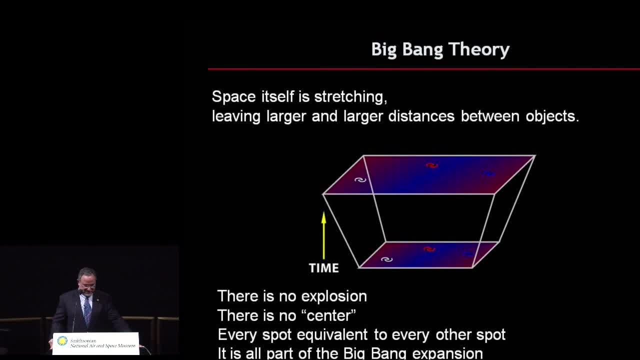 Everything in the universe is participating in this expansion, So here's a way of illustrating it. Here's objects in the universe, and the whole picture just expands. I wish my screen were bigger, but ignore the fact that they're going off the edge of the screen. 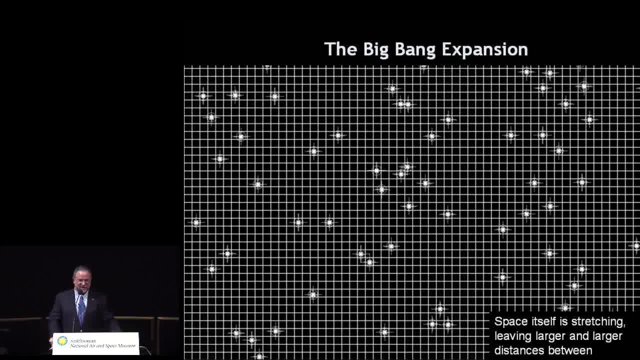 So if you just pick with your eyes any two objects in the screen there- and it doesn't matter which two you pick and you just follow them with your eyes- you will see that over time they get farther and farther apart from each other. 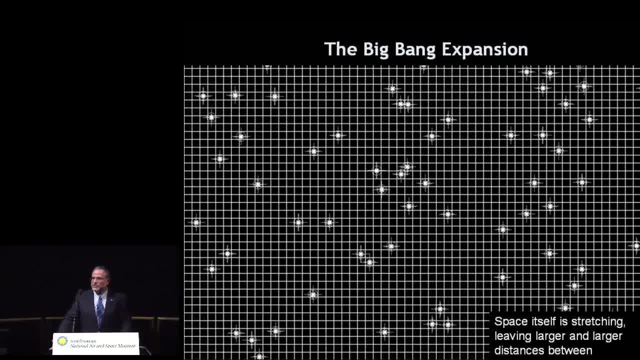 and it's true for every pair of objects. It's also true if you pick any one object, that it looks. if you imagine living on that object, it looks to you like everything is moving away from you. It's not something you said. 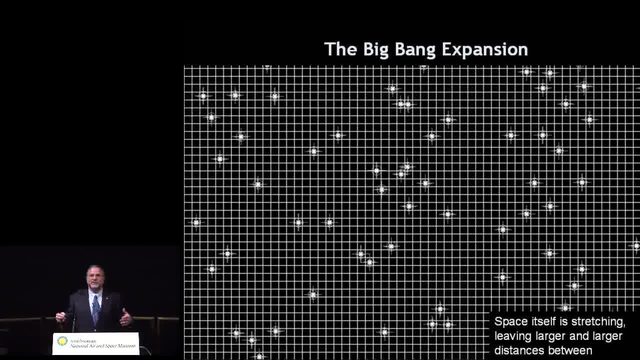 It's the fact that space is expanding, And that, again, is true of every object. So when Edwin Hubble saw that all these objects are moving away from us and the universe is expanding, he assumed that it wasn't just us, that you would see this from everywhere else as well. 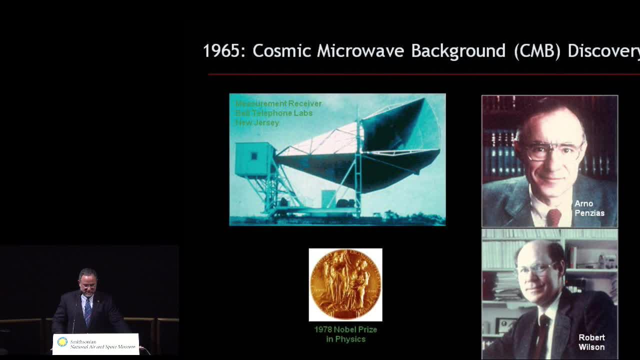 The discovery of the cosmic microwave glow was by Arno Penzias and Bob Wilson in 1965, for which they won the Nobel Prize in Physics. This was an accidental discovery. They were not looking for it. They were annoyed by this extra stuff. 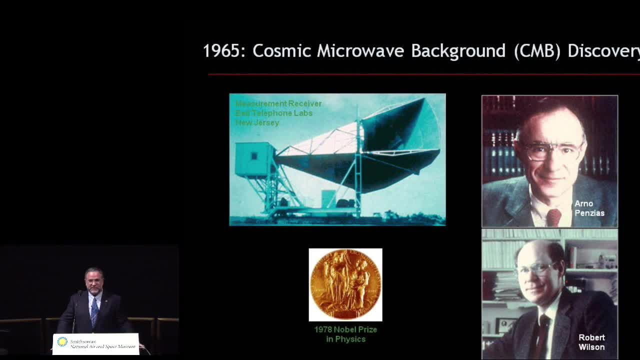 that they were seeing all over the sky, and this contraption at the Bell Telephone Lab was picking up. However, they did make a discovery and did win the Nobel Prize for it. So this discovery really nailed the Big Bang theory, especially against its competitor. 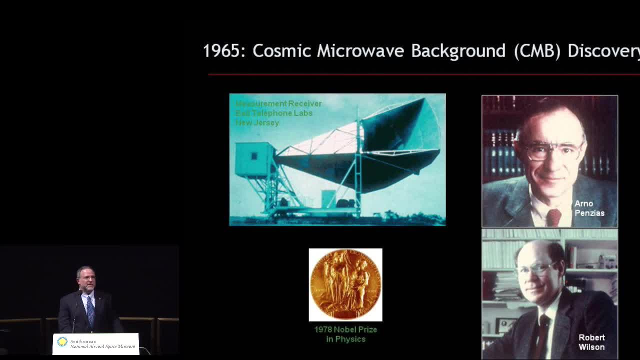 which was called the steady-state theory. I don't have time to go into that, but again, this was predicted by the Big Bang theory and it was hard to manufacture in the competing theory. So this left a question If I represent Penzias and Wilson's measurement. 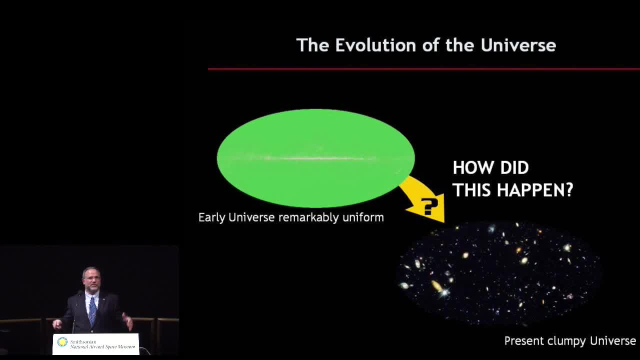 on a map of the whole universe. Now it's hard to show a whole universe on a slide, so it's a projection here, just like you were projecting the surface of the Earth onto something And I made a weather map out of it, so that 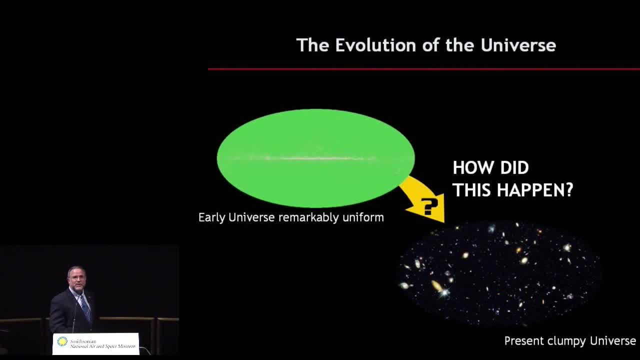 So you would have basically a very boring weather. You would have the same temperature everywhere in the sky. Penzias and Wilson actually measured a temperature of 3 degrees above absolute zero. Compare that to the prediction of 5. Pretty close. And they measured this 3-degree temperature across the sky. 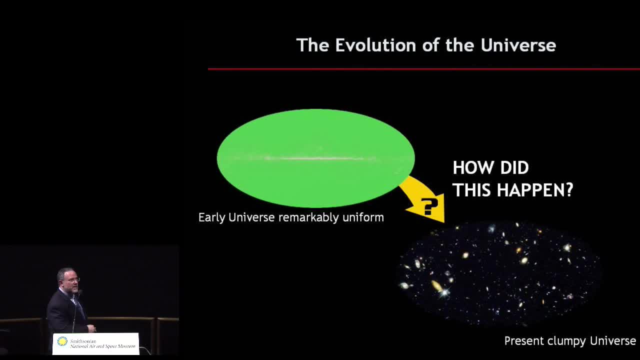 except for this band across the middle, which is extra microwaves that come from our Milky Way galaxy. They're in the way And Penzias and Wilson understood what that was, But the rest of the sky is still glowing in microwaves. 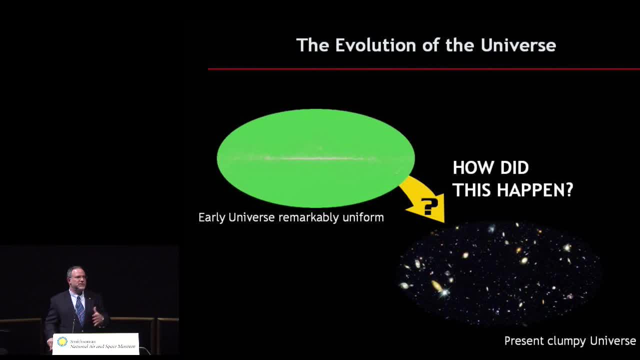 Penzias and Wilson could measure that this glow was uniform, toward their measurement error, which was about 10%. But we know that when we look at the sky today with the Hubble Space Telescope, the universe is very clumpy. We have galaxies. 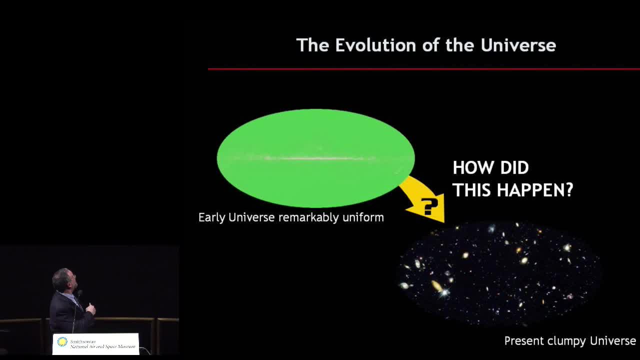 It doesn't look at all smooth, And the question is: how did the universe get from being so smooth to being so clumpy? And the answer was felt to be gravity. But for gravity to make these clumps, there had to be some initial fluctuations. 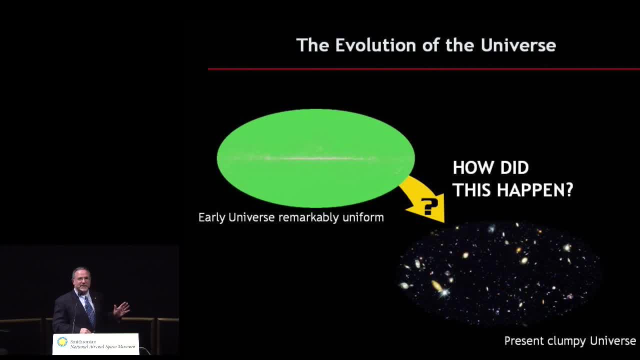 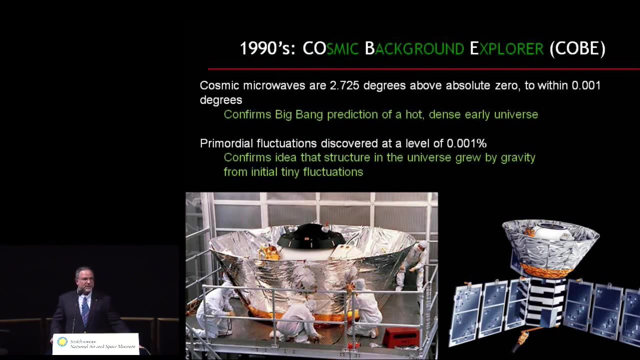 in that early universe. Something had to be there ever so slightly to allow some spot to be denser than the spots around it and for the gravity to build up the objects. And people searched for 27 years to find it and it was finally found by the COBE satellite in the 1990s. 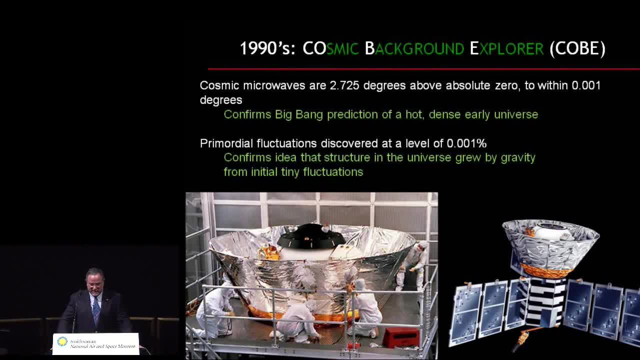 The COBE satellite had several discoveries. One is that it measured once again the temperature of the cosmic microwaves. Remember, predicted at about 5.. Measured by Penzias and Wilson, discovered about 3.. Now measured by COBE as 2.725.. 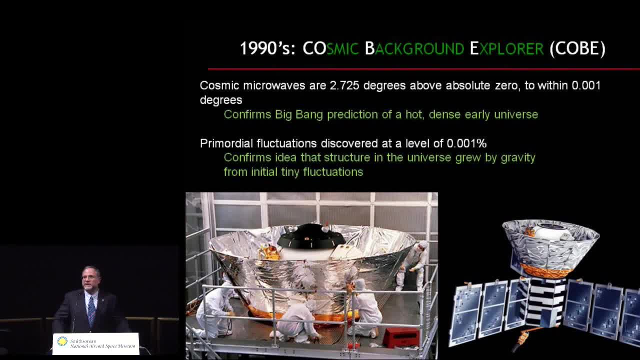 Very accurate measurement: give or take 0.001 degrees. Notice the progress being made in our studies of cosmology, from the point where maybe we have to sit in an armchair and can't measure anything to now making very precise numbers about the universe. 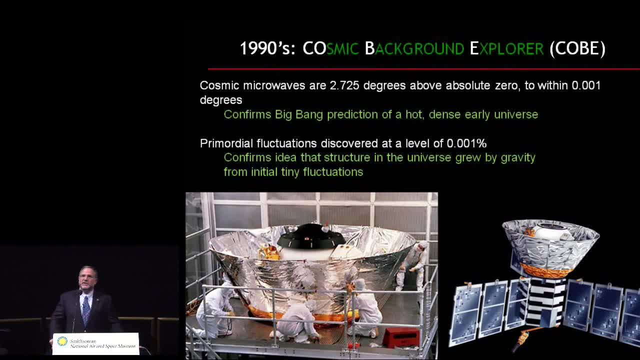 And so the idea that there is this radiation that is characterized by a temperature is very strong confirmation of this big bang: hot, dense, early universe. But also, as I mentioned, the COBE satellite discovered for the first time the tiny variations in the early universe. 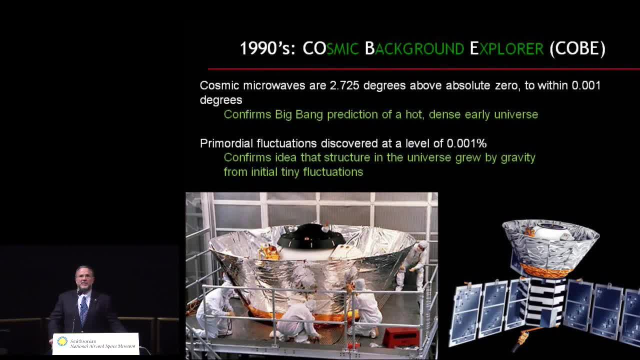 the tiny temperature differences, density differences from spot to spot on the sky, And the reason it took 27 years of effort to do it is because Penzias and Wilson put a limit of 10% on their measurements and the answer wasn't at 5% or 1%. 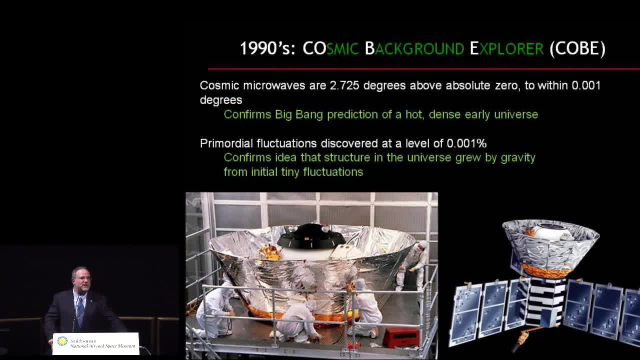 It was at 0.001%. These variations are tiny, really tiny, and it took a long time for the technology to develop to the point where they were detectable, And so COBE detected these tiny, tiny fluctuations. So you have this 2.725 degree temperature level. 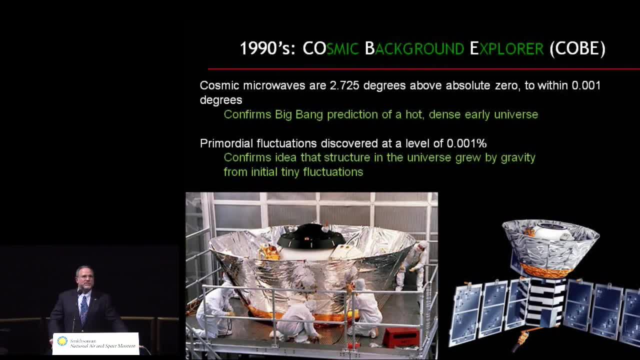 and tiny, tiny little fluctuations on top of that, which represent little, tiny density differences, from which all of the structures in the universe grew- Clusters of galaxies, galaxies, planets, us all- because of those tiny little fluctuations. Well, once COBE discovered these fluctuations, 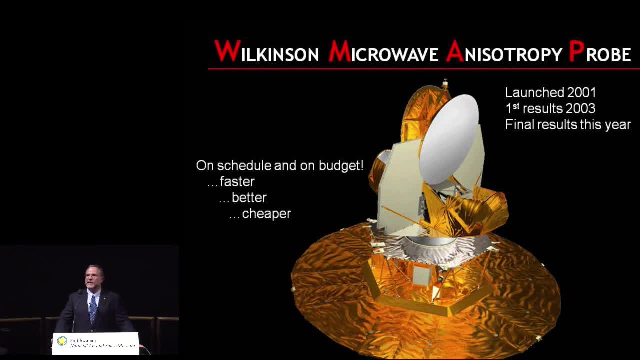 a group of us decided to propose to NASA a follow-up satellite called WMAP- and this was in the era of what was called better, faster, cheaper satellites- and we managed to finish building this one on schedule and on budget. That wasn't necessarily what happened to all of them. 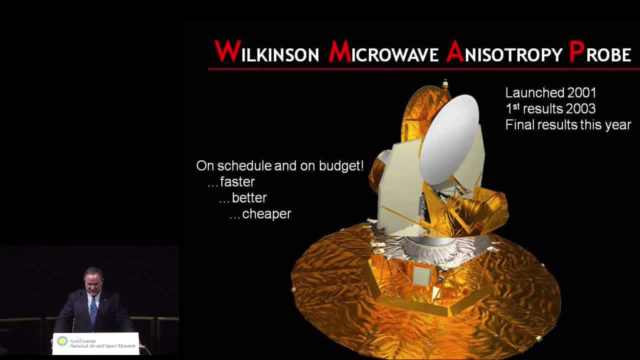 but this one did well and it launched in 2001, and we released our first results in 2003, and our final results are going to be released this year. The satellite is no longer operating, But I'm going to tell you about the results. 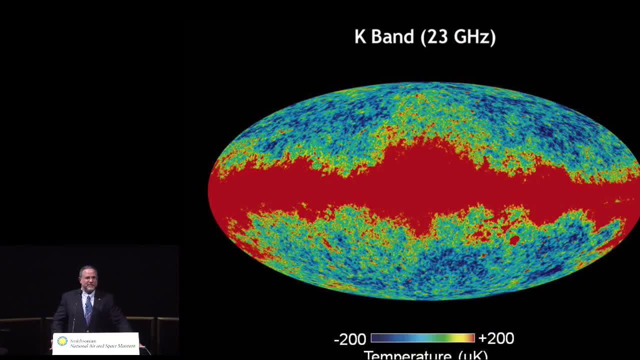 First of all, it makes these maps of the full sky and it makes it in five different bands, and what you can see as I cycle through them is this: the most obvious thing is this red stripe across the middle, and this is again microwaves. 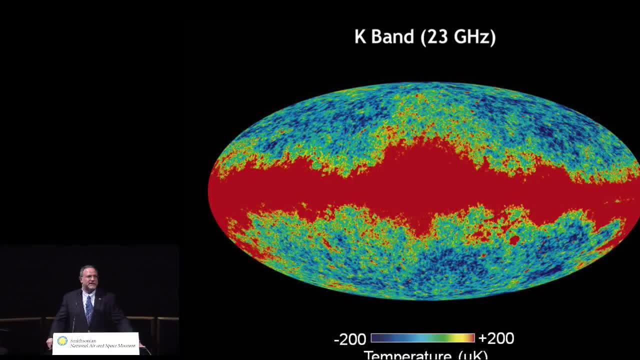 from our own Milky Way galaxy. This is the stuff that's just in the way, that we don't care about, other than it's in the way. But the rest of the sky, the fluctuations that you see in the bluish part of the sky, 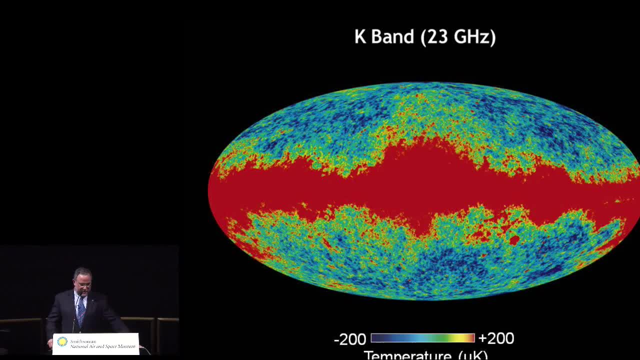 are all fluctuations from the early universe. Notice the temperature scale here: from minus to 200 millionths of a degree This is. these are very fine temperature measurements across the sky. So just to review, Penzias and Wilson discovered the radiation. 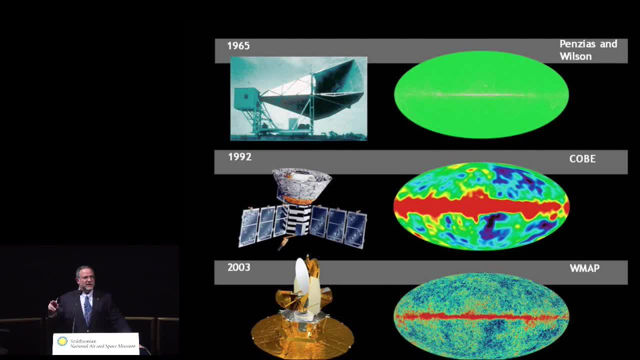 the microwave radiation. The COBE satellite discovered the tiny fluctuations in the temperature on top of this very uniform temperature sky, and WMAP now has brought that into fine focus and with much greater sensitivity. So we now have that map. Now we still have to get rid of the galaxy. 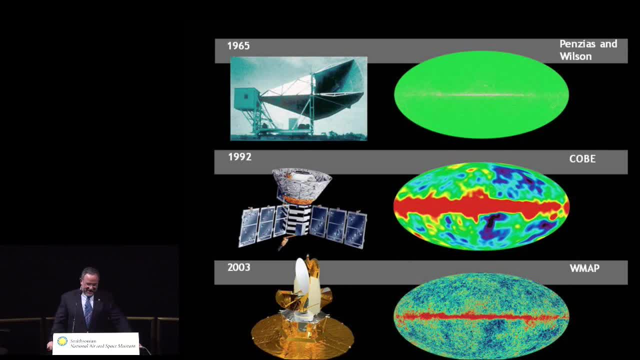 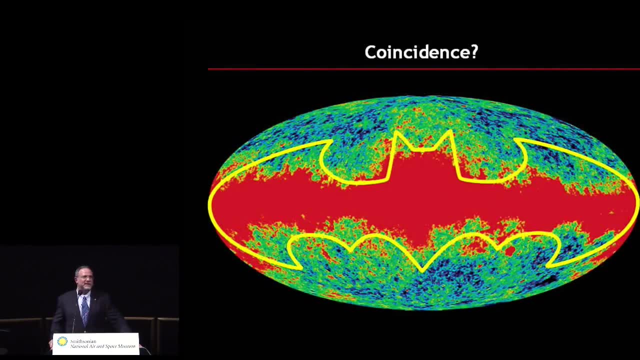 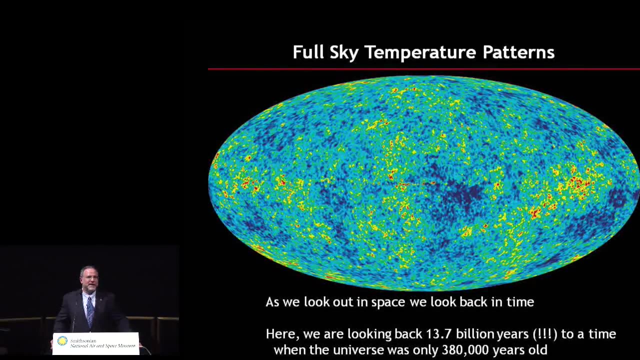 and we developed a very complex model of it here. So if we take away the galaxy, we're left with a map, a temperature map of the early universe. Remember, as we look out at distance, we look back in time. We can't help it. 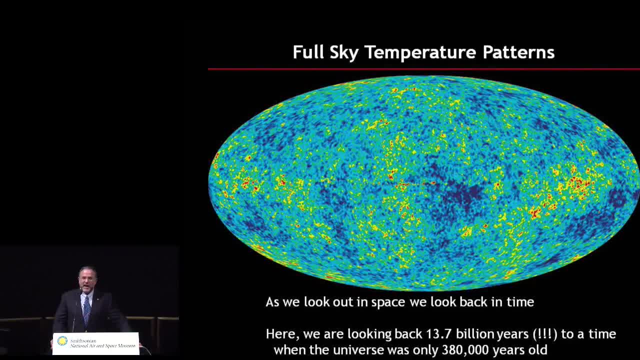 That's what happens because of the speed that light travels, And here we are now looking back 13.7 billion years. This light has been traveling across the universe all that time, just waiting for our satellite to detect it. This is a picture of when the universe 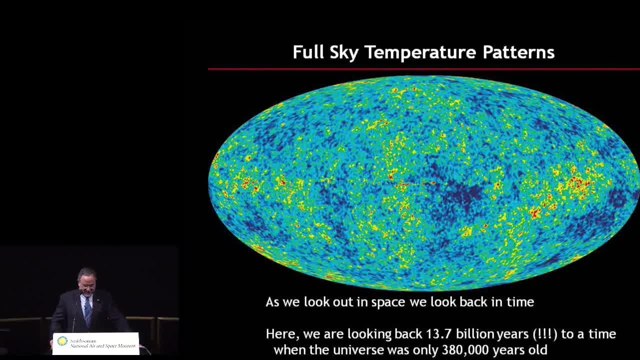 was only 380,000 years old in its infancy. So WMAP has provided us with a baby picture of the universe thanks to the time machine we have, and, just like is the case with the cake, we now have a picture of the universe in the making. 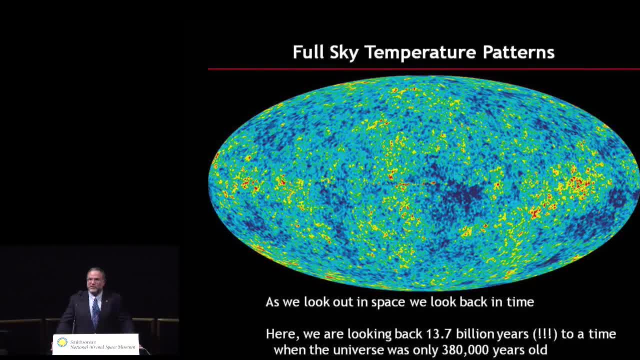 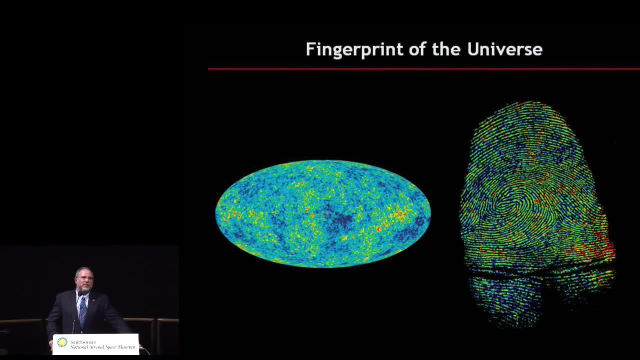 and this is what we're out to get, because we can learn a lot from this picture, as I'll show you. So what counts in this picture are the patterns of the temperature fluctuations, and think of patterns, maybe like a fingerprint. And the interesting thing is: 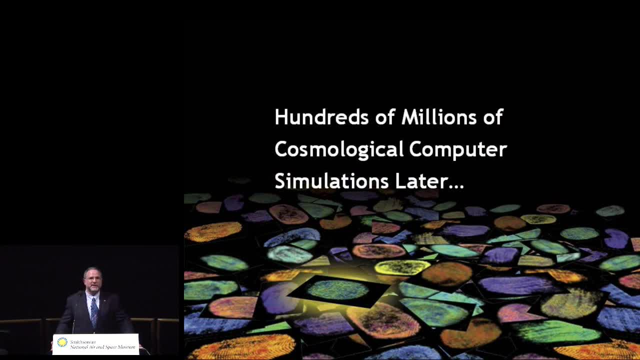 we actually understand the laws of physics that go into this, and so we make computer programs where we just tell it the ingredients and it tells us what the pattern should look like. You say so many of these atoms and this age and whatever you want to tell it. 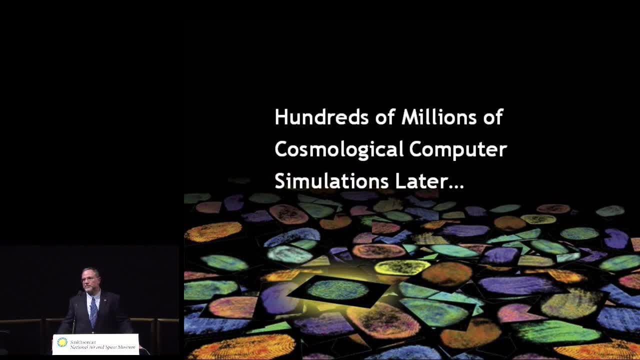 and it tells you what the picture should look like. So we run this computer program hundreds of millions of times, just varying the input ingredients, and it spits out all of these patterns that are possible universes and we sort through and we look for the one. 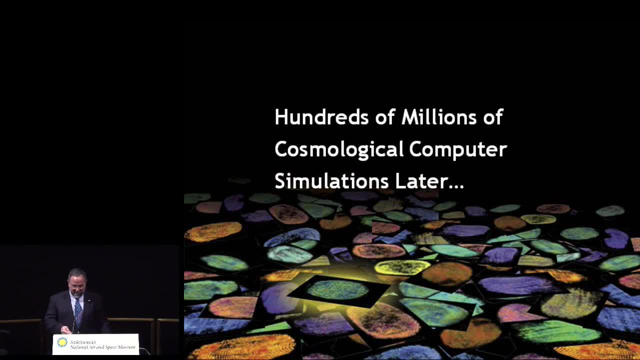 that matches our universe. And when we find it, then we know the ingredients of our universe because we know what we put into the computer program. And this is literally what we do. We've got the picture. we use our laws of physics to understand it. 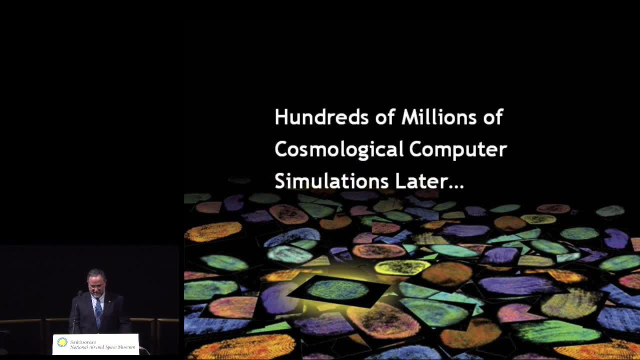 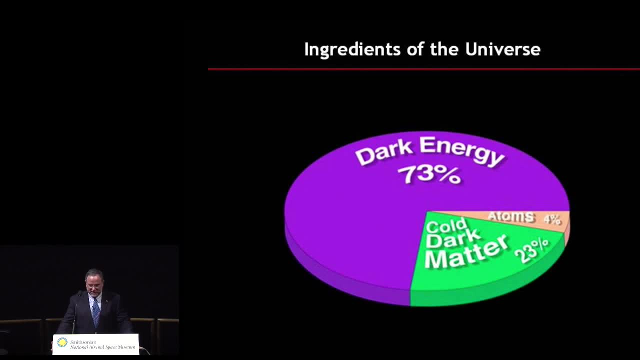 and we pick out the solution. And so, what's the solution? Well, here are the ingredients: 73% of something called dark energy, 23% of something called cold dark matter and 4% atoms. What is dark energy? 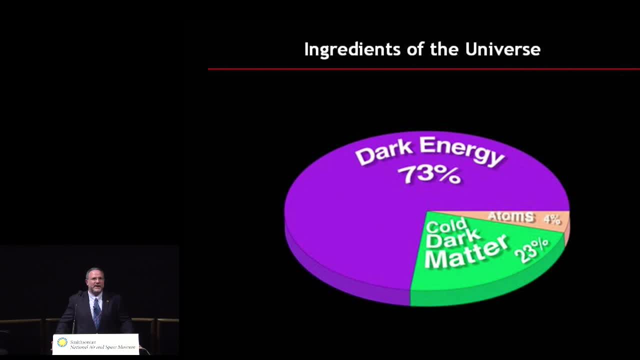 We don't know. Dark energy is some kind of anti-gravity and, if that sounds familiar to you, one of the top leading candidates for what it is is Einstein's old cosmological constant. Remember my greatest blunder? maybe most of the universe. 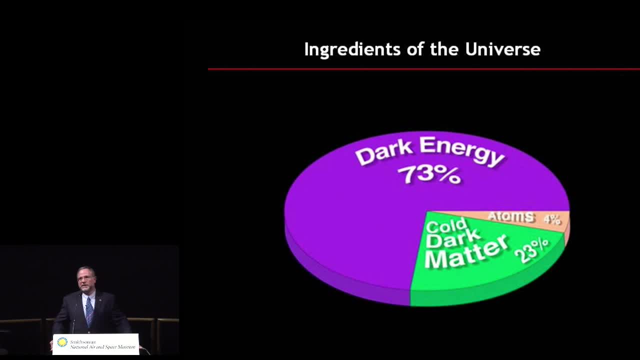 Cold dark matter. what's that? Well, we don't know, But I'll tell you what the words mean. It's kind of a secret code here. Cold means it moves slowly, It lumbers along, unlike the neutrinos you heard about. 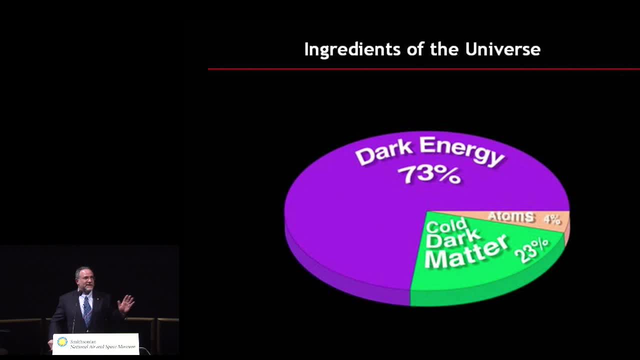 that go faster than light, Not This stuff. that's hot, This is cold, It lumbers. Dark means not just dark, but dark means it emits no light at all, None Zero. It doesn't absorb light, It doesn't scatter it. 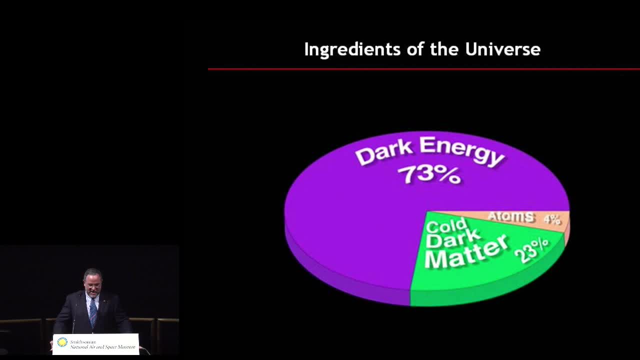 It doesn't know anything about light that's going through your body right now. It's 23% of the universe and there's far more of it This stuff Zwicky was talking about. Why is there so much more stuff in this cluster of galaxies? 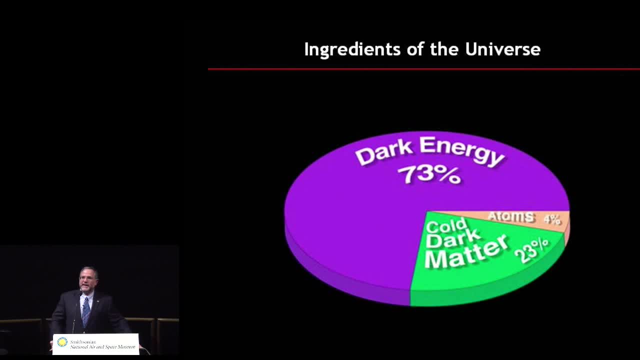 It's this cold, dark matter And only 4% atoms. All those years in high school chemistry for 4%. But it's what you're made of, It's what I'm made of, We are the 4% right. So it turned out a few years ago, 1998,. 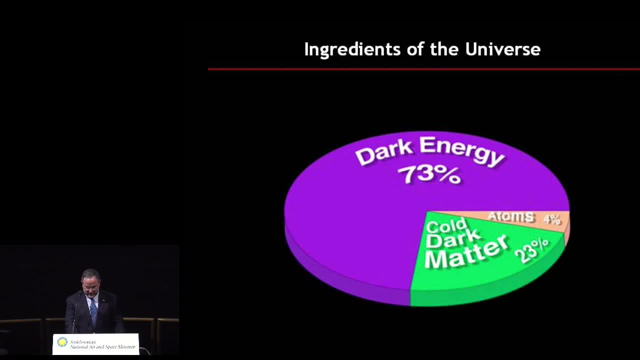 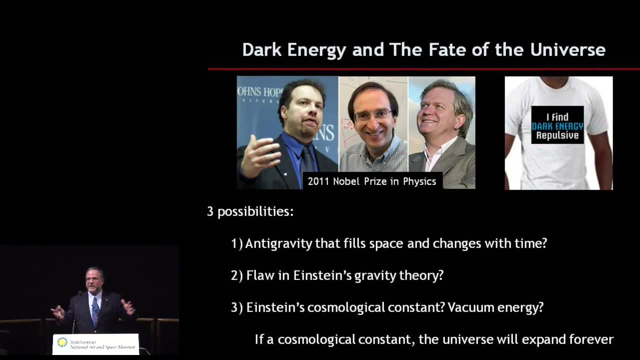 that a group of scientists measured the expansion of the universe and they were looking for how much it was slowing down, Because you think the universe is expanding, the gravity ought to pull back on it- And they were surprised that the expansion was speeding up, not slowing down. 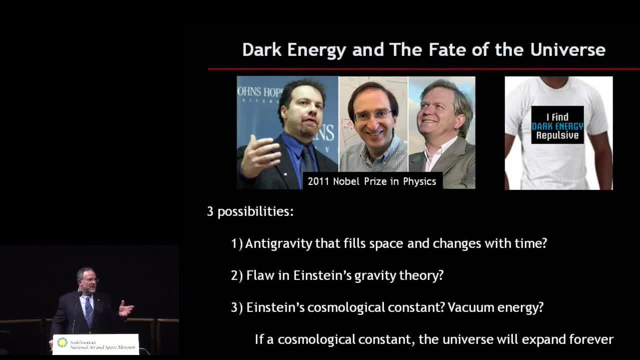 And this is really weird. I mean, if you took your keys and threw them up in the air, you expect them to slow down, Maybe even come back down again. This is like throwing your keys up in the air and having them go up faster and faster and faster. 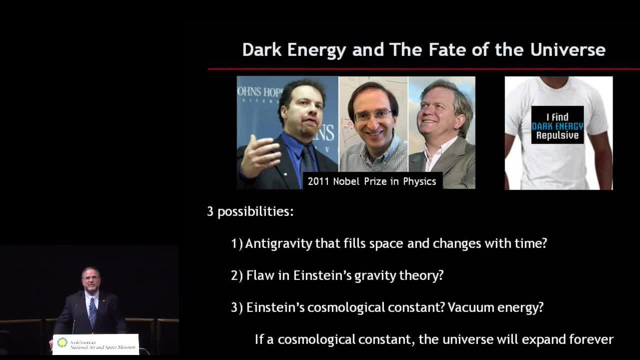 Really weird, right, But they discovered that this is what the universe is doing. Hubble measured that the universe is expanding and it's not slowing down. It's actually speeding up. It's expanding faster and faster all the time, And they won the 2011 Nobel Prize in Physics. 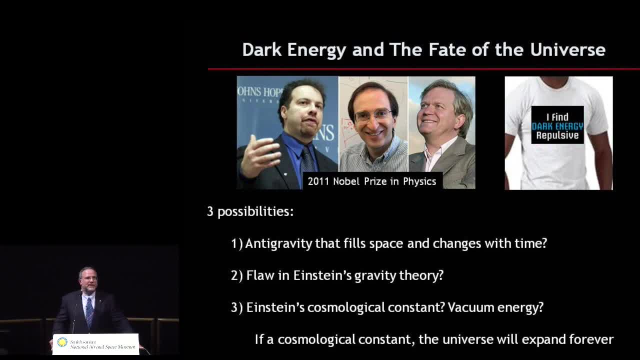 for this discovery. What they did not win the Nobel Prize in Physics for is explaining why it's happening, only for discovering that it is happening. So we believe that that big 73% of the universe that's dark energy is what's responsible for this. 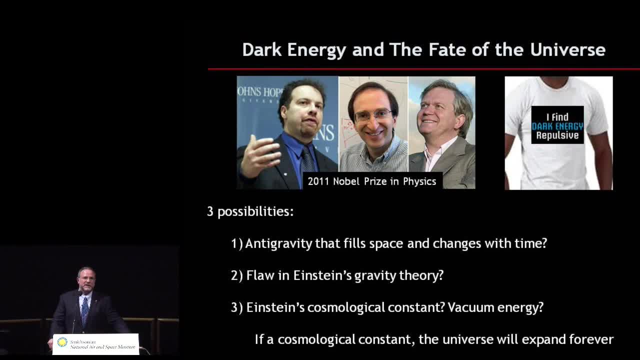 But there are three things or possibilities of what's going on and we don't know which is right. One possibility is that there's some kind of anti-gravity field that fills all of space and that it's evolving with time. A second possibility is that there's actually a flaw. 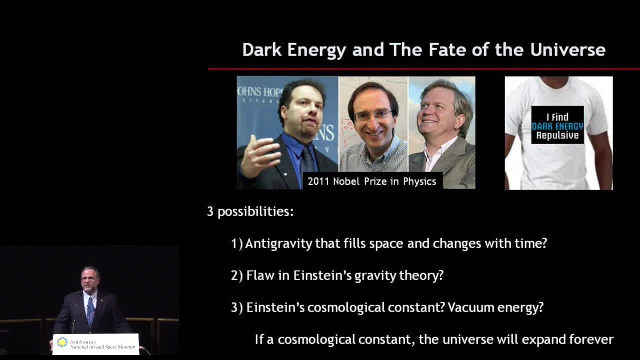 in Einstein's general relativity and his gravity theory. Now I told you all about testing it in the 1919 eclipse, and there have been many other tests of the theory too, and it's always passed with flying colors. But we are now applying it on the scale of the universe. 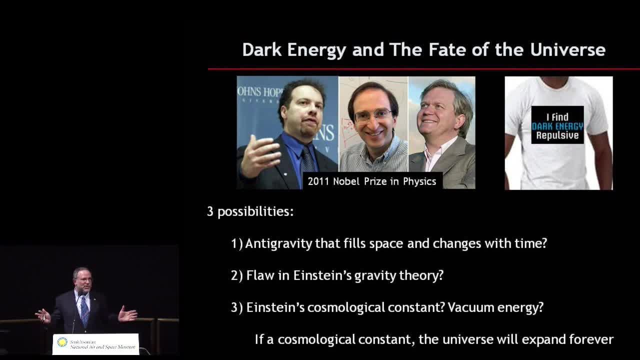 a scale at which it's never been tested, and maybe it's broken. Possibly, We don't know. The third possibility, and I would say currently the favorite- not that that matters, but the current favorite possibility- is that it is in fact Einstein's cosmological constant. 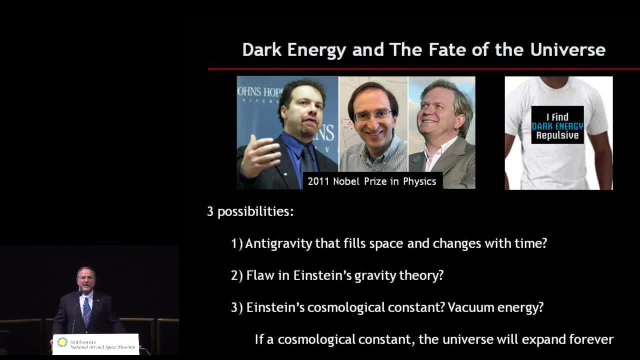 The twist here is Einstein just threw that in, as I described to you, but actually there's now some understanding of physics behind it, and that is to say, a topic called vacuum energy. What is vacuum energy? Well, if you go out into space and get a box of nothing, 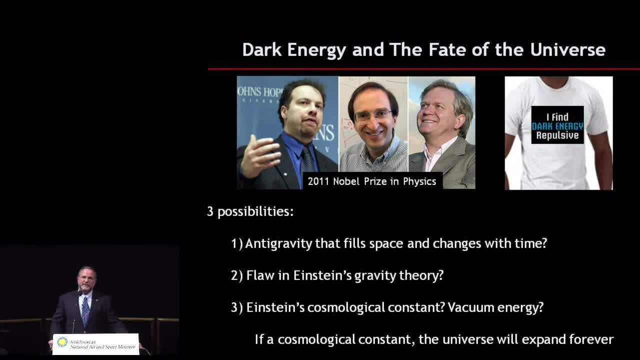 you might expect, it weighs nothing, but in physics that's not necessarily true. In fact, in physics what is true is that there's no such thing as nothing. If you have a vacuum in physics, you constantly have particles appearing in and out of the vacuum, out of nothingness. 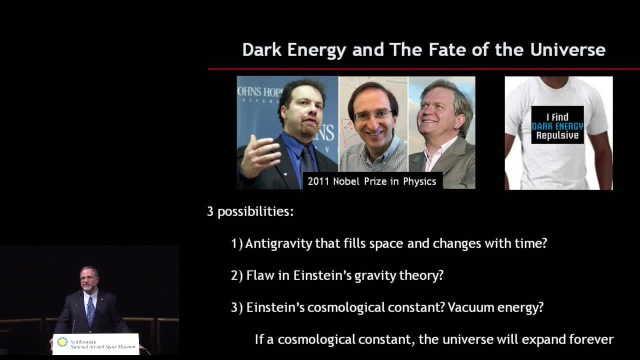 This is what the Heisenberg uncertainty principle says. It says that things can appear, disappear, appear disappear. These are called virtual particles. This is standard physics. The question is that if you have a box of nothing, how much does it weigh? 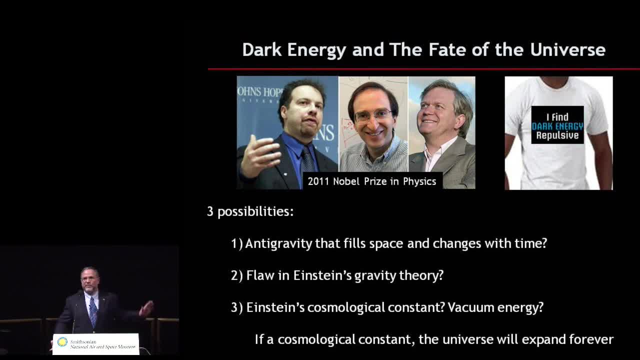 Now, physicists tried to estimate this a long time ago, before the accelerated expansion of the universe was discovered, and they came up with a ridiculous answer. If it was true, it would be some enormous amount. We wouldn't be here, So we know that they got that wrong. 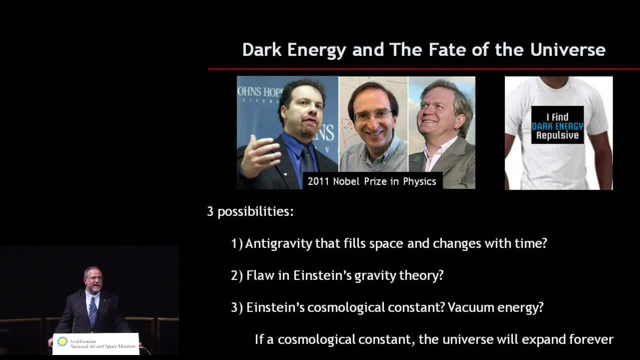 They had assumed for a long time that there must be some reason. it's exactly zero. but they didn't know why. and now we discover that the universe has this accelerated expansion. so now they're thinking: well, maybe it's not exactly zero. 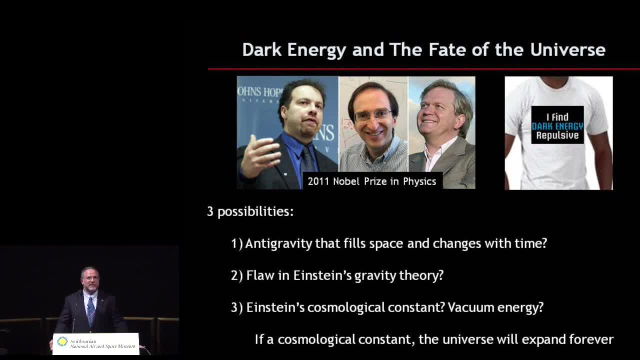 So there's some basis for thinking that there's something here, but right now we don't know for sure. What we do know is that if the dark energy is Einstein's cosmological constant and this vacuum energy, then the universe will expand forever. 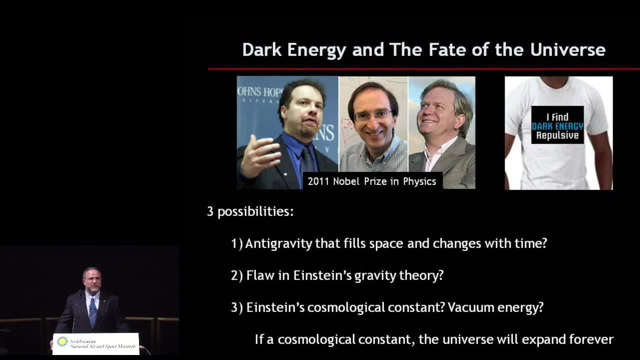 faster and faster and faster. That would be the fate of the universe, But since we don't know for a fact that that's what's going on, we can't really say what the fate of the universe is, which all goes to show that it's tough to make predictions. 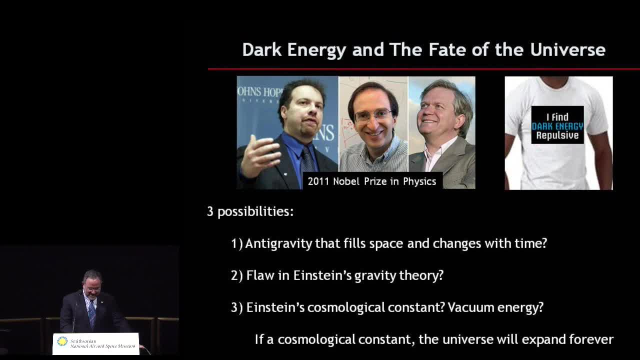 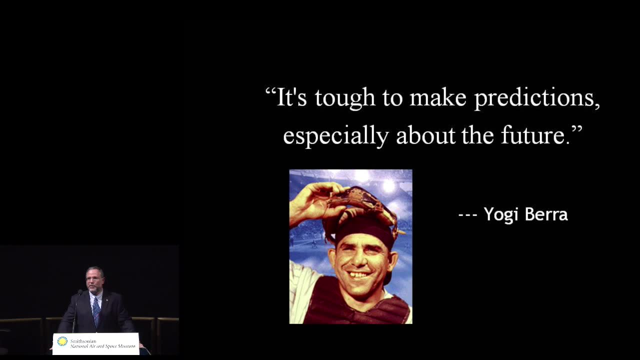 especially about the future. So what else came out of that picture, from WMAP, that pattern in the computer programs? One thing that came out is the age of the universe: 13.75 billion years, give or take 0.13 billion years. 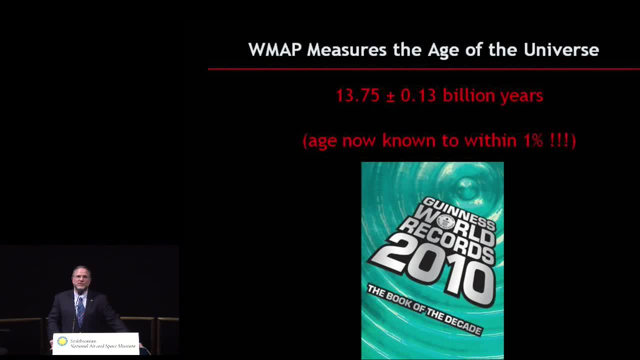 This is an age now known to within 1%. When I was in graduate school at MIT, I didn't know whether the age of the universe was 8 billion years or 22 billion years. Now we know it to 1%. This is more of the progress of our precision cosmology. 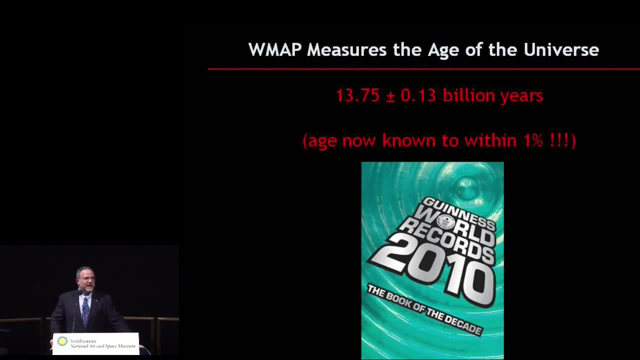 And if you don't believe it, check the Guinness Book of World Records. It has the most accurate measurement of the age of the universe. Credit: WMAP. WMAP also measures this shape of space, the curvature of space that we talked about. 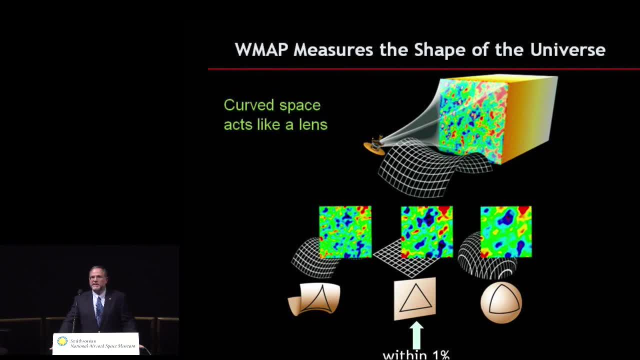 that Einstein introduced, And the reason for this is that curved space acts like a lens And we're observing across the universe to this sort of picture and this light is coming to us across space, And so, depending on how space is curved, 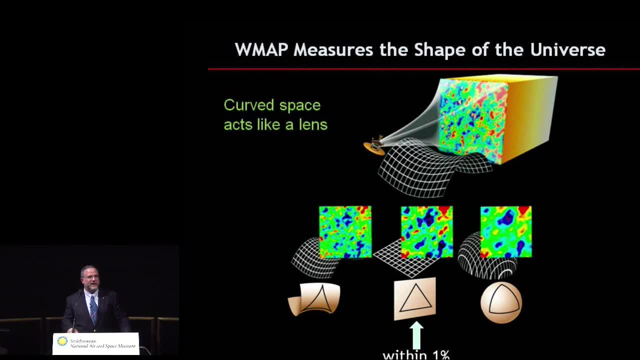 it can magnify the picture or it can demagnify it like a lens. And the question is: what is it doing? Well, the way to know whether space is curved, or one way to know, is to draw a triangle. You learned in high school, if you remember. 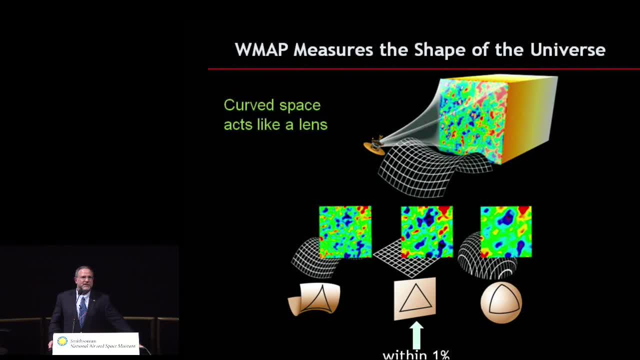 that if you add up the angles of a triangle, you get 180 degrees. But that's only true if you're in Euclidean, what we call flat space. If you're on the surface of a sphere, then the angles add up to more than 180 degrees. 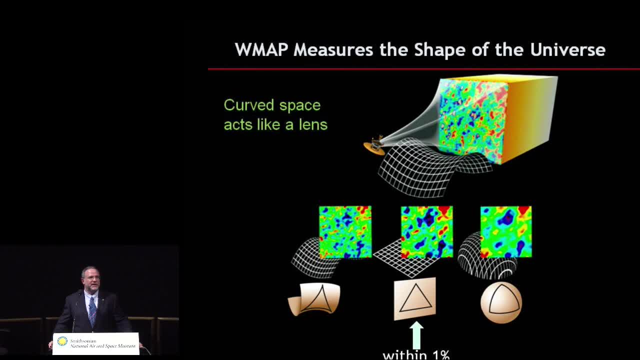 And if you're on the surface of a saddle, they add up to less than 180 degrees. So if we draw a triangle in space, then we can measure the angles and we can know what kind of curvature the space has. And in fact that's just what WMAP has done. 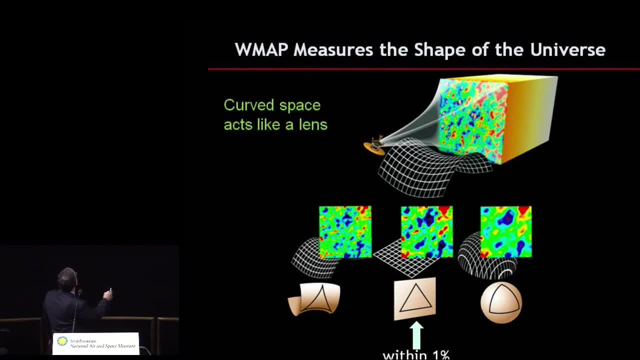 I'll show you the triangle Right, And so what WMAP says is that the curvature of space is as close as we can measure to this kind of Euclidean solution from high school geometry, And it's measured that it's that curvature within 1%. 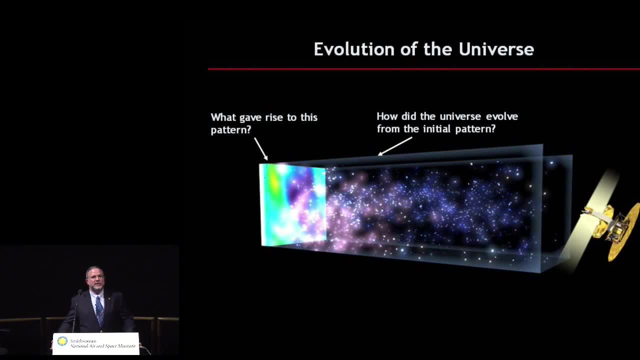 Now, up till now, I've been describing this pattern that we've been observing from the satellite and the light that's, and everything that's happened since that, and the light that's been traveling to us. But now I want to turn the whole conversation. 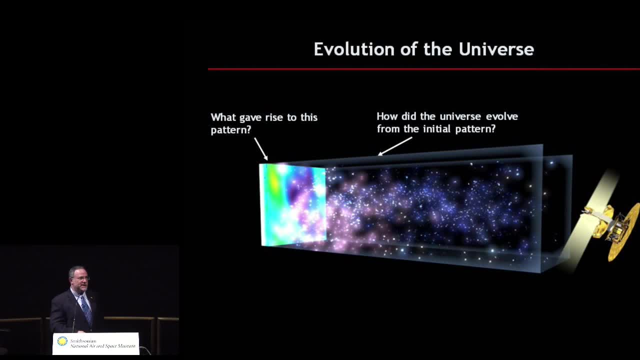 around the other way. to address the question I asked at the beginning of what happened at the beginning of the universe, Not only is this surface that we're looking at, where this light is coming from, the beginning product of everything that came after, it's also the end product of everything that came before. 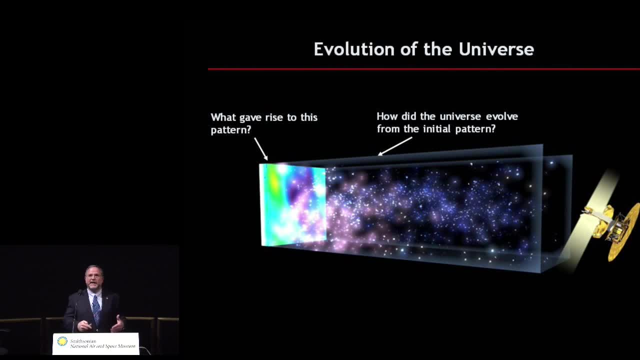 If we want to construct a theory of the early universe, it has to produce a picture like that, or it isn't right, And so we have a way now to measure what happened in the very early universe. So how did the universe begin? 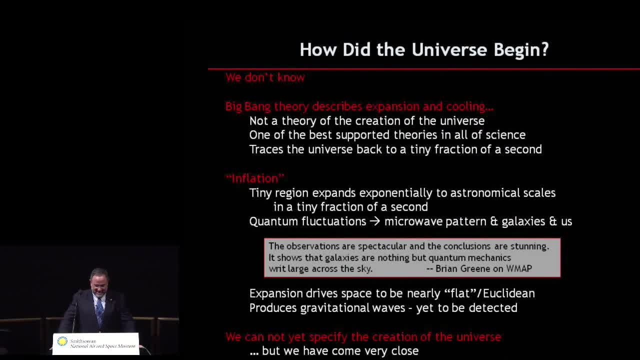 The answer is: we don't know. Um, But the Big Bang theory describes the expansion and cooling, but it is not, despite common wisdom, it is not a theory of the creation of the universe. Um, It is one of the best supported theories in all of science. 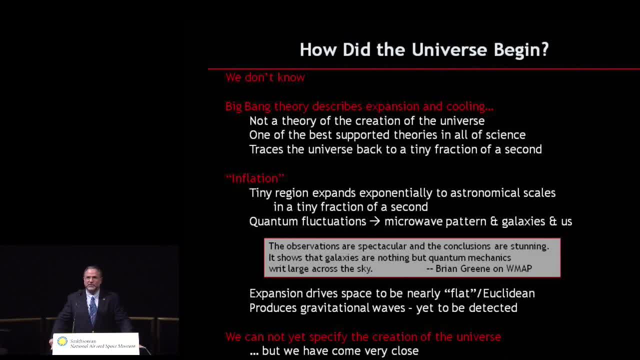 I've described that to you. I've described the predictions and the verifications. The universe has been expanding and cooling And we can use this to trace the universe back all the way to a tiny fraction of a second. But that's it. 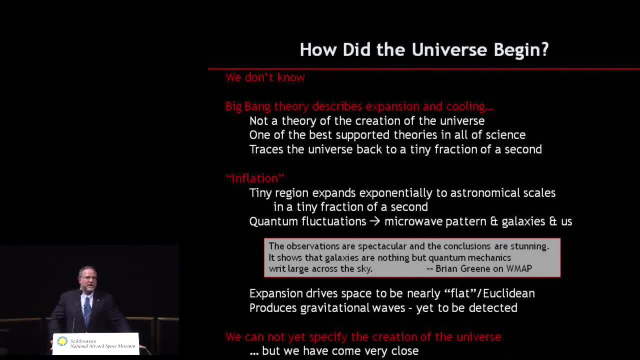 We have another theory called inflation. It is not as well supported as the Big Bang theory yet, And in fact it isn't even an individual theory, It's kind of a class of theories. But the idea is that you begin the universe with a very, very tiny region of space. 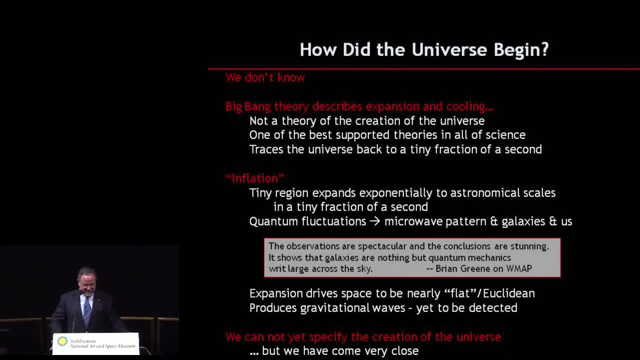 much smaller than a proton And it expands incredibly quickly, exponentially to astronomical scales in a fraction of a second. Sounds crazy, but this actually works in physics And um The quantum fluctuations that begin that it that you have in the universe. 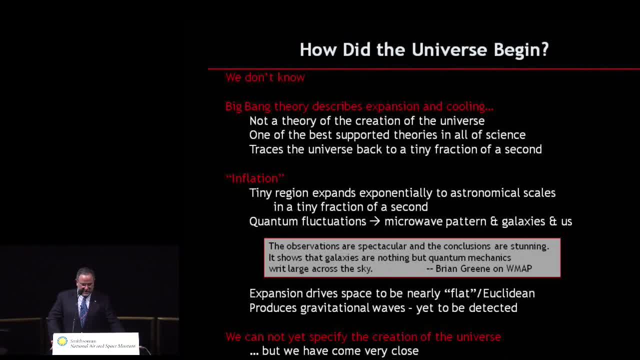 are converted by this process to ordinary fluctuations And in this picture, the microwave picture I showed you, all of these patterns are a result of this and they're all from initial quantum fluctuations of a universe that was spontaneously created from nothing And everything that came after. 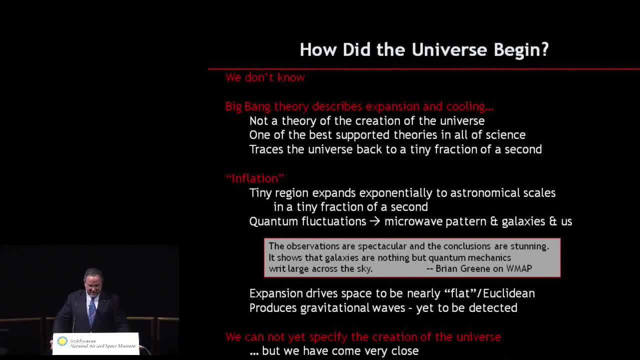 was a result of these quantum fluctuations. I particularly like a quote from Brian Greene when he was commenting on one of our WMAP results. I think it's quite poetic. He said: the observations are spectacular and the conclusions are stunning. It shows that galaxies 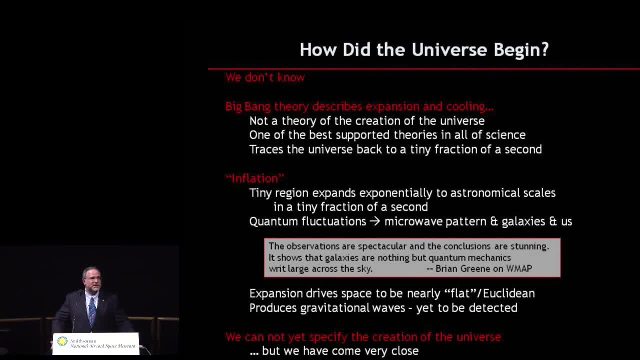 are nothing but quantum mechanics writ large across the sky. I think that's really a very nice picture to have of the galaxies. One question we've had. I showed you that we've measured that space is very close to this Euclidean flat space. 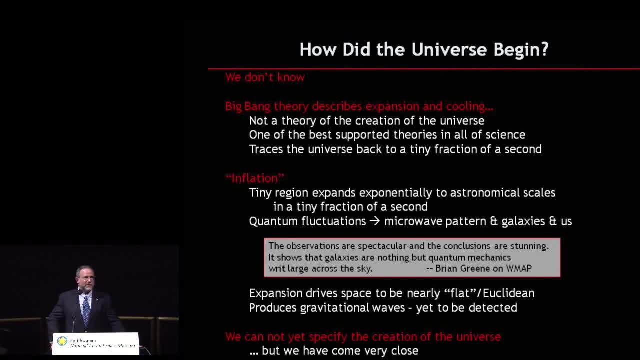 This is a very unexpected result from the Big Bang theory. However, this inflation theory explains the mystery And it's easy to explain why The Earth is curved, but it looks to us flat because it's so big If you start with any curvature. 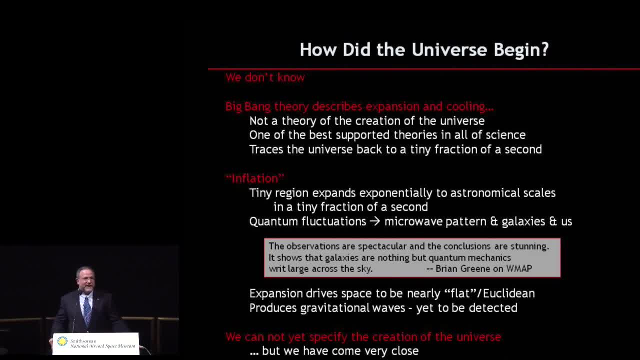 and you take the size of the thing and blow it up enormously, it's going to look flat to you no matter what, And inflation does exactly that. No matter what curvature we begin with, the inflation drives the universe to be so big that there's only a prediction of inflation. 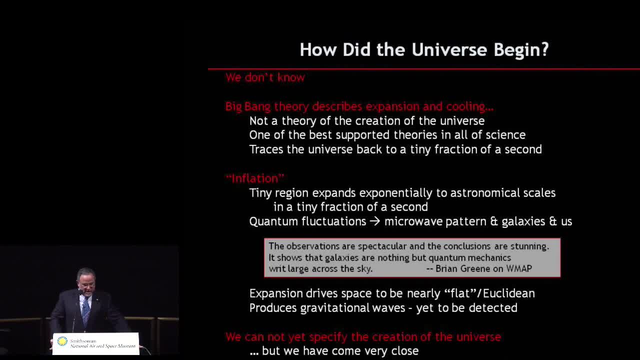 that is being verified by the measurements. There's a lot of other predictions of inflation theory that we have in fact verified with WMAP and with other experiments. Prediction after prediction is looking good so far, And even more than that. I mentioned that inflation. 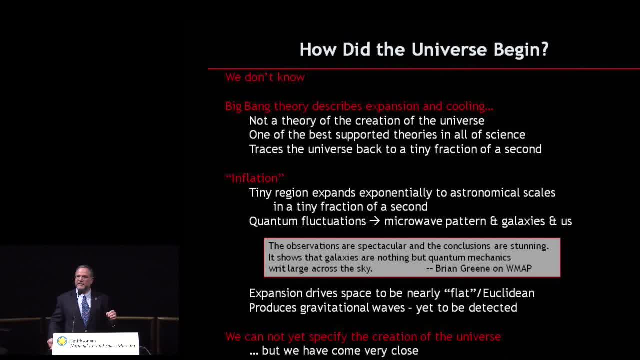 is not a specific theory but a whole class of theories. We have now been ruling out specific versions of the inflation theory. to emphasize what this means, We are using our observations to say what did and didn't happen, or what didn't happen in the first trillionth of a trillionth. 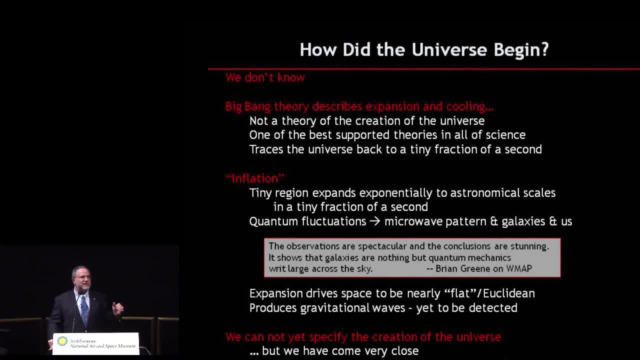 of a second of the universe. This is amazing. This is amazing that we humans have the capability of doing this, and it's largely thanks to this light that's coming to us, this microwave light that carries so much information with it that we are ruling out versions of inflation. 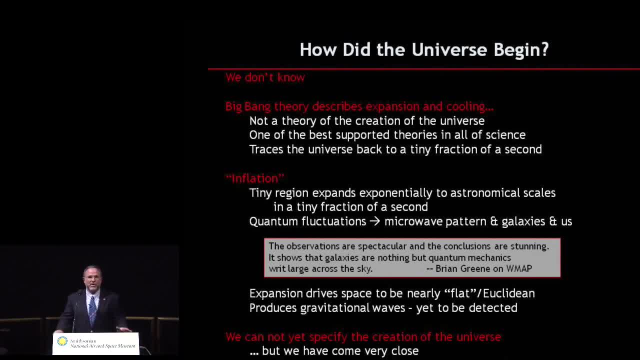 theory after theory after theory, with these measurements, which are still very workable, There is a prediction made that has not yet been verified, and that is that, at least in the simplest versions of inflation, gravitational waves are generated, and these gravitational waves should also fill the universe. 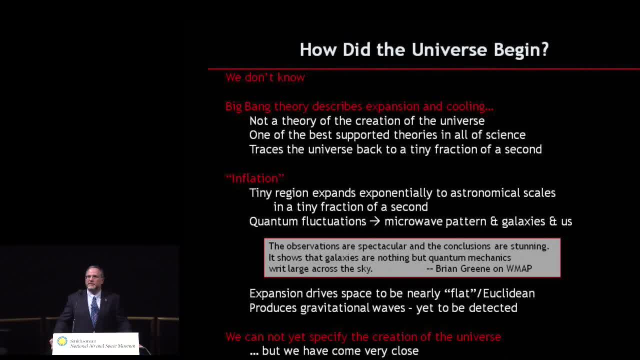 The trouble is that we've never detected gravitational waves of any kind at all, ever. We're working on it- not me personally but a lot of people- and we hope to do that, but so far it's turning out to be hard to detect. 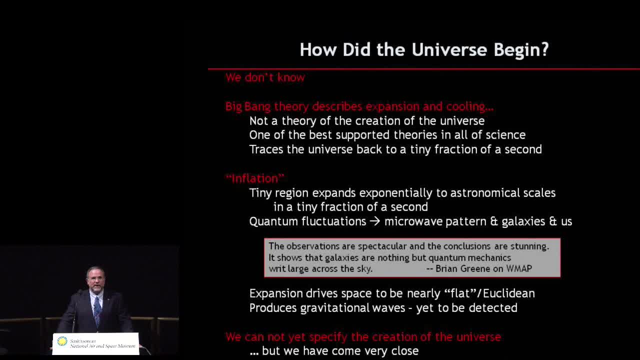 and I think the ones from the early universe will be even harder to detect. However, we have a little gift, which is that the gravitational waves create a certain polarization pattern of the same microwave light we're looking at. So if we can measure and look, 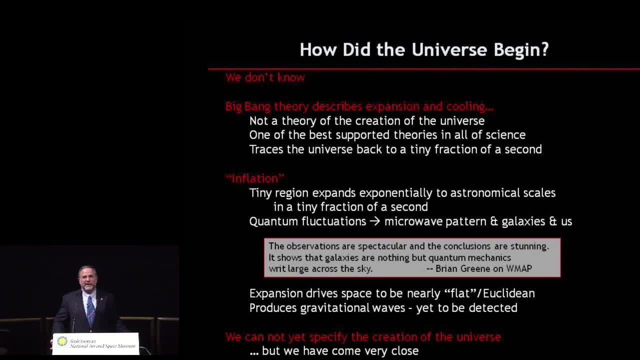 for that polarization pattern. I think, if we see what's predicted by the inflation theories, that that would be smoking gun evidence that inflation is indeed what happened, and the nature of the polarization pattern can tell us what kind of inflation. So to me that's one of the most important measurements. 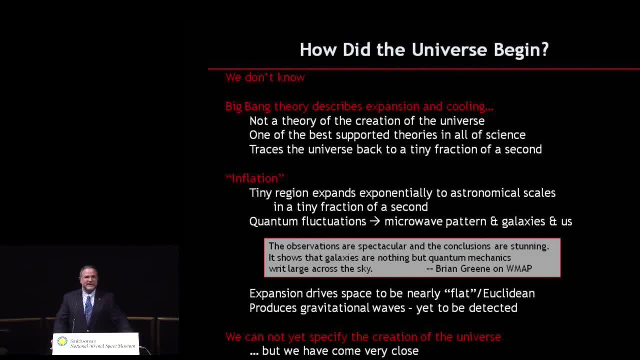 to make of the future. So we cannot yet specify what happened at the creation of the universe, but we have come a very long way. I hope you can see that that the measurements over the decades, and especially recent measurements, have made a lot of progress and new instruments and measurements. 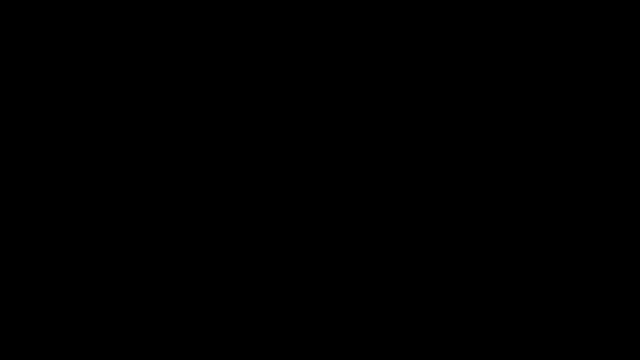 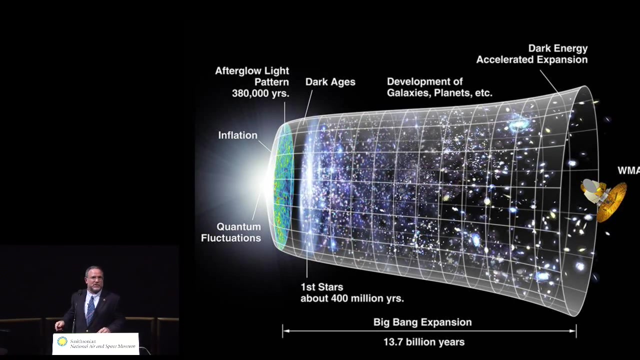 are on the way. Let me summarize the story that I've told you: producing fluctuations. because the fluctuations are so tiny, there are not yet any stars or galaxies. There hasn't been time for gravity to pull things together yet, So there's a period of time. 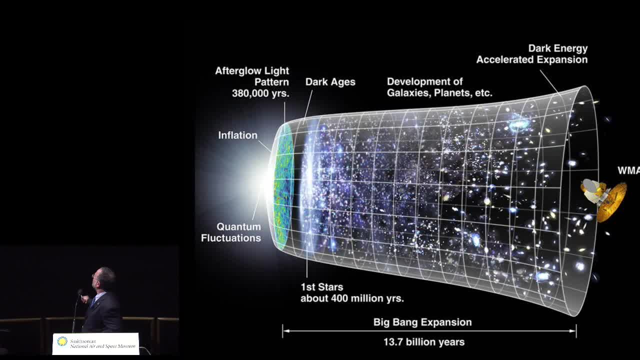 called the dark ages, because there are no stars glowing until there's enough gravity to pull them together and form the first stars, at an age of about 300 million years. And then we see the big bang, expansion, the universe is expanding while clusters of galaxies and galaxies 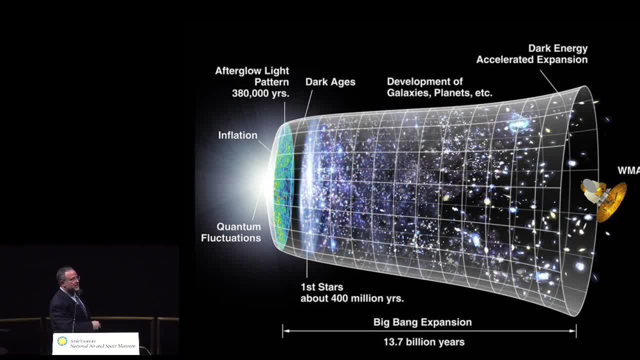 have accelerated expansion. we see this kind of turn up in the expansion rate. So think of this as a graph of how the universe is growing Very quickly in inflation: this big bang expansion and then this recent accelerated expansion from we don't know, but possibly the cosmological constant. 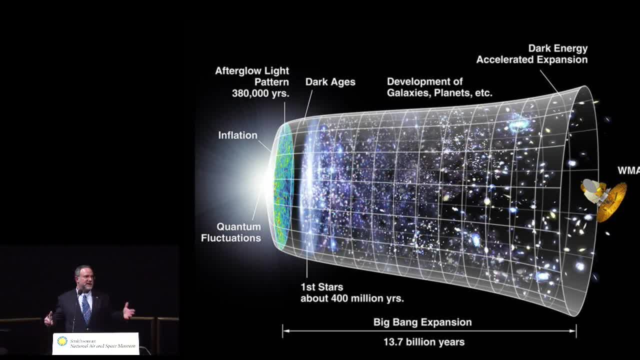 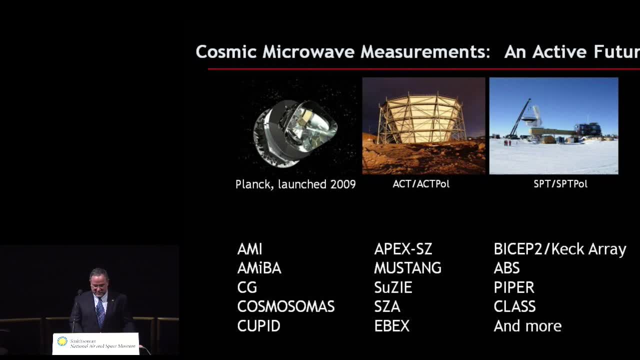 So, as I mentioned, there's lots of experiments, lots of acronyms up here. I just want to give you a sense that there's a lot of effort still going on. There's a lot more to do. We have the Planck satellite that was launched from the European Space Agency. 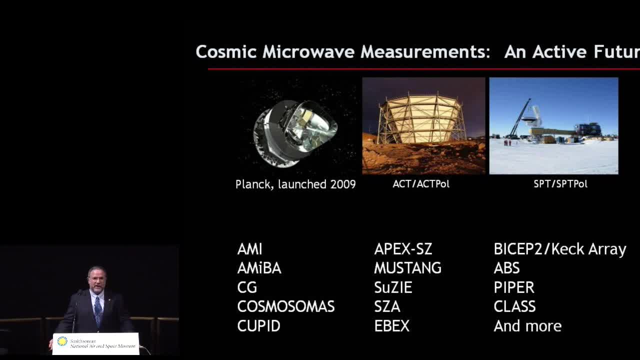 in 2009.. They'll be reporting on results early next year. We have observatories high in the Chilean Andes. we have observatories at the South Pole- All of these things aimed at measuring this precious cosmic microwave radiation. I'm leading one of these experiments myself. 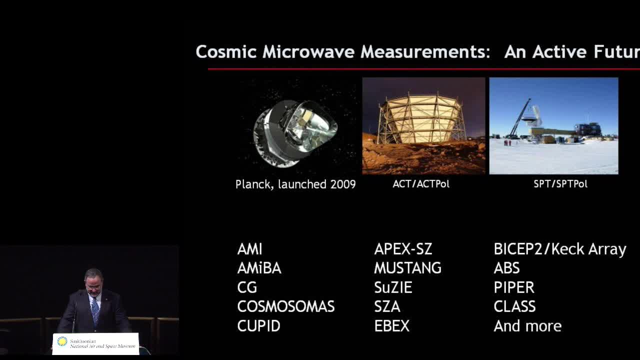 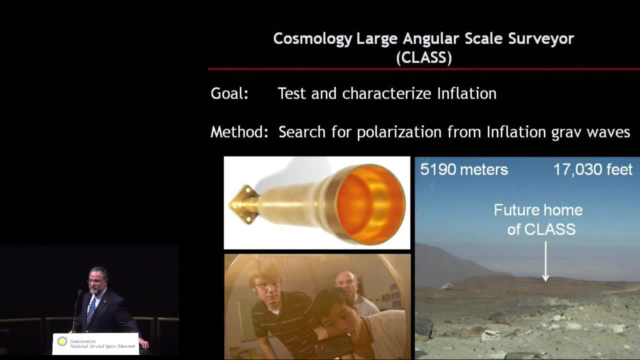 called CLASS the Cosmology Large Angular Scale Surveyor. as is the history of many of these measurements, We're going to develop new technologies to make these very, very sensitive measurements more sensitive. all the time, My graduate students working on a wire grid mesh working on how to collect the radiation best. and then we're going to place this high in the Chilean Andes, in the Atacama Desert, at an altitude of 17,000 feet, which, in case you're wondering, is only half the oxygen at the sea level, so it's hard to breathe there. 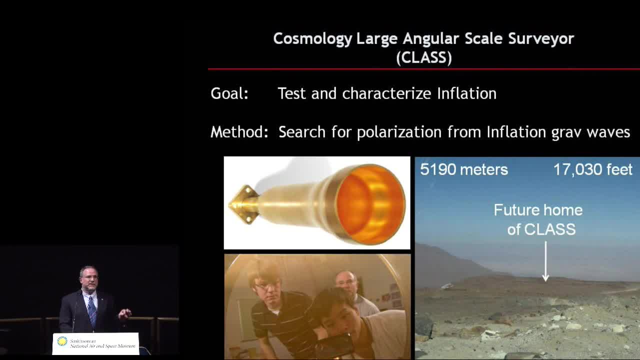 but it's the next best thing to being in space and we're going to try to look for this signal in gravitational waves in the polarization pattern. So let me close now. We are here. you and I are here because of the tiny fluctuations that were born in the first moments of the universe. 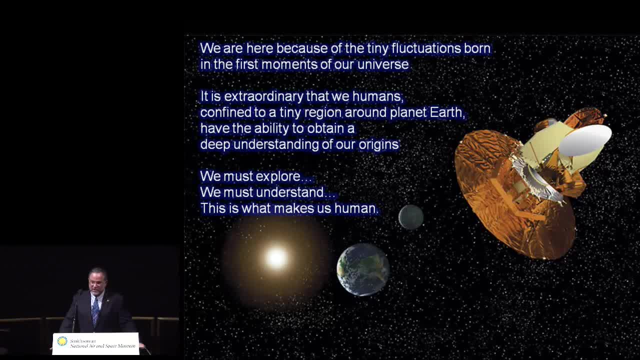 It is extraordinary that we humans, confined to a tiny region around planet Earth, have the ability to obtain a deep understanding of our origins. We must explore, We must understand. This, I believe, is what makes us human. Thank you, Thank you, All right. 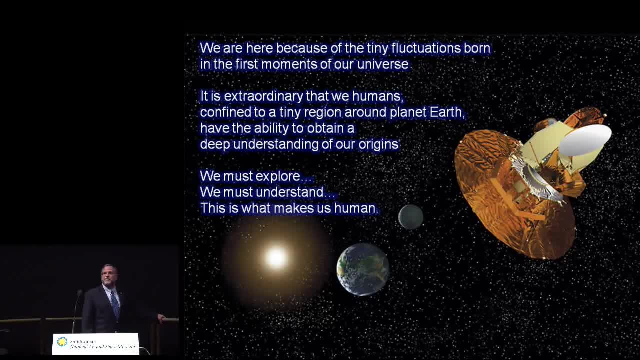 Dr Bennett has kindly agreed to field his own questions, so have at it Right there. Yes, Many of the ones on the list that I showed you. in the frontier area for many, many years, as I described, we try to detect the temperature. 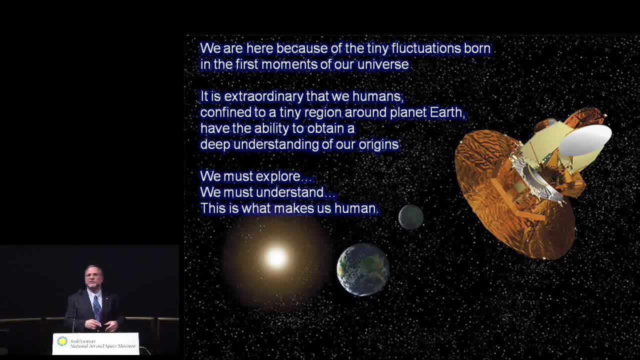 We try to detect it at all, as Penzias and Wilson did Try to detect these fluctuations, Try to characterize these fluctuations, And now much of the scientific community that works in this field is turning to the polarization as a way of doing this. So there's a few experiments trying to do that, And it's important that there are, because every experiment has its flaws and we're all using different approaches, and that's good. We're all using what doesn't work and we have a really good attempt at it. 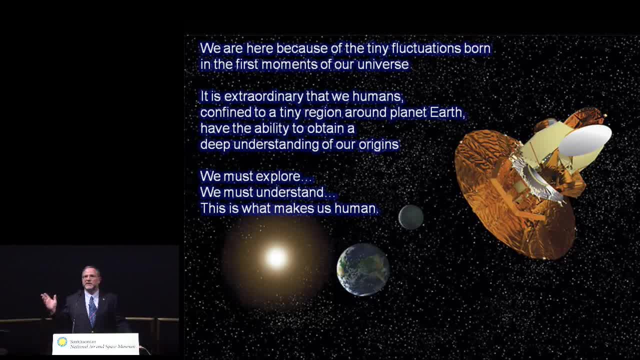 But I think there's something like six or something of those doing that. Do you have any questions? Sorry, I'll take them and then you Let me answer The gravity waves as a whole. there's an NSF funded project called LIGO on the ground. 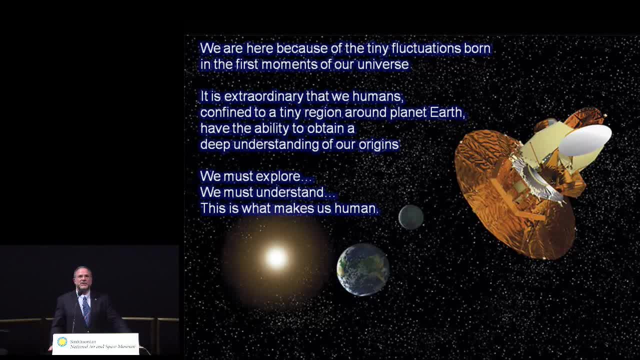 looking for gravitational waves. They're making progress all the time in their sensitivity. It's a very difficult problem, but I am hopeful that they will actually get there. They're getting close to the level where they should be able to detect gravitational waves. There will be a little time yet. 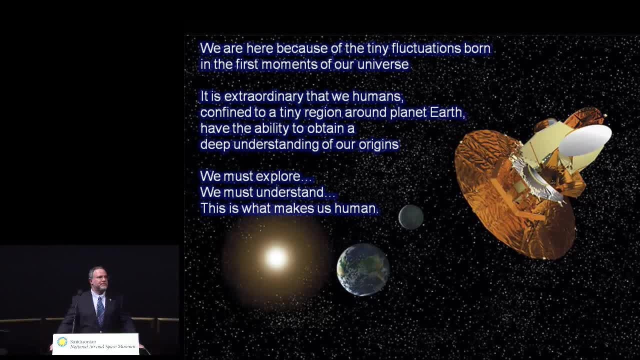 but I think they're going to get there. Question here: This is pure serendipity. Have you noticed that the shape of the detector you showed on almost the last slide is almost exactly the same as the schematic of the universe? Yes, 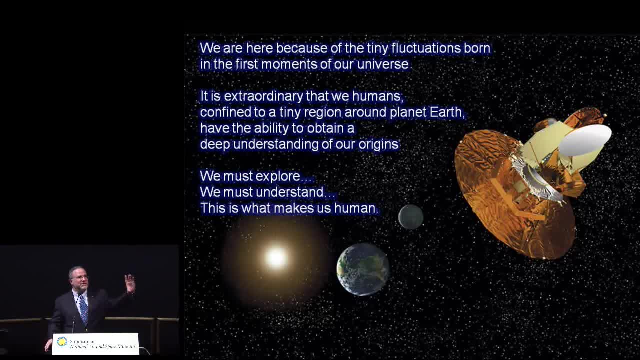 It was an observation that I hadn't thought about before- which is the shape of the technology I showed that collects the radiation and guides it down to our detector is sort of the same shape as the curve of the expansion of the universe. I'm going to remember that. 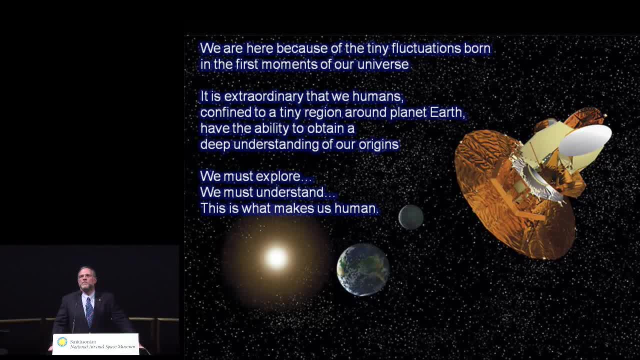 Up there? yes, Where are your satellites located Around the Earth, or do you use them around the planet? The COBE satellite that I worked on was on the Earth, but we had too many effects on the satellite from that kind of an orbit that we didn't think that we could handle. 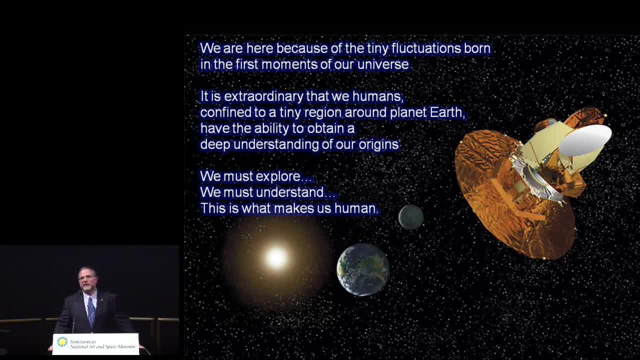 that with WMAP. So we sent WMAP out to the second Lagrange point. It was actually the first satellite to have that L2, to have that as its permanent observing station. For those of you that don't know, you have the Sun and you have the Earth. and about 1% farther than the Earth is where the second Lagrange point is right behind the Earth, going around the Sun, and that removed a lot of the effects of being in a near Earth environment. So that was a good observing place to be. 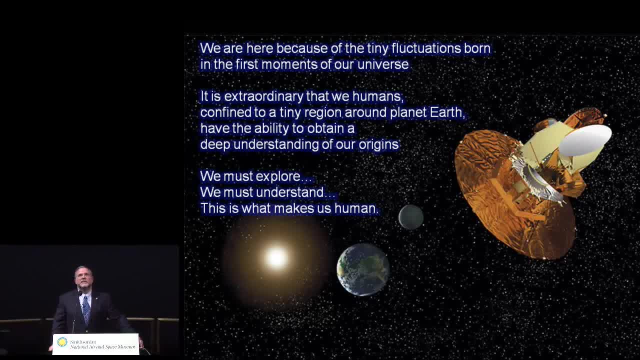 The European Planck satellite is there now as well, In the back back row? I will try, but I don't know. So the question is: what do I mean by transitions? So if you look at, for example, a hydrogen atom, it has certain. 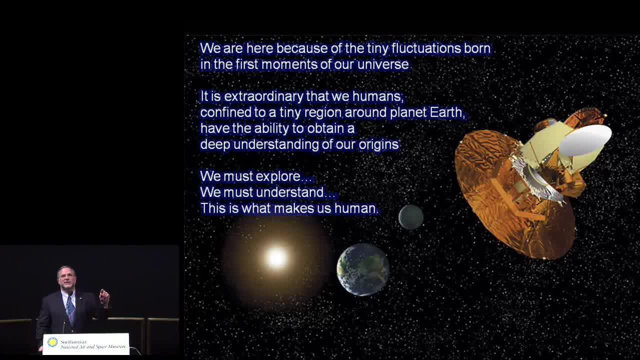 quantum transitions, and this is to say you get certain colors out of a hydrogen atom, not a whole continuum, but certain discrete colors out of it. This was noticed early in the 1900s, or at least explained early in the 1900s, in terms of a 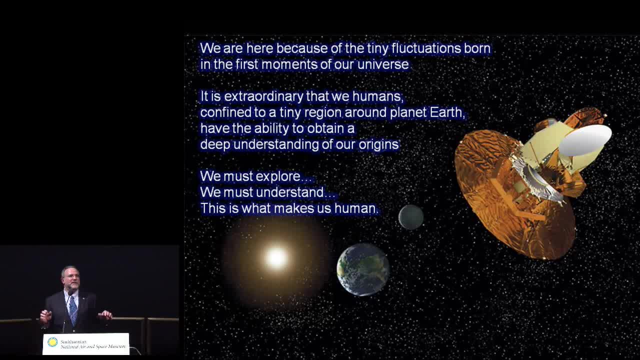 probabilistic way of physics, which is a big break from physics being very deterministic, and in fact, there is a lot of nature that deals in quanta of energy, and quantum mechanics is the whole field that describes this. so this is a good opportunity for me to say that we have 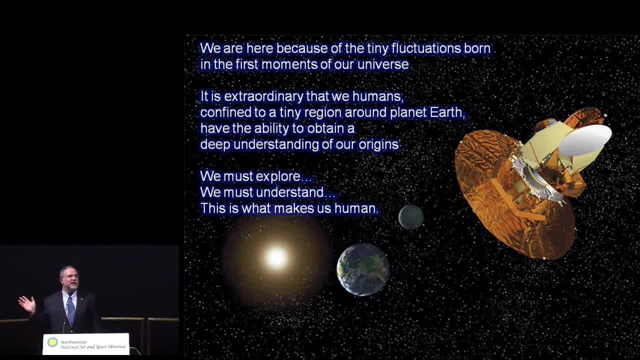 two great theories of 20th century physics. we have Einstein's gravity theory, the general theory of relativity, and we have quantum mechanics, which, by the way, Einstein wasn't very pleased about. I don't know if you remember the quote from Einstein: God does not play dice. 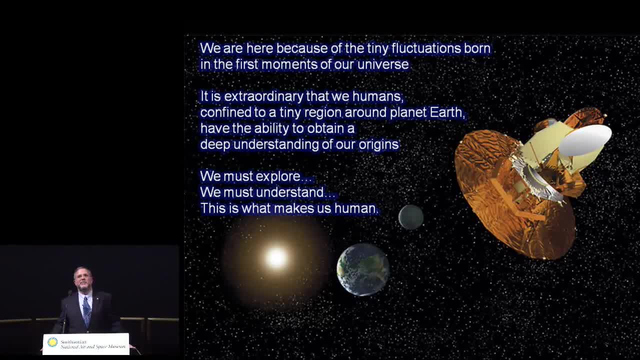 this was the idea that things aren't random, but actually things are random in many ways. but the thing that's very important here, the important point I want to make, is that these are our two great theories of 20th century physics, but they are incompatible with each other. 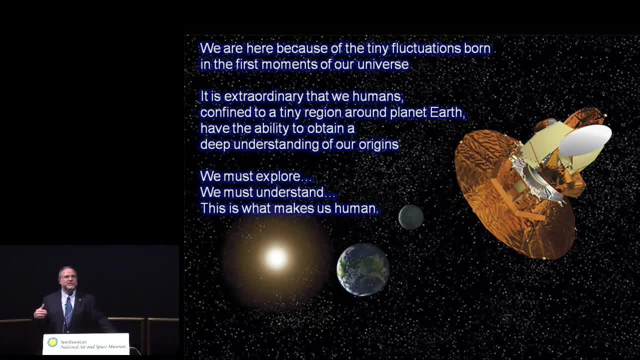 they do not work together and so something is wrong. and one of the reasons I'm so very interested both in the dark energy question and in the question about the beginning of the universe is, I believe, that these are the two places where you need to use in the inflation. it's very direct. 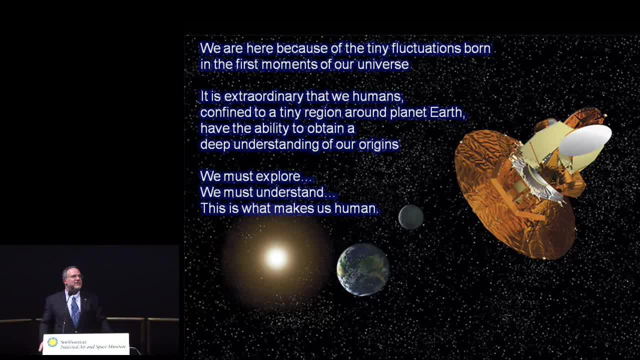 you start with quantum fluctuations and you end up with large scale gravity, so you're actually joining these two theories together, or you need to. clearly we need a quantum theory of gravity. we don't have one. there's a lot of people working on one. I hope somebody figures one out. 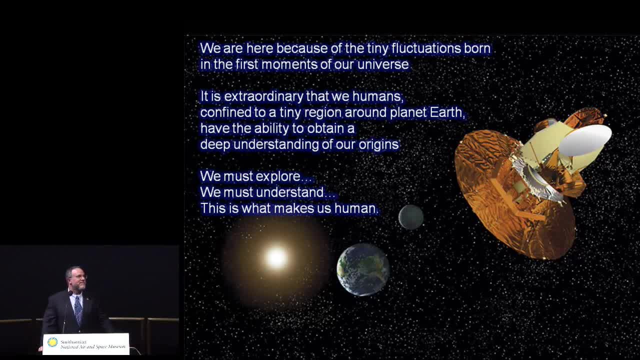 it won't be me, but I'd love to use it. there's a question right up here in front of you. I think there is a difference between the two, maybe trying to think of a simple way to describe it. but the one thing I didn't mention. 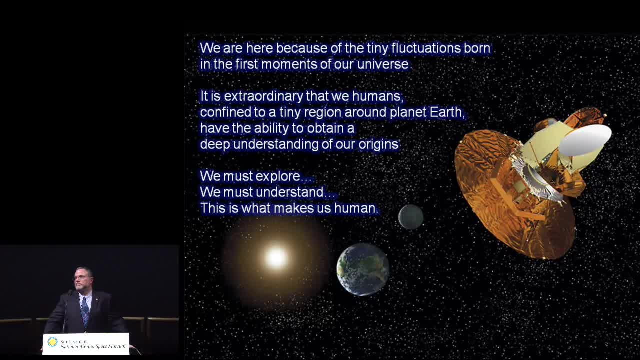 is that matter that is bound together, like your body or the earth, don't participate in the expansion. the only things that expand are things that are not bound together. so the universe on average has this very low density distribution and the matter, in a sense, is not moving, but the expansion. 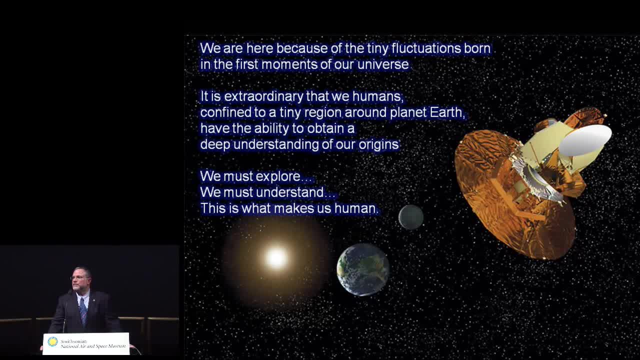 is still happening. so I think that they're fundamentally different things, but it's an interesting question. I think a little bit about maybe a better way to explain that, but not all things that have already condensed and combined like you're talking about. if matter falling together actually doesn't participate in the expansion. 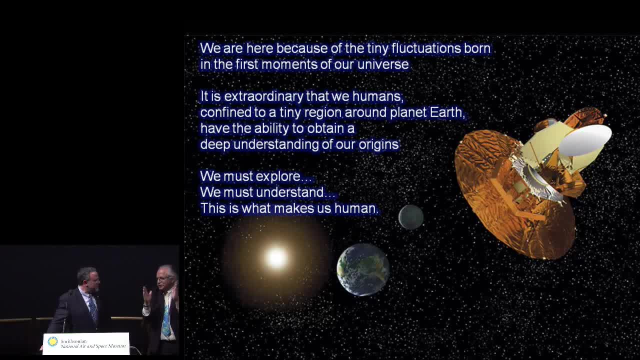 the image that you had of the grid expanding, but not the stars. yeah, that's, let's see. if you go back to Einstein's theory and you actually solve it for the universe, like Einstein did or Alexander Friedman did even better- you solve the equation. what you get is that the space itself. 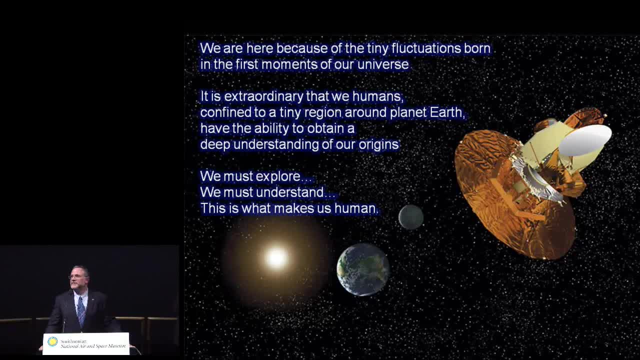 is expanding, and that's true even in a universe where there is no material. so, yeah, right in front of him, and then in front of the blue shirt and then the white shirt. I didn't quite hear, is it CERN? oh, CERN, okay. so the question is: 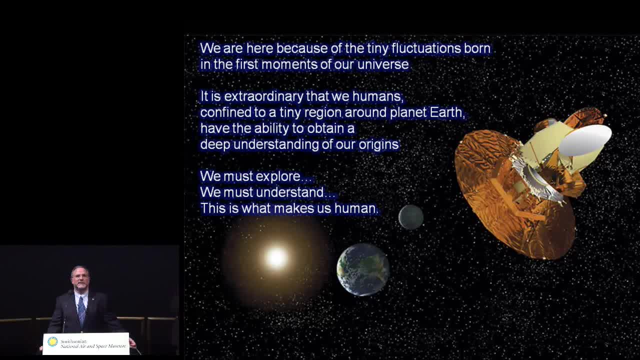 we have the Large Hadron Collider, the LHC, in CERN in Switzerland. it's a very important particle physics accelerator, and what does it bring to this topic it brings? my offhand reaction is two things. one is it brings, we hope, a better understanding of physics, and that helps all together. 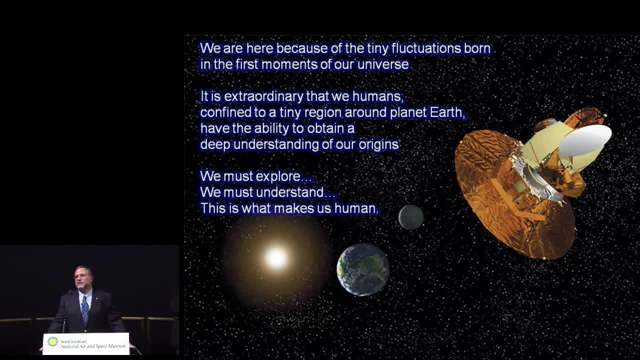 a little more specifically. I mentioned the cold, dark matter. I mentioned that we know what the properties are. the properties are a matter that doesn't interact with light and that it goes slowly cold. but we don't know what the particle is and it's quite possible that. 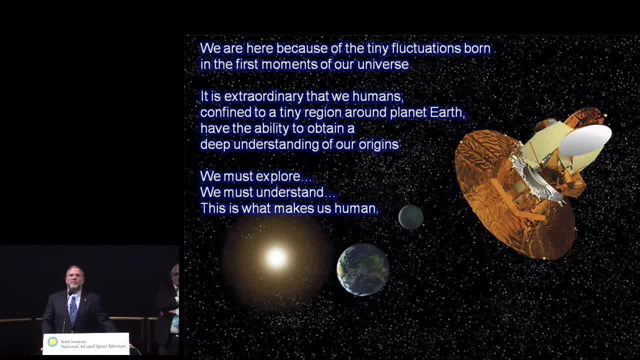 from what we learned at CERN at the Large Hadron Collider, that we will actually be able. it will play a role in identifying what the particle is. in addition to CERN, there are experiments around the globe actually trying to directly detect this dark matter. they fill old. 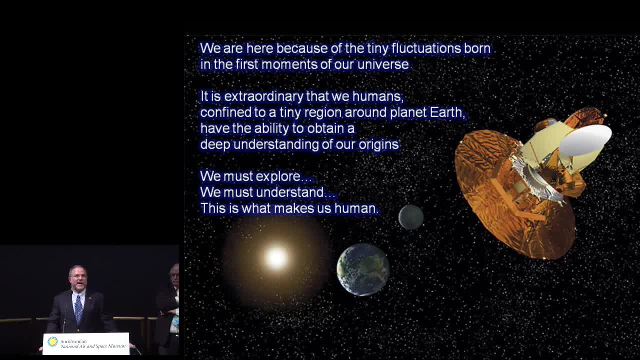 mines with detectors and try to stop the stuff and look at it, and so I think, between what we learned from the Large Hadron Collider and these what we call direct detection experiments, I'm actually pretty hopeful that we're going to learn what the dark matter is within the next few years. 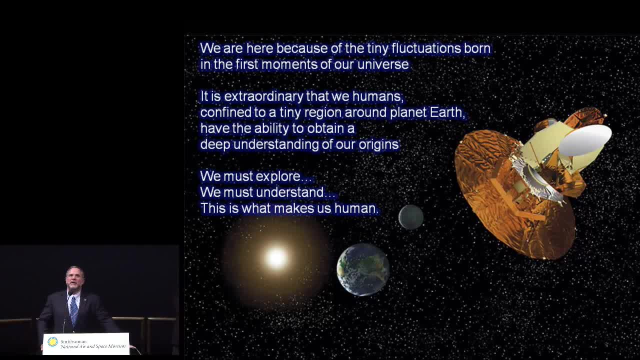 yeah. so the question is: in unifying the gravity theory, the general theory of relativity, with quantum theory, where does things like string theory and m theory and things like that fit in? and those are exactly the kinds of things that need to be worked on. those are exactly aimed at a deeper understanding. 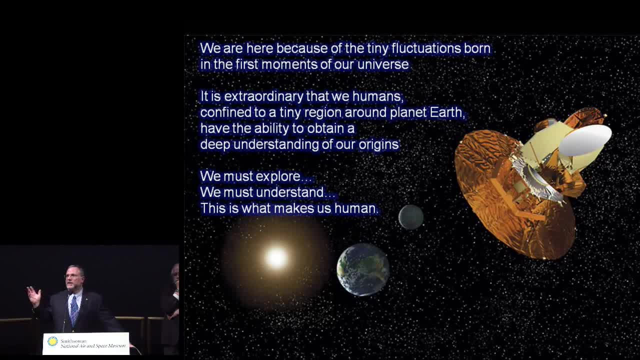 you know, it used to be long ago that electric fields and magnetic fields were thought to be different things and Maxwell discovered that they were related to each other. and then it used to be that the different other forces of nature, the weak force and the electromagnetic force, used to be different and Nobel prizes were given. 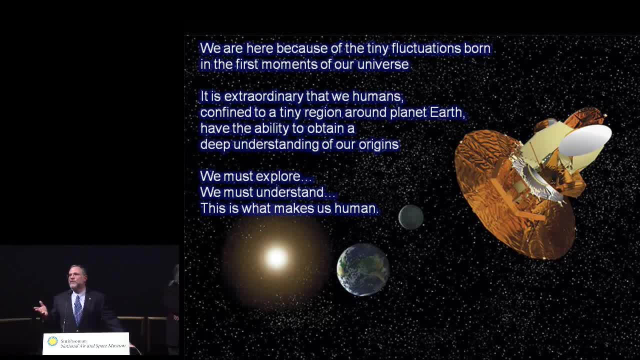 for realizing that those are related. and then it used to be that the strong force was thought to be different than a Nobel prize was given for relating that. the thing that's left out still is gravity. and these new efforts, whether it's string theory, m theory, along all those lines, 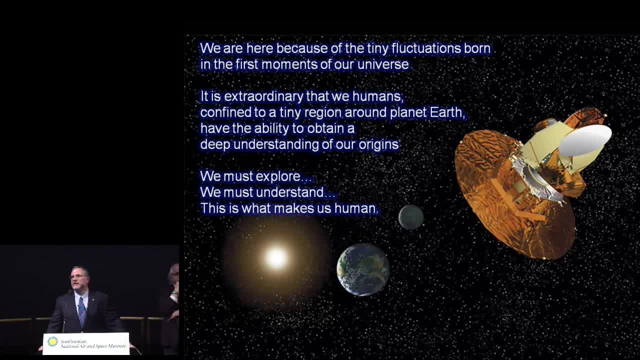 part of the idea is to try to bring gravity into this unified theory and, if and when that's successful, this will be our quantum theory of gravity. there are some people that argue that it's the quantum part that's wrong. what we need is the better quantum mechanics. 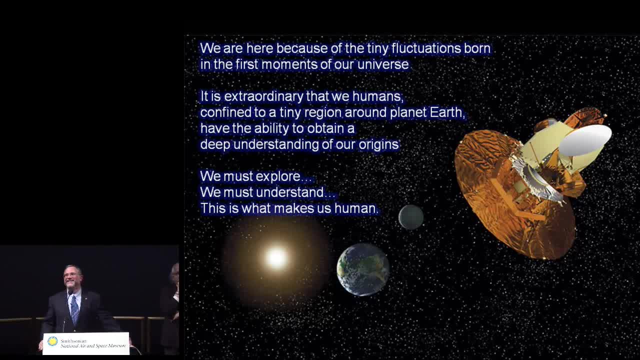 but I think most people think that it's the other way around. just a few more, just one or two more questions, really, because we're running out of time and since I don't see the telescope observer here, it must have a clear sky, so the telescopes are open. 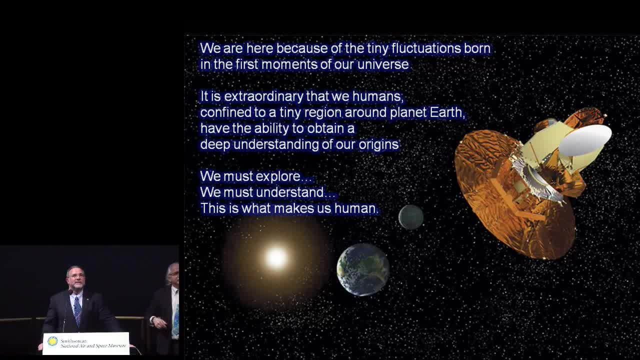 here and then two of them up there, and that'll be it. yeah, okay, let me answer the second question first, because I think I can do that more quickly. so the question is: does the light we get from the sun? 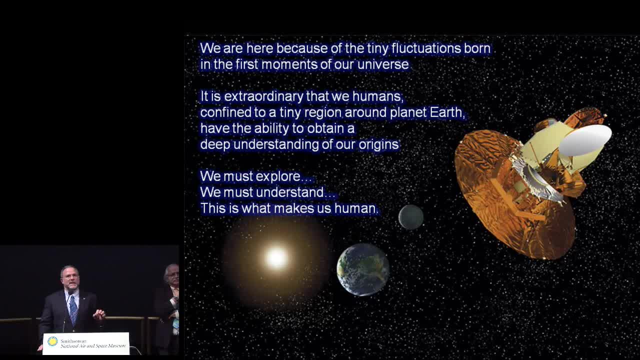 have any relation to the light we get from the early universe, and the basic answer to that is no. the light we get from the sun is from E equal mc squared. the sun converts matter to energy and the energy is the light. so that's because of the nuclear fusion that's going on in the sun. 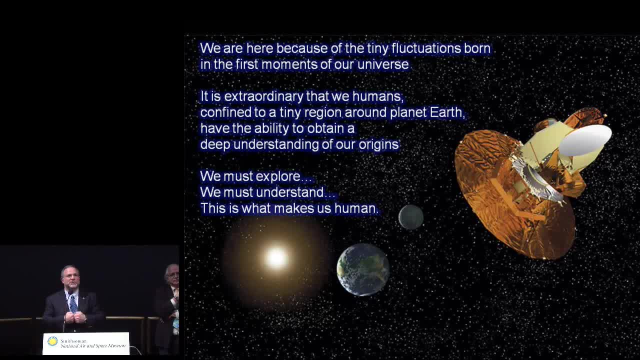 that light is being generated from fusing hydrogen atoms together to helium. 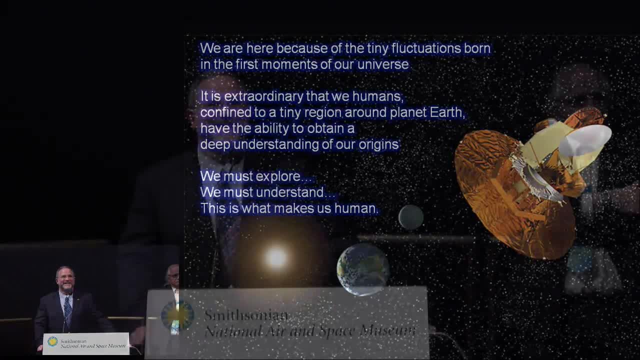 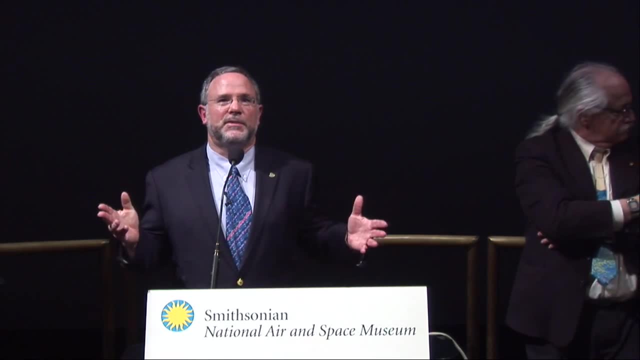 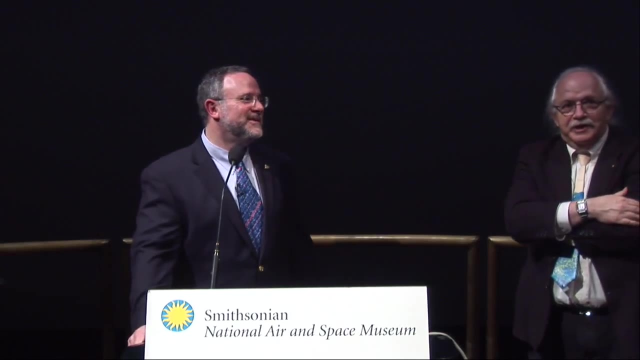 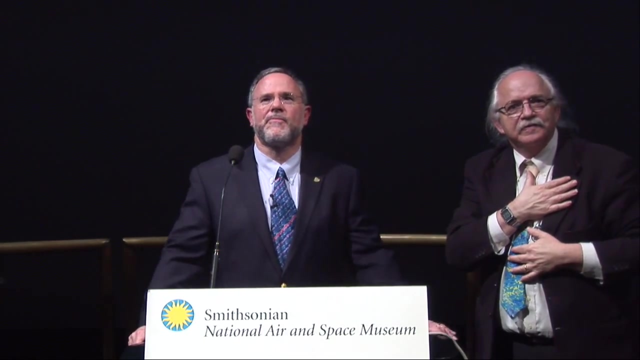 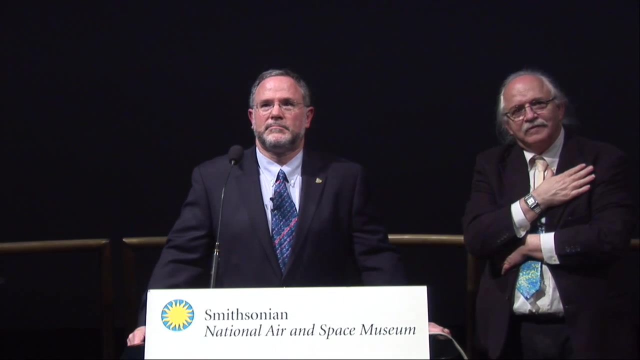 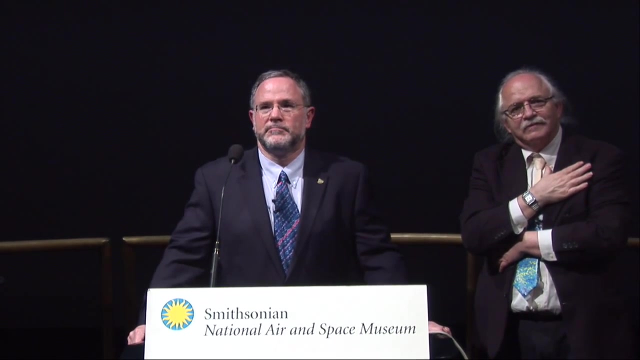 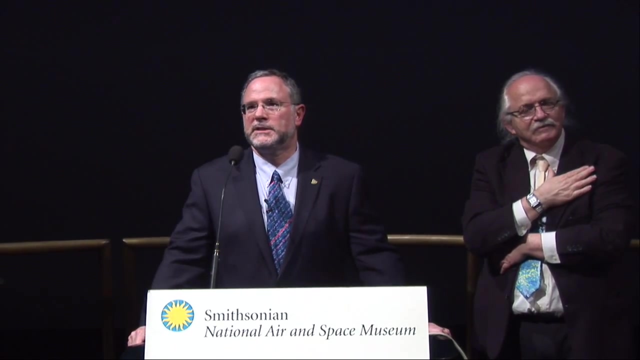 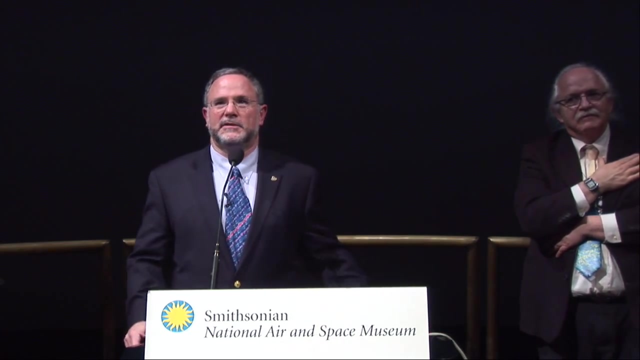 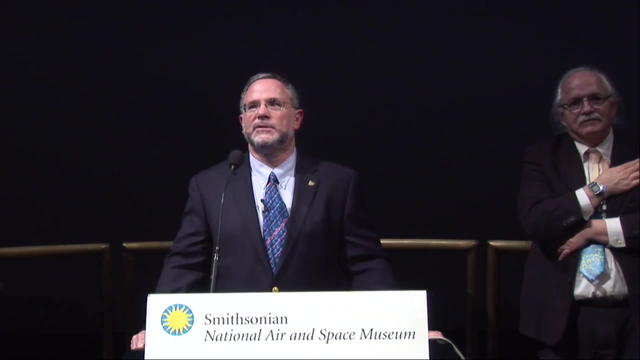 Right. so the question is basically whether dark matter could be the result of multiple dimensions in the basic theories of fundamental physics, And this idea has been around for a while. I don't think it's likely. I'm not saying. 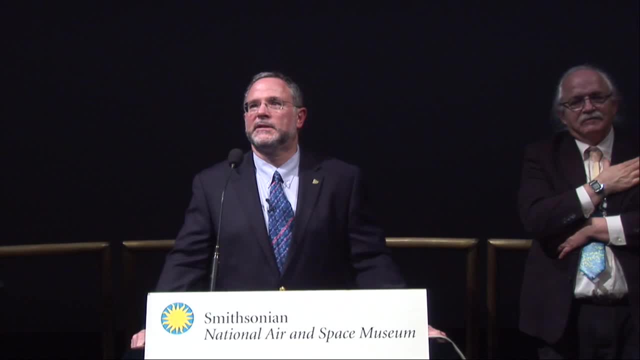 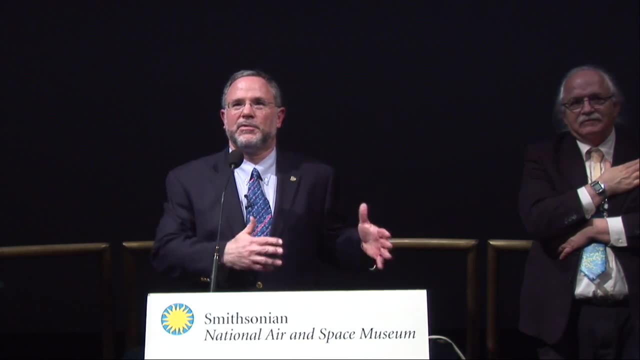 impossible, but I don't think it's likely. I think it's much more likely that there are particles that we just haven't discovered yet, And there's a theory called supersymmetry, that for every particle we have, there's another particle that we don't know about yet. 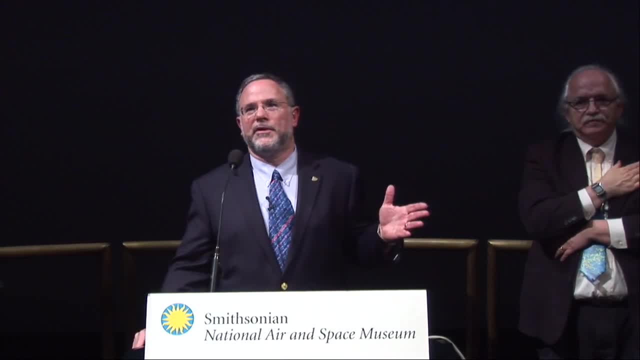 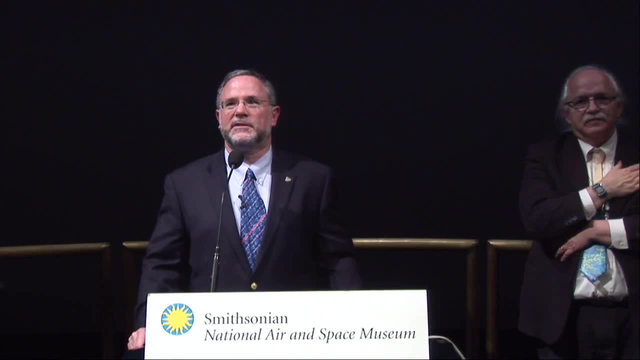 That it's sort of its supersymmetric partner And I think if supersymmetry is right, whatever the lightest, stable supersymmetric partner is is the odds-on favorite for the cold dark matter. And this is why the LHC insert is important, because 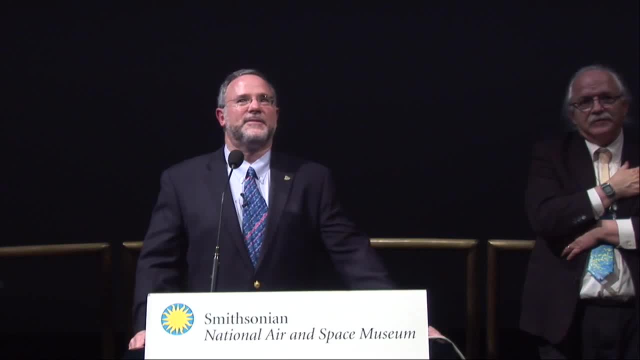 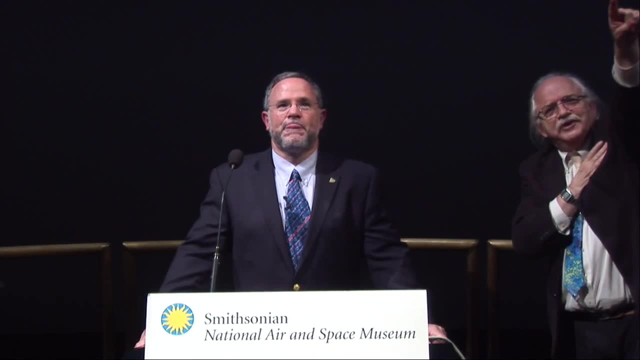 it's going to tell us whether that theory is right or not. I hope. Okay, there's a Yeah. let's just go with the three going up: the Yeah you first, and then in the middle and then on the top. Is there a theory? 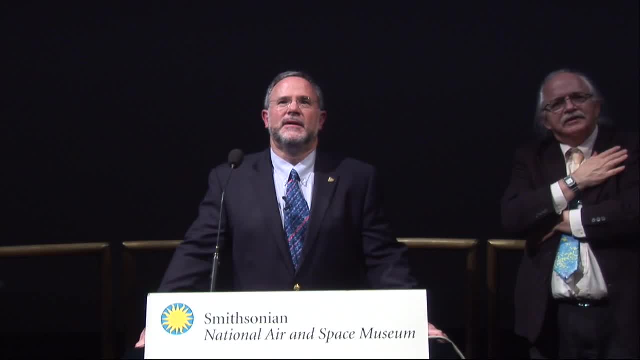 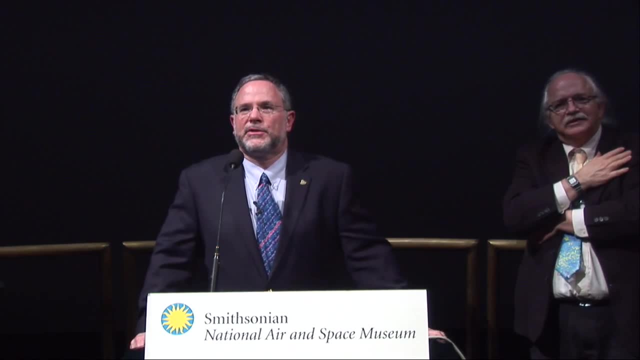 that explains how mass curves space. Well, the question is, is there a theory that explains how mass curves space? And I guess it depends on exactly how you take the word how? but I would say general relativity describes the idea that mass curves space, and in a way that you can. 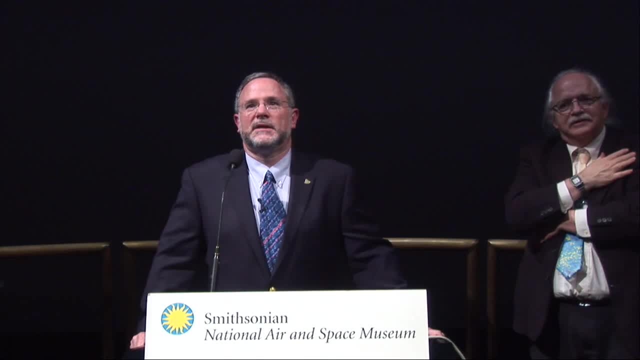 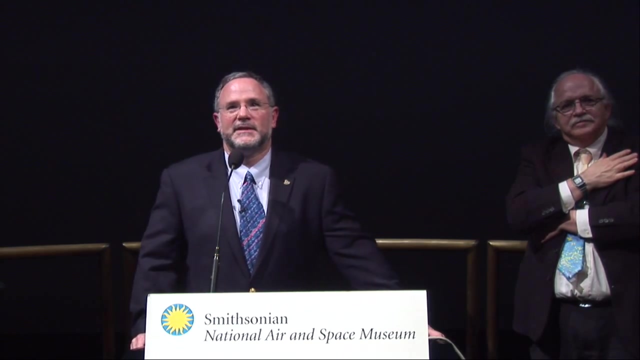 calculate. You know, since I don't know that you could say, this may be somewhat parallel to the situation with Newton saying about how the Earth goes around the Sun, that you can calculate it, but how it does it is another question. So I don't know. 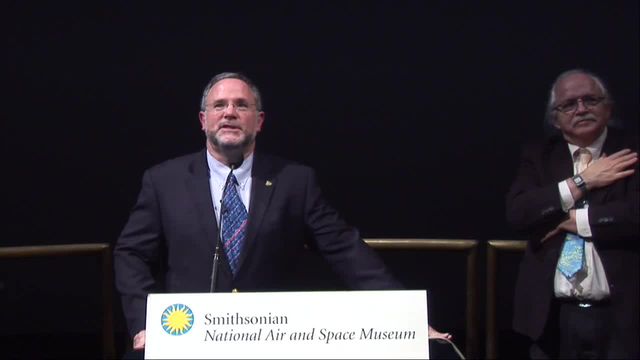 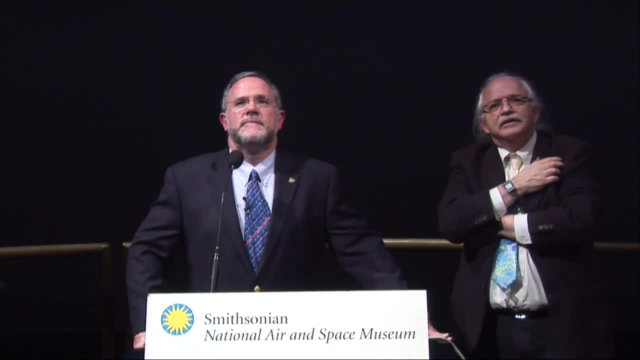 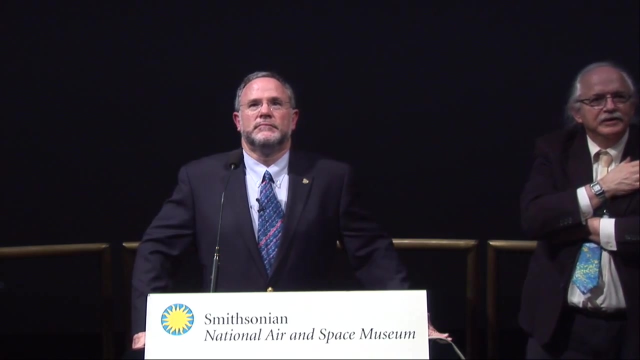 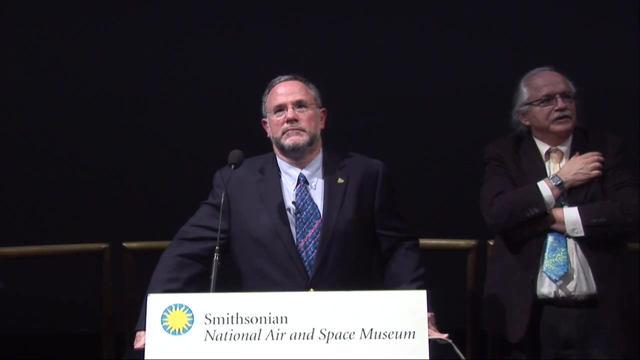 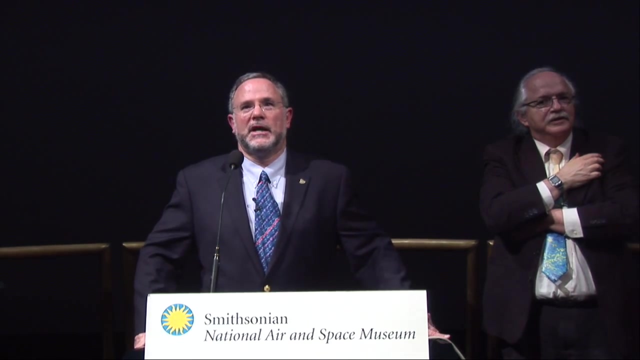 beyond Einstein's equations. any other explanation of that? Okay, with the beard and then up in the back, and that'll be it. The question is: is there a contradiction between the geometry of the universe and the acceleration of the universe? and the answer: 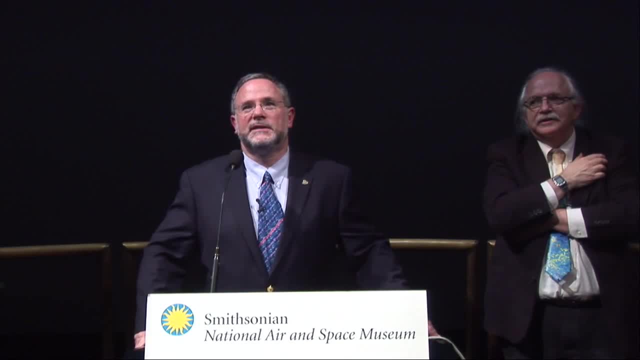 is no. You can accelerate a universe that is flat, Euclidean. you can accelerate one that's spherical. you can accelerate one that has what we call negative curvature, the saddle shape. So all of those can accelerate. There are combinations of things that don't work because they